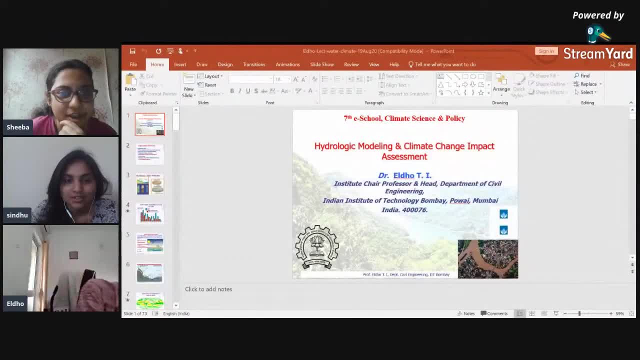 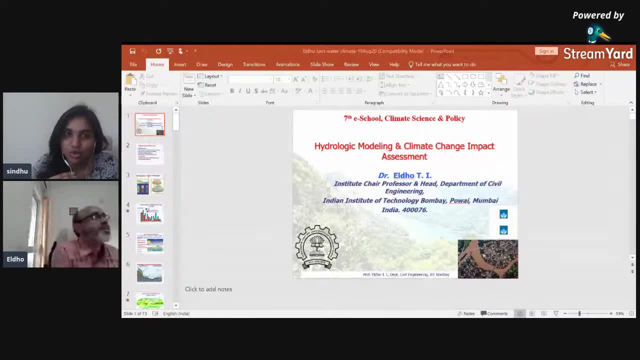 Good evening everyone. I'm Sindhuja and I welcome you to the third session of the 7th year school on climate science and policy. I hope you found yesterday's session on statistical extreme value theory to analyze floods, droughts and heat waves by Professor Arpita Mandal. 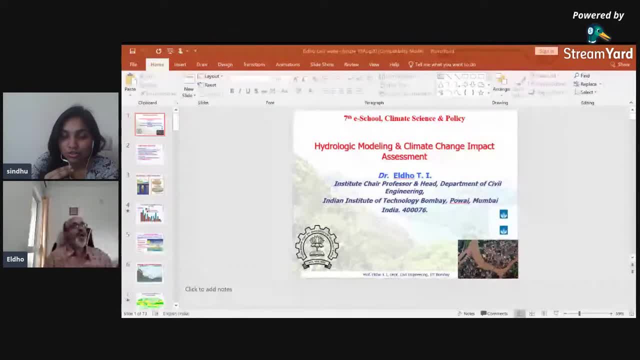 insightful. Those who could not attend the first two sessions can find those videos on YouTube. Joining us today is Professor Eldo. Professor Eldo is an institute chair professor and head of Department of Civil Engineering in IIT Bombay. He has 28 years of experience. 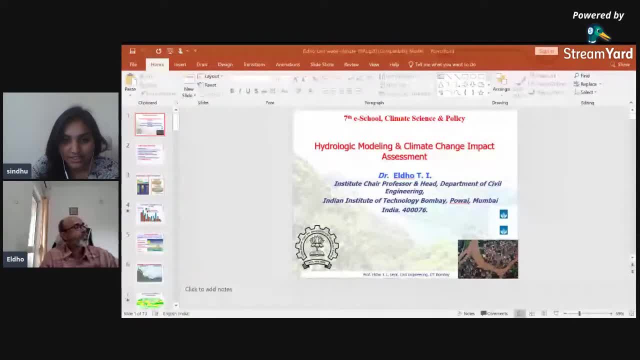 in the area of water resources and environmental engineering. as scientist, professor and consultant, He works in the areas of fluid mechanics, coastal hydrodynamics and climate change, impact on water resources, CFD, water groundwater flow and contaminant transport. He has guided 28 PhDs, 44 postdoctoral fellows and 52 master's thesis, and presently guiding 14 more PhDs. 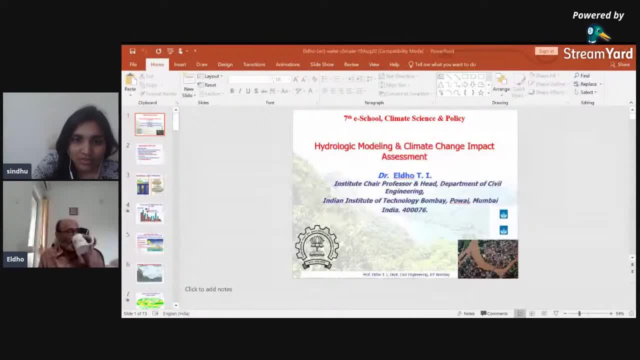 students in various areas. He has published more than 450 research papers in various international journals and conferences. He has developed and offered 25 courses and a number of short term courses for college teachers and working professionals. He has also developed two popular video courses on fluid mechanics and watershed management. Professor Eldo serves as an editor. 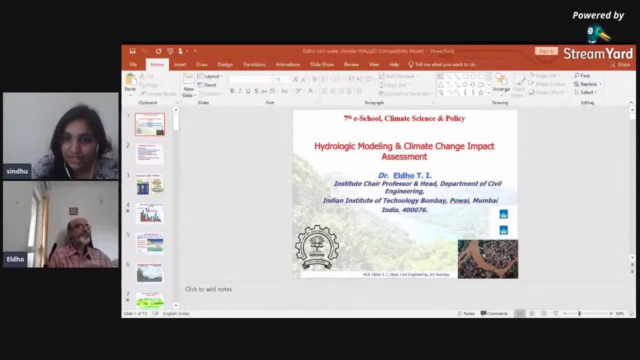 associate editor and editorial board member of a number of Indian and international journals and has been a director for more than 50 national and international journals in the past. in the recent past, He is also a research proposal reviewer for many recent research organizations and delivered several invited keynote lectures at various national and international organizations. 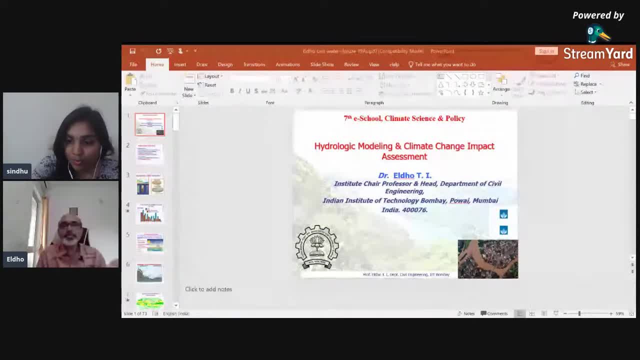 and conferences. Dr Eldo has co-authored two popular note textbooks and contributed 12 book chapters in various edited books. He is recipient of many prestigious awards, including eminent water. He is a professor of the Indian water resource society in 2018.. 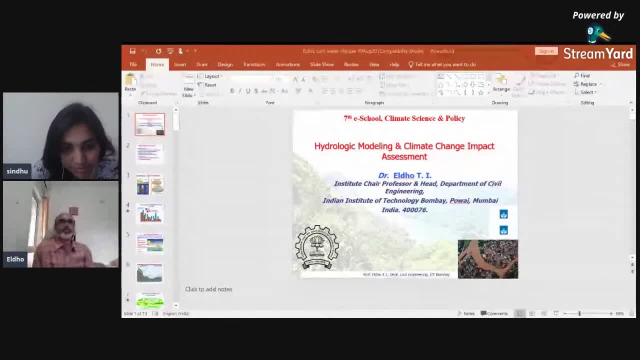 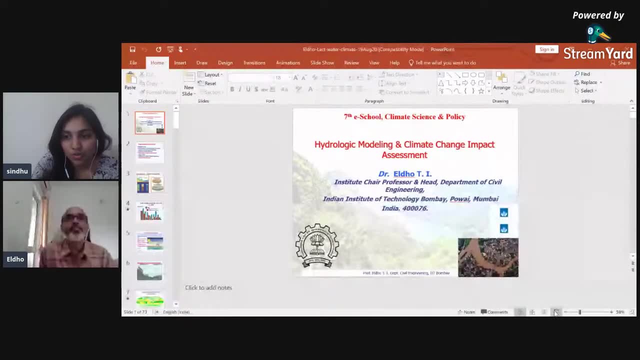 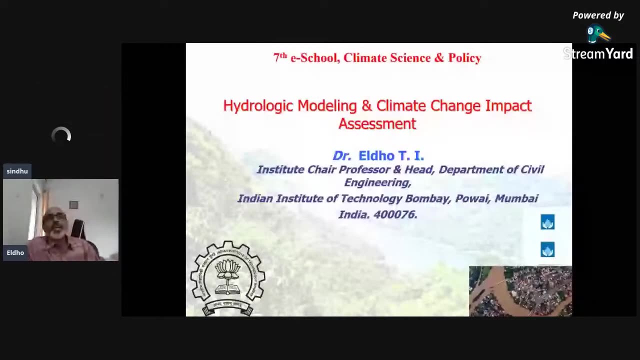 We welcome you, professor, and can you hear me Yeah Over to you, sir? Thank you for joining us. Okay, Okay, sir. Very good afternoon and welcome to this third lecture in the 7th E School of Climate Science and Policy of IIT Bombay, IDP climate. 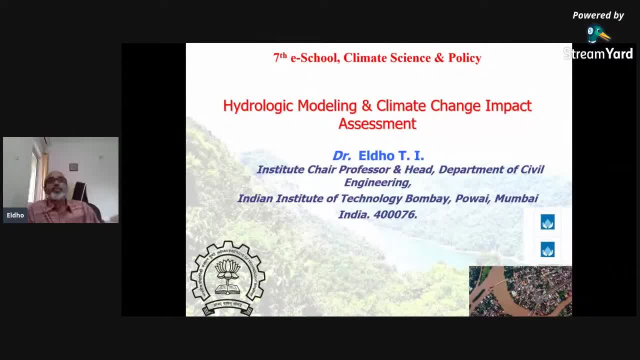 Thank you, Thank you very much, Thank you for having me. So today we are going to discuss- So the already two lectures are over- and then you would have got some idea about various aspects of climate change and its impacts, and then 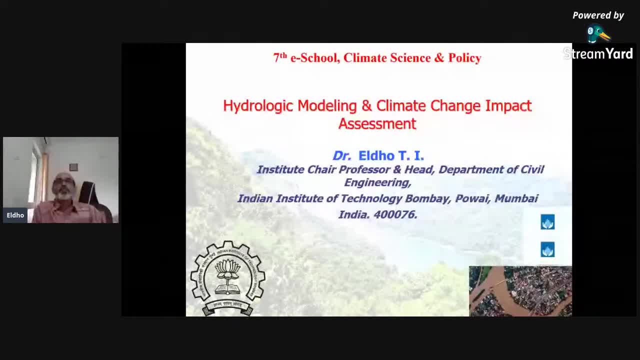 its techniques? what are we are generally using for climate change impact assessment. So today we are discussing, going to discuss in a general way. I am not going to go in a very specific areas, but I am going to give a somewhat general lecture. So, as far as 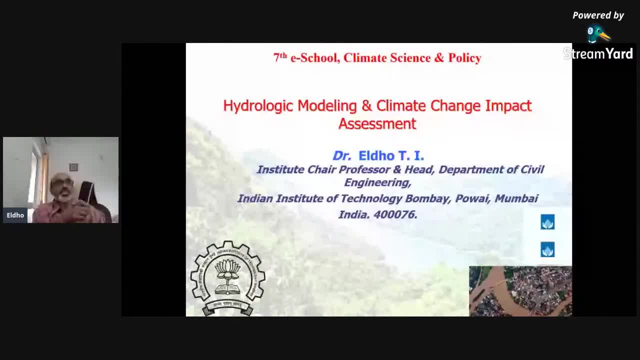 the climate change impact assessment of hydro on hydrology is concerned. So, as all of you know, that climate change, some of the most The the the severe impact, which is already mentioned, is a temperature is rising, carbon dioxide emission, all these things. 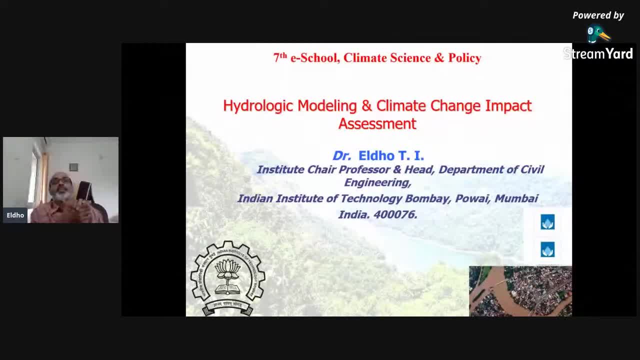 are rising, And then there is a lot of changes taking place to the atmosphere system. So that way, when we look into this, so hydrology, you see that the hydrology and then the climate, and then the climate, and then the climate. these are all important parts of the process. 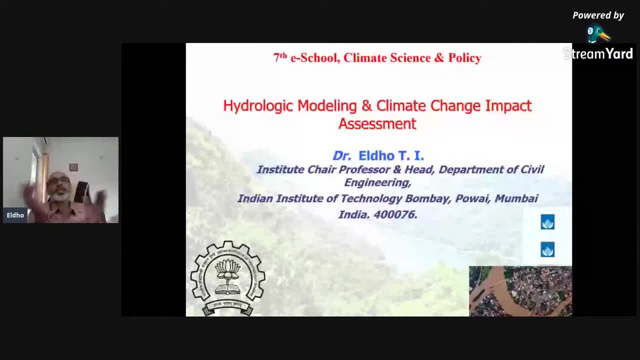 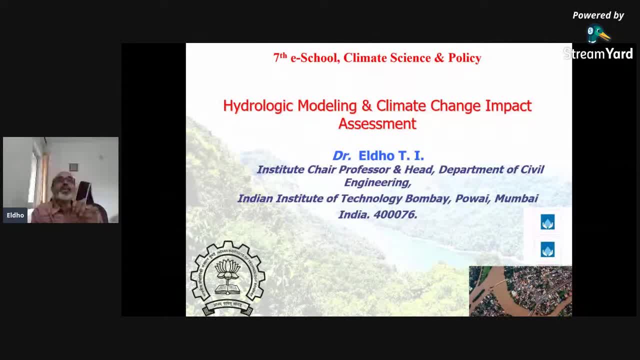 and that is actually as a system, the climate system. hydrology is one of the system which is very much affected, generally should be affected, and then we can see that last few decades so much of impact is there. as far as the hydrological impacts, we can see like 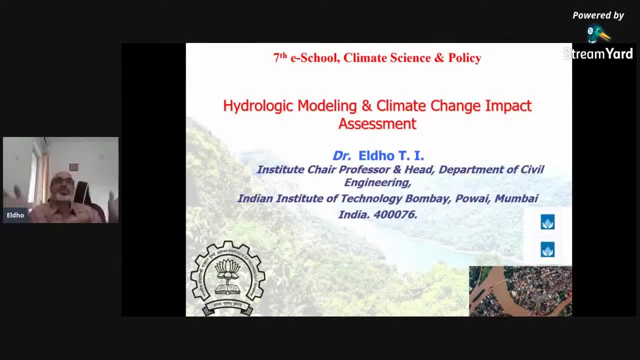 severe rainfall or flooding or droughts. all these kinds of phenomena you can see all over the world And in a country like India you can see. this is very much, since we can see that in India there is only four months of monsoon and then remaining eight months. we have to depend. 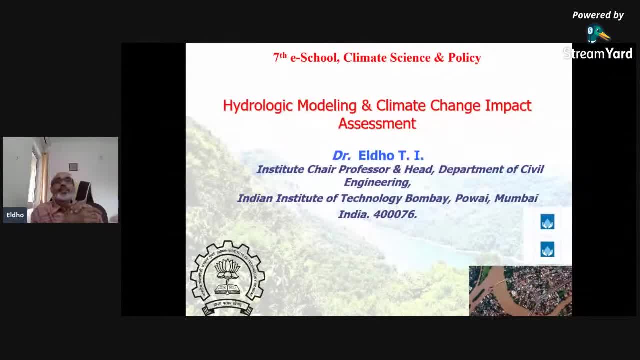 upon the four months of rainfall. So that way, the starting of rainfall, the monsoon, and then how it is going through the country, and then how it is repeating back, all those things are so important. and then it is observed that if you have the 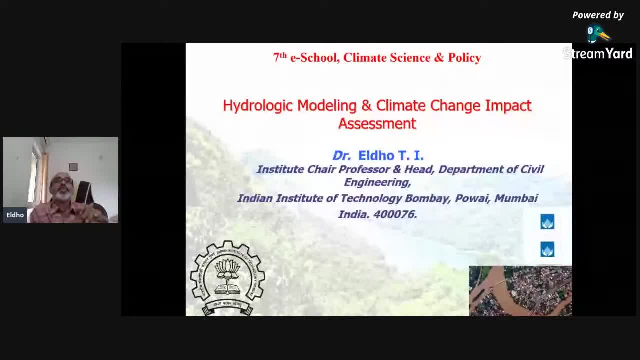 say, the studies then last a few years have shown that a lot of impact is there as far as the hydrology is concerned with respect to the climate change. So within this context we will be discussing the various aspects of hydrological aspects, then how we do the hydrological modelling, and then what are we within the context? 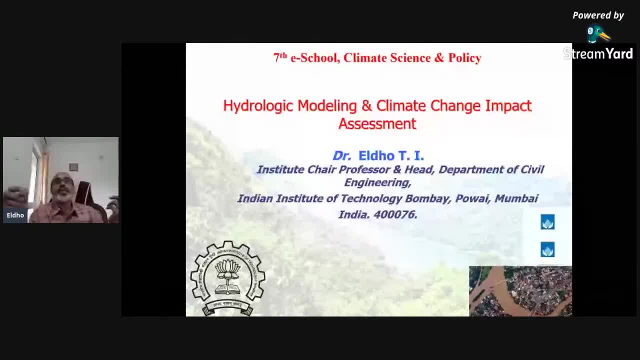 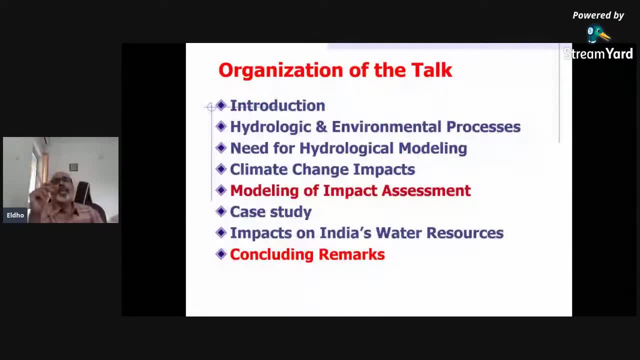 of climate change, So how we can assess in terms of hydrology. that is what we are going to discuss in this lecture for next one hour. So some of the important topics which we will be discussing first one is hydrologic and environmental processes- then say, as you know, that hydrology is concerned, so complex process. 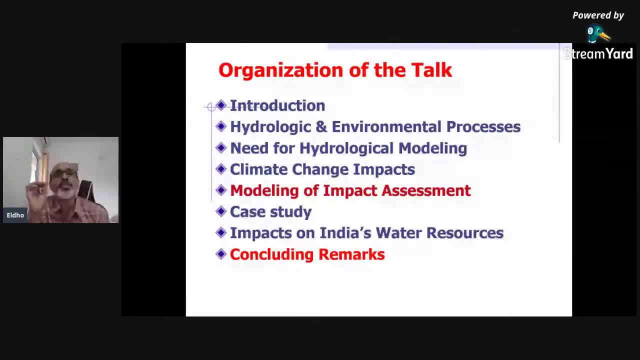 So we need to do so, to understand it properly. we need to go for modelling. So what kind of modelling we can do? hydrological modelling: we will be discussing, and then we will be discussing as far as hydrology is concerned. Okay, 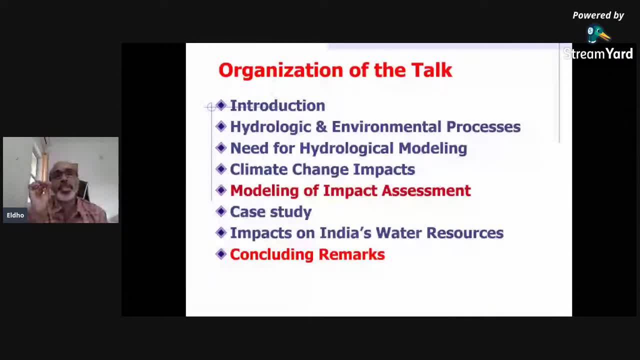 And then what are the climate change impacts and then how we can model these impacts, So that also we will be discussing further. I will be putting one specific case study for a river basin and then also that was done by one of my PhD student, and then we will. 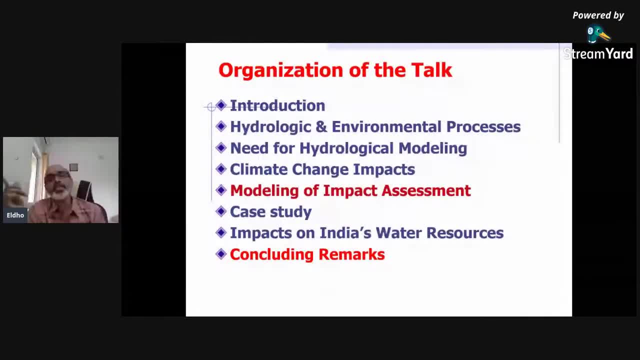 be also discussing for the entire country India, what will be the impacts- So that was taken by from literature- how the variations are taking and then taking place, and then we will be discussing what are the important conclusions and then what is the way forward. 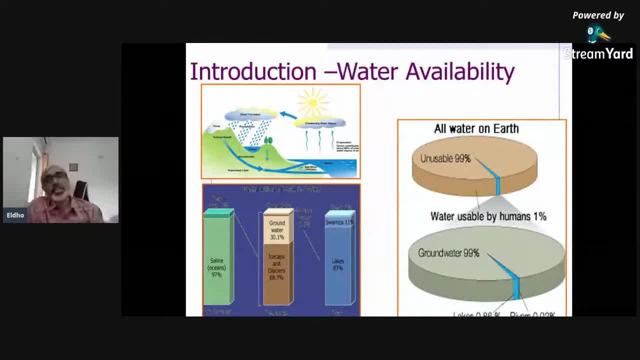 Okay, So, as all of you know that without water we cannot live, or even the earth, the system, the human life or the entire life depends upon water. without water, life is not possible. So that way you can see that what is happening is that everything depends upon this water. 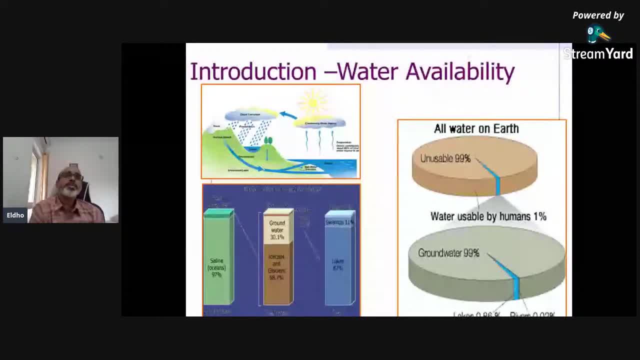 cycle or hydraulic cycle. so you can see here, so that what is happening is that the evaporation takes place and then it is going and then finally coming back as rainfall and then again it is somewhat part of the water will be infiltrating and some part of the water will be evaporated. 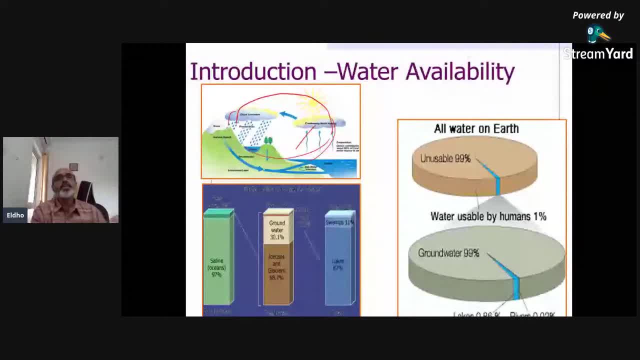 and then again runoff will be formed, and then it will be joining the river and finally it will be reaching the sea. All these cyclic process taking place also. generally we call it a cyclical cycle. So this, though, it is regularly taking place. but if we look into the availability of water, 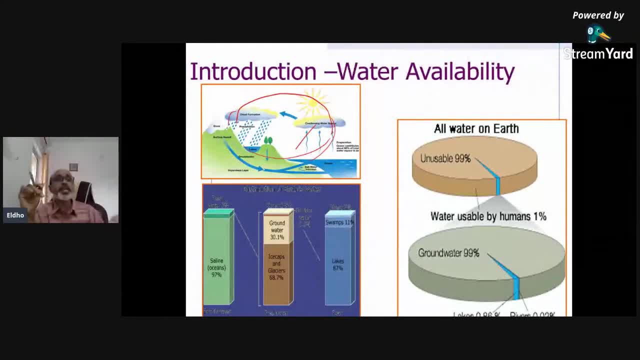 okay, We see that so much of water is available on earth, but almost 97%. we can say that it is saline water and then say hardly out of the available water, the fresh water. say 30.1% is in the groundwater and then 68.7% is in the glaciers and then out of available water. 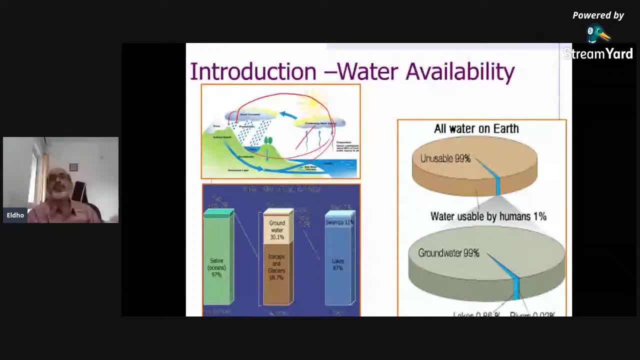 so total fresh water available, hardly one person is utilizable. Okay, So 99% is unutilizable. The reason is that it may be in glaciers, it may be in a very deep groundwater, all those we cannot utilize And then even available this 1% for the 99%, since the deep groundwater is also possible. 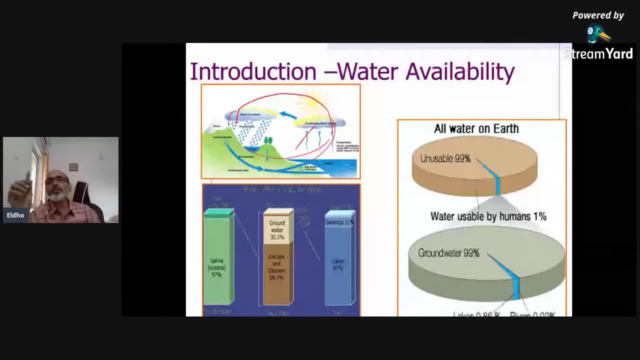 so that most of the water will be in the underground or as groundwater and remaining water is only available in lakes and rivers. So that way, we need to see that. what is happening? So all the what is the so-called climate change, all the impacts that will be mainly affecting 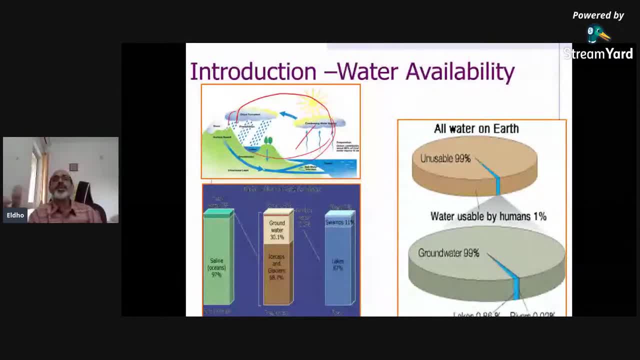 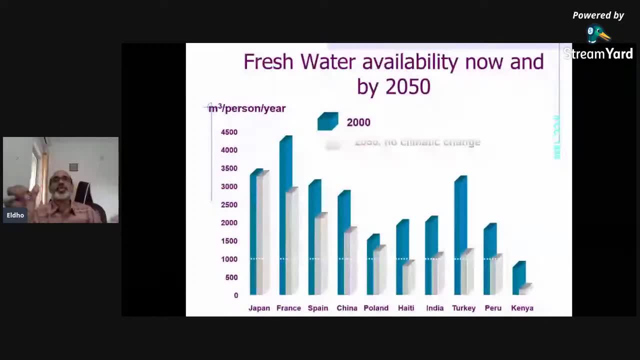 all these available water, either surface water or groundwater. So within this context, we need to see what is happening Now. if you look into some statistics, so these statistics may not be always correct, but this is just an approximation. Say now: fresh water available between now and by 2050. 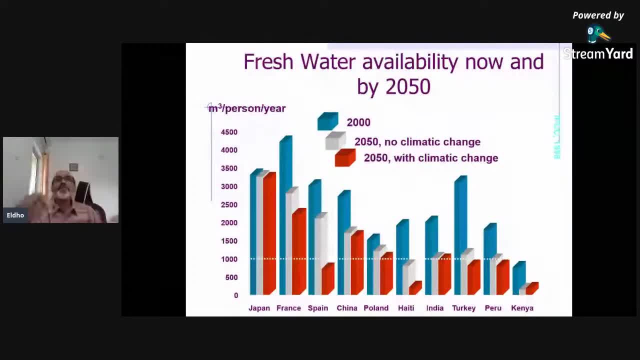 So now 2020, another 30 years. this is only a rough approximation. So, as you can see, that if there is a say, normal, normal conditions, So this, that is what is shown here, And then if there is no climate change, that is only white, this white bar and red bar. 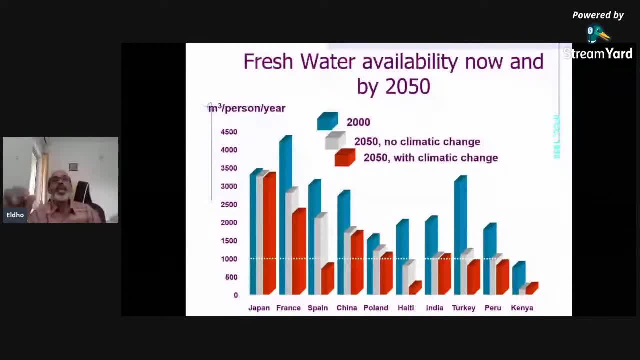 is climate change. So climate change is anyway now very much visible. So then, many countries you can see that the effect of climate change is too much. You can see here, say here, this is too much gap. So here, many places you can see the impact of climate change. 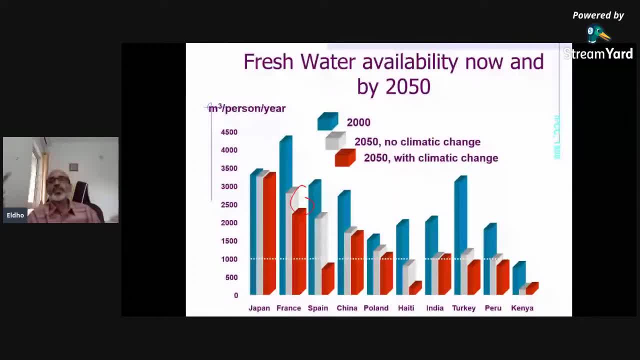 But a country like India, since we are now currently by 2050, our water will. fresh water availability is very, very low And that way that impact is not that much visible, but definitely even a small change, since, whatever you can see, that 1000 meter cube per person per year is. that is what is. 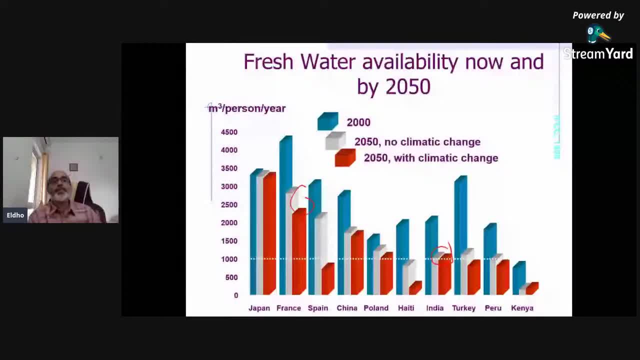 available, And then even there is a small change in space. So if you compare with Japan or if you compare with other developed countries, this availability of water seems to be a population in India. So you can see that this water availability is very, very low. 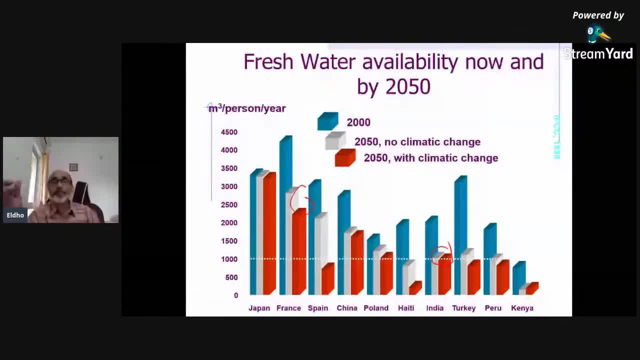 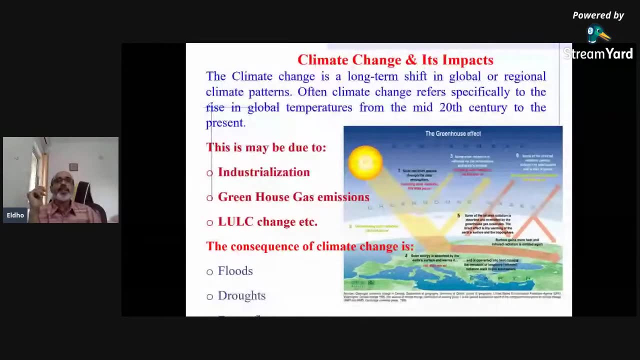 And then in the climate change happens, or the way it is happening, then it will be a major challenge as far as water source management is concerned. So now, when we look into, in terms of hydrology, so, climate change and what are its impacts, 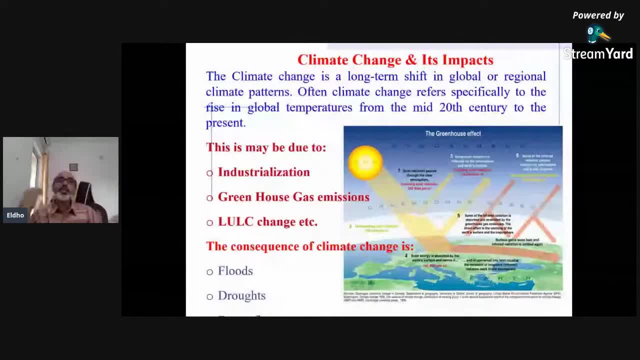 So, as all of you know that I am, I'm sure that many of you have already heard a lot of lectures already studied when your courses related to climate change. So the climate change is a long time shift in global or regional climate pattern. So that way the climate change refers specifically to the, the rising global temperature from 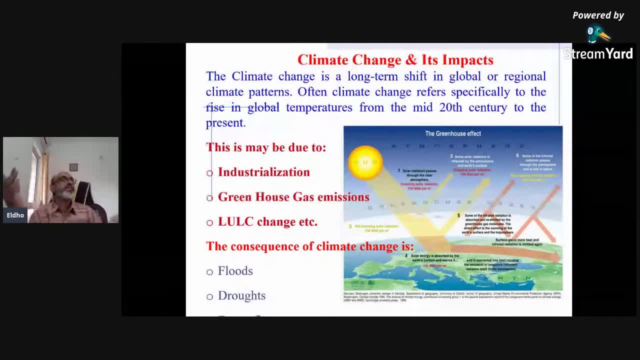 the mid 20th century to the present, And that is, as all of us know, that it can be due to industrialization or greenhouse gas emission or severe changes like urbanization or land use, land core change, etc. 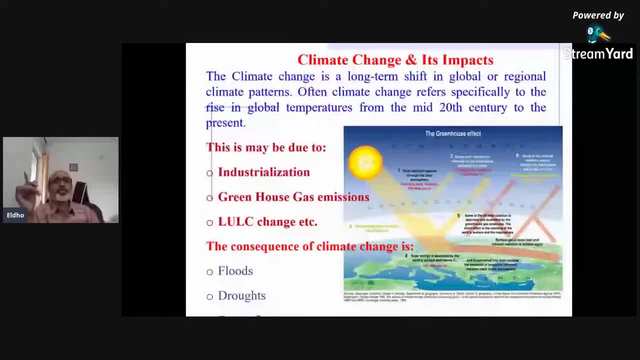 So, as far as the generally as we can observe, what are the issues that we can see the explicitly? there is some number of changes, Okay, So there is a lot of implicit effect to be there and explicit effects. some of these which we can visible throughout the world is, say, floods. you can see that the frequency 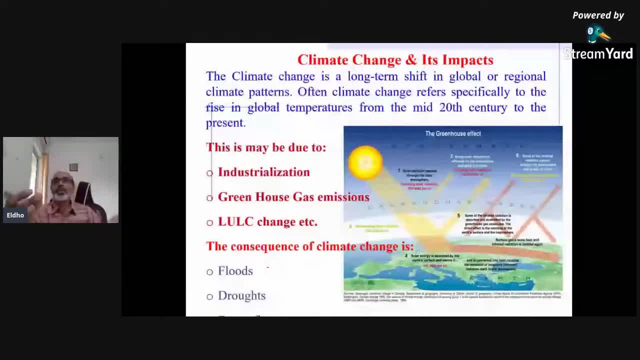 of flood is keep on increasing. So if you consider so, I will show you a table what is happening in India later. But we can see that the the, the number of flooding events is keep on increasing And there will be say: this is year by year, it is keep on increasing. 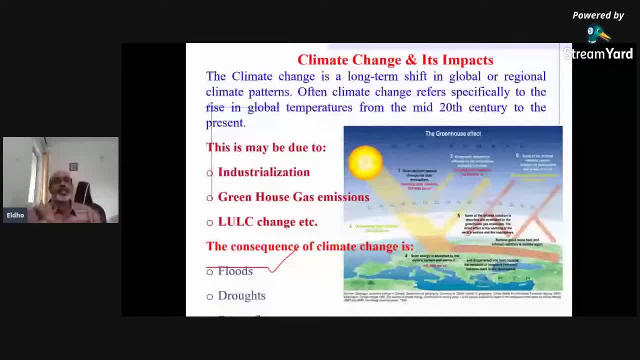 And then also not only the flood events but droughts, Okay, So also you can see that that is also increasing, So that is also very much visible. So then also you can see that last year there was a severe forest fire in Australia and 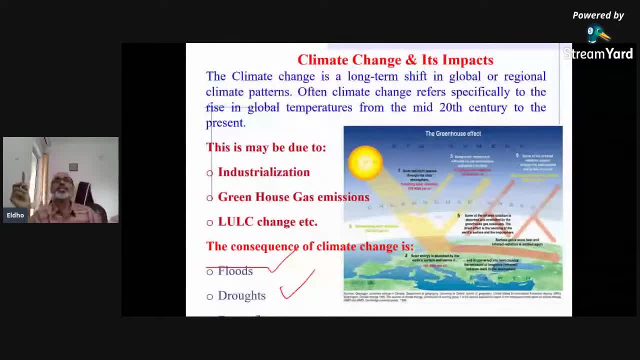 then many countries. so forest fires, all those things effects, you can see. So this is a visible impact as far as the climate change is concerned. So for related to this, we are going to discuss mainly water related issues, So that is mainly floods or the interest to availability of water in the country. 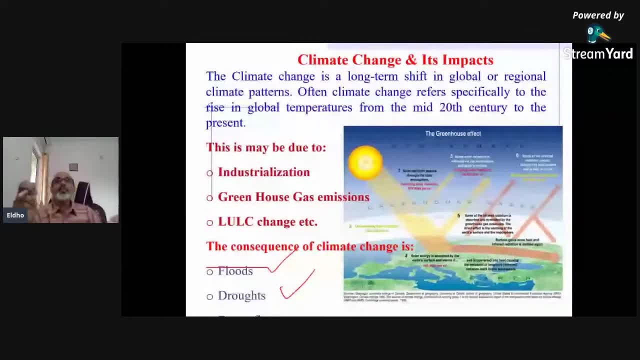 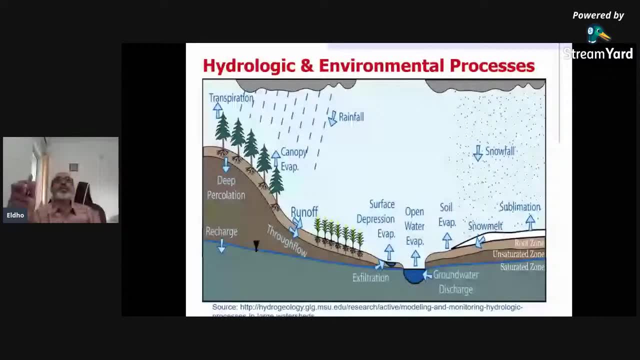 Okay, Okay, So hydrology only we are going to discuss in this lecture. So now, if you look into hydrology as a part of environmental process, so you can see that, as I mentioned, this is all water cycle or hydrology cycle. 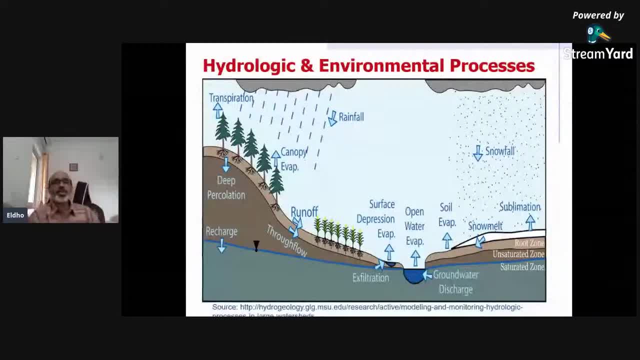 So, with respect to rainfall, then evapotranspiration, all these processes taking place, And then when you consider the reason is that I am showing this slide, is that it is. this is too complex. So this is the complexity is too much, since it is varying from one location to another. 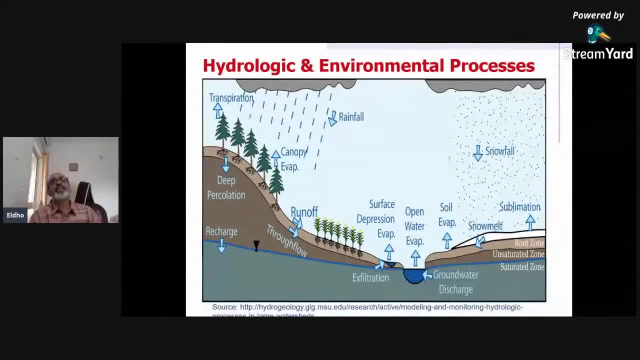 location. The complexity is different, the changes are different and since when the topography changes, when the land use, land cover changes, when all the other system changes, then you can see there will be a lot of difficulties. So to quantify, to say that what is going to happen, or to predict, or to even project, 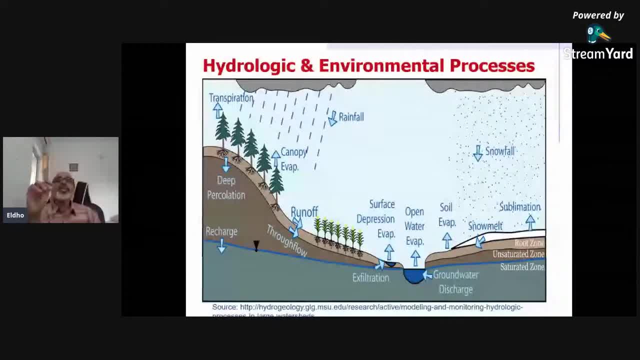 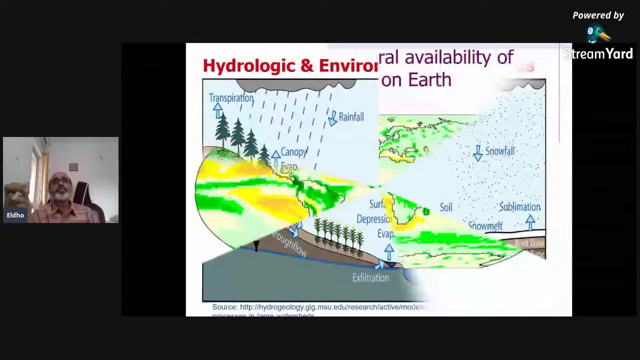 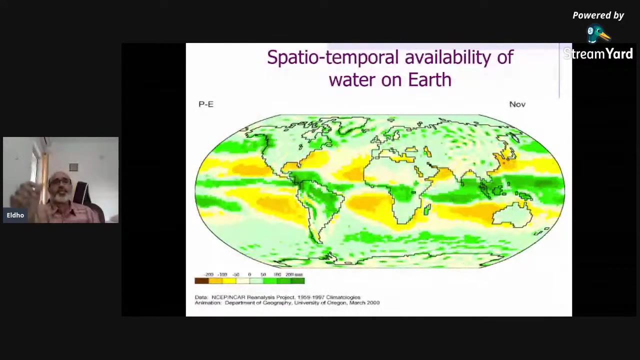 that is, a lot of difficulties, will be there. So that way, Gupta of space applicants at Ahmedabad, you can see that this is a major challenge as far as 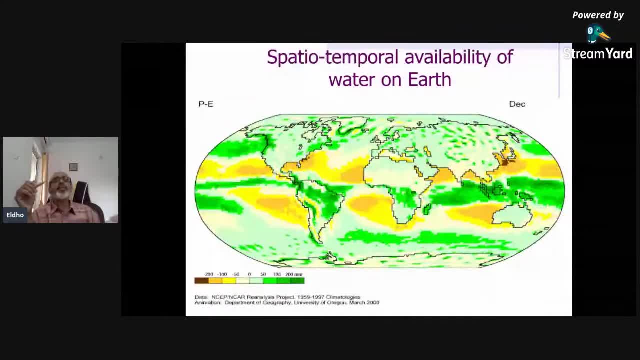 most of the countries are concerned, as in India. So the water availability is keep on varying with respect to space and time. So you can see that in India the monsoon is, as I already mentioned, only starting from June to October the monsoon season happens, and then only the rain is available. 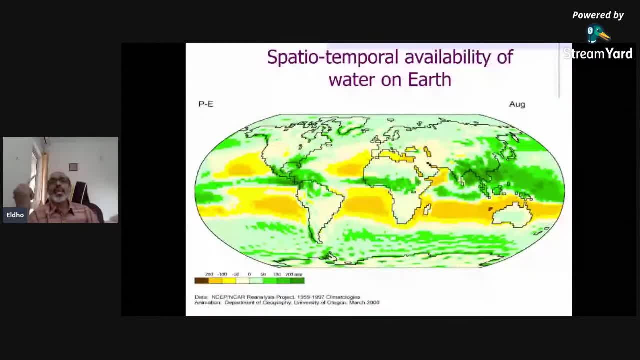 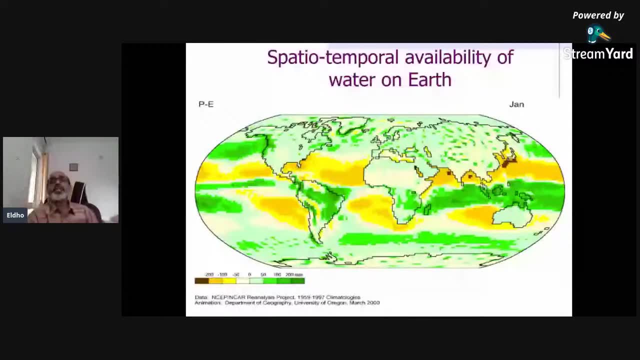 Otherwise the remaining- say, 7 to 8 months there is no rainfall and then we don't have that much water. And then space-wise, if you look into, you can see that some parts of Western Ghats or Northeast we have got almost 3,000 millimetres per year, or even some places more than 5,000. 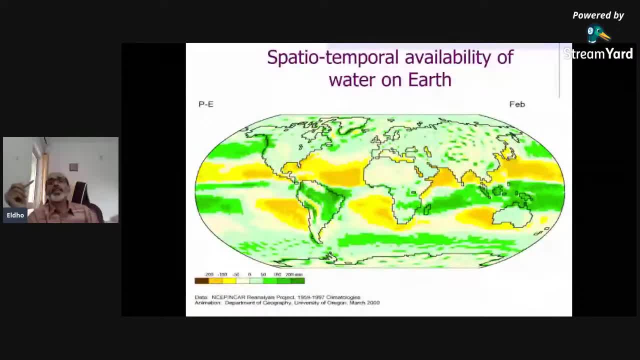 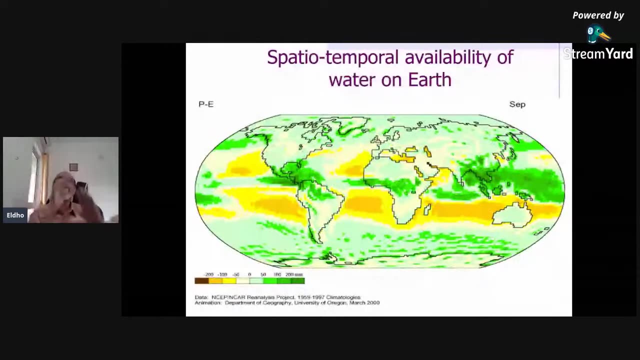 millimetres per year, But in places like some region, like Gujarat, Kutch or the Rajasthan region, we are hardly less than 10% of that. Even say, some places even 20 centimetres or just less than that. So that is the main issue. So space-wise also, there is huge variation, and then temporal. 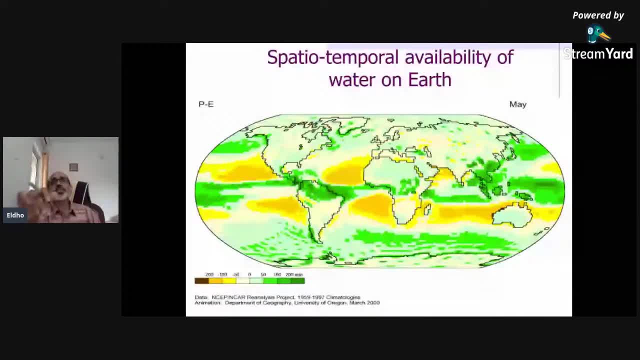 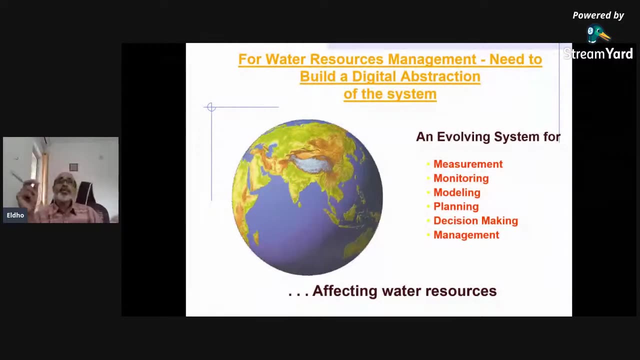 variation. So that is why the water resource assessment, the water resource planning and management becomes so challenging. And now we are having this, climate change means, that is, the challenges further increasing and then we need to deal so many aspects. So that way, when we 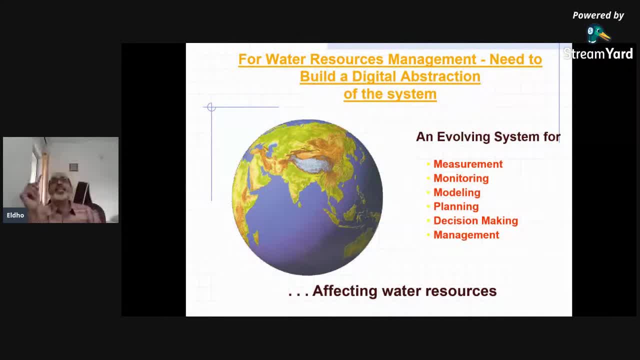 look into water resource management, we need to build a digital abstraction of the system. So that is why say, for example, if you consider a country like India or a particular river basin, so we need to evolve a system for various aspects like measurement, monitoring, modelling. 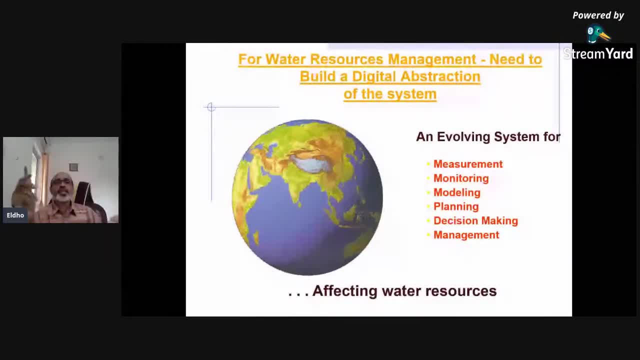 planning, decision-making, management, etc. So that is very much essential. So that way, modelling is very, very essential. Hydrological modelling is essential to understand what is happening and, with respect to climate change, how we need to go for the planning. So that is. 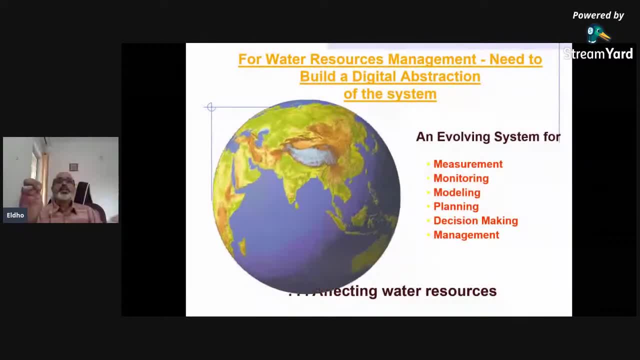 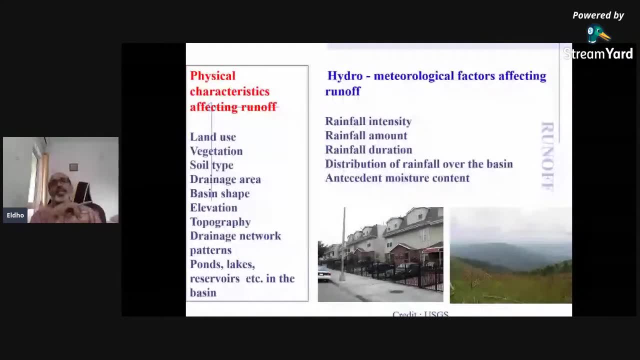 very, very important. So now further, if you look into, say we need to see that whenever we say in terms of hydrology, the climate change impacts, So we have to see the hydrometeorological various factors. So first one is the physical characteristics affecting the runoff. So when we 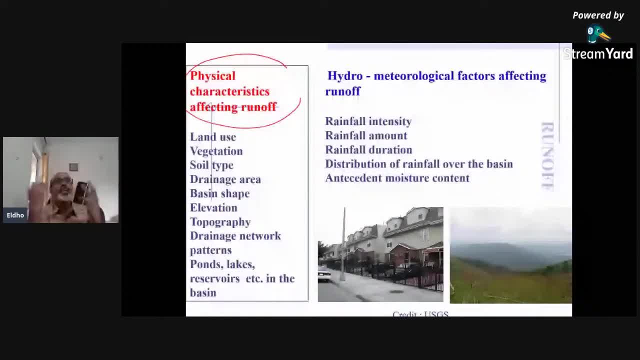 consider, say, a particular river basin, we need to see the hydrometeorological factors affecting the runoff. So when we consider a particular river basin, a particular watershed, of course the country-wise or state-wise also we can consider, But say as a scientific unit. 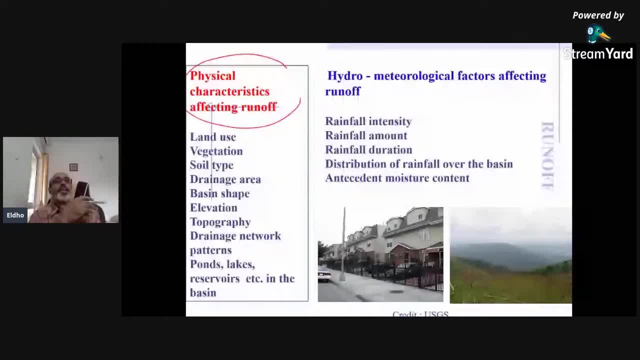 we generally consider as a river basin or a watershed. So that way we need to see various aspects. So most of the aspects I have listed here, like land use, vegetation, soil type, drainage area, basin shape, vegetation, topography, all these aspects we need to consider. 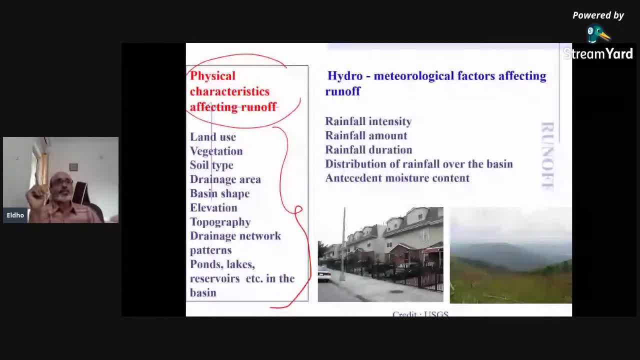 in totality, so that we get a better assessment. So that is as far as the physical characteristics of the watershed or the river basin, And then the hydrology. what is happening with respect to the hydrology system, hydraulic system So, or hydrometeorological factors like what is the intensity of rainfall? 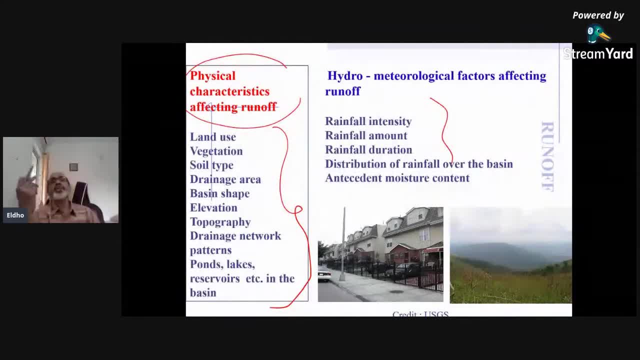 So if they say the intensity is increasing and short duration rainfall, that is always causing the floods, And then we need to assess how much is the rainfall amount and how much is the duration. So all these things are very, very important. So most of the studies conducted so far show that. 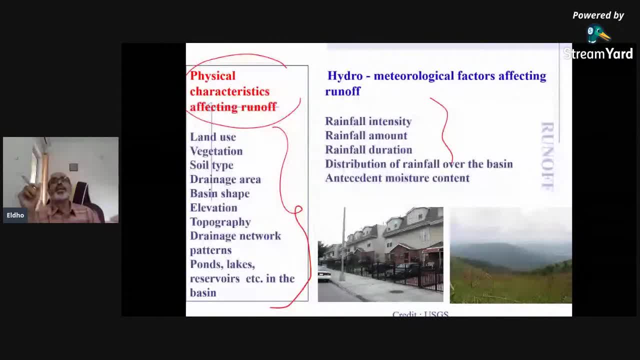 though many places the total rainfall may increase, the total available water may increase, but this rainfall is going to happen in few events, So that high, intense rainfall happens. short duration rainfall will happen. So that way, what we can see is that there can be severe 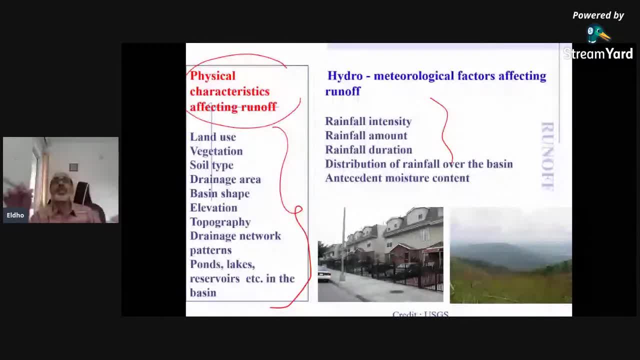 problems of flooding, So number of events decreases. the rainfall even decreases. means then we can have afterwards there is water, So number of events, water scarcity or drought type of conditions can take place. So that way we need to take in the physical characteristics of the watershed or the river basin. 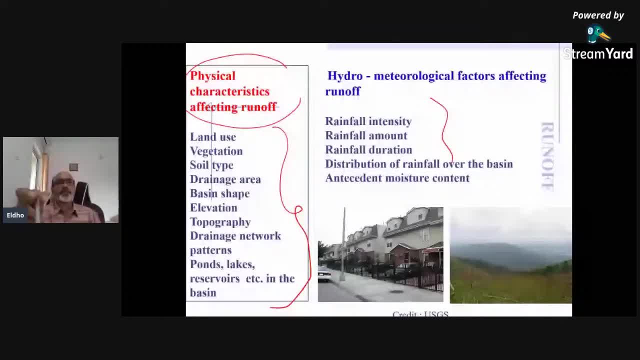 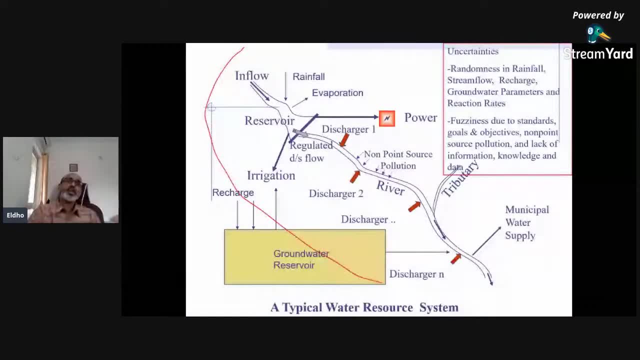 And then also we need to see the hydrometeorological factors as listed here. So now, if you consider, say, for example, now this is a watershed or a river basin, So here we are having the river basin, So this is the major river passing, And then you see that at various locations. 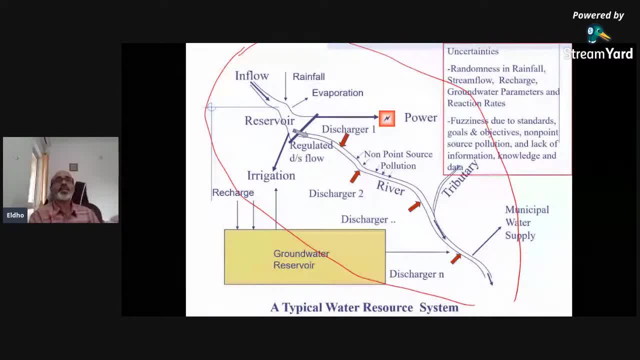 and we are having the discharge, then we are taking the water. so various recharge, various system is there. so this is just like a watershed or just like a river basin. so there we need to consider in a holistic way: so what kind of? of course the input is rainfall only, mainly, most. 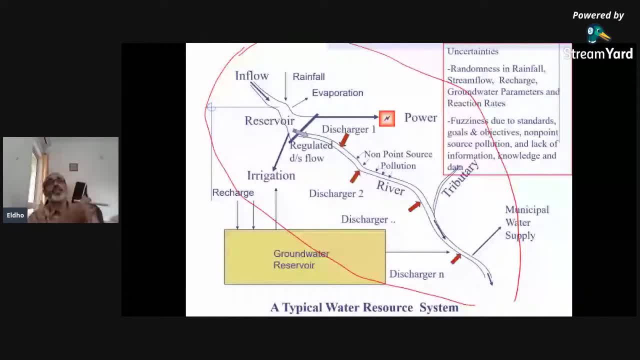 of the time, rainfall or otherwise, some inflow coming from other watersheds or the other side of the river, and then the, the, the usage or the, the, the way which we are using the water is. it can be so, of course, evaporation, then infiltration, all those things place and then 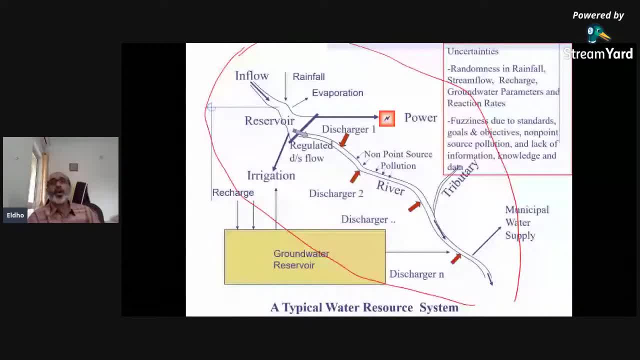 water is taken for power production, water is used for various purposes. all those things happen. so a typical water source system. we need to see that. so here, this is the, the outlet. so we want to say, if you are going to construct here a dam, so like this, we need to see that, how much water is we? we are 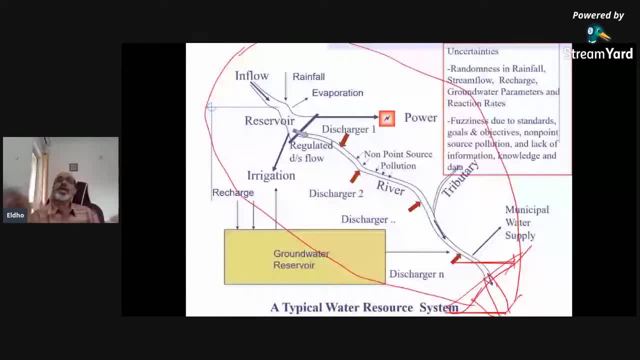 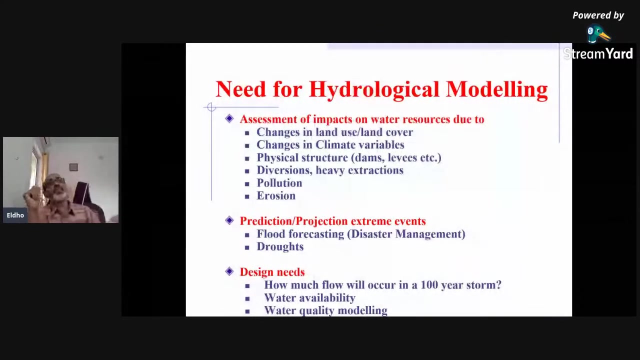 able to store and what way the system will be affected. so that way, when we look into, there are so many uncertainties, so- and this means can be rainfall uncertainty, stream flows, recharge, groundwater parameters, so so many uncertainties are involved in all these kinds of systems. so that way, as i mentioned, if you take a river basin or a or a watershed, we need to model it. 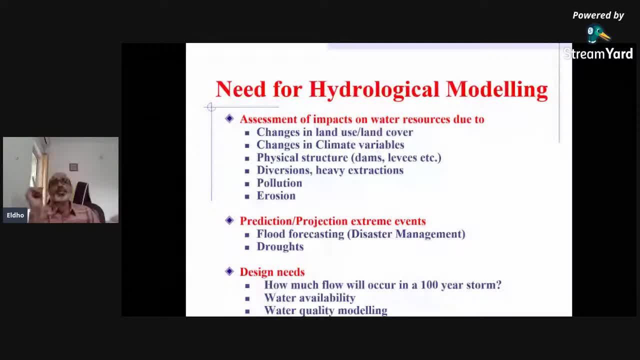 properly, so that the hydrological modeling is so important. so hydrological model, why you need a hydrological model, so here. i have put so many aspects here. so this is uh hydrological modeling for assessment of impacts on water source due to so change is in land use, land cover, as i mentioned. 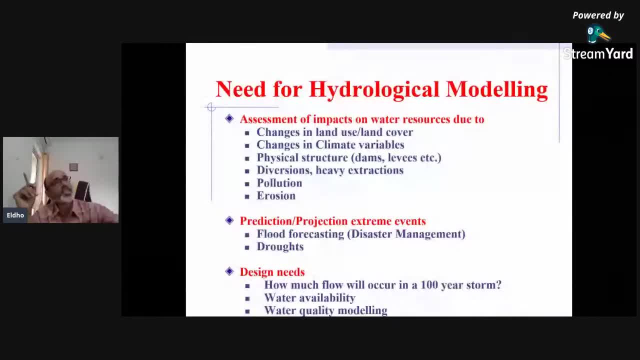 if you take the last few decades, there is a drastic changes has taken place with respect to the land use, land cover change, especially urbanization and destruction of forest. and then you have to see that the the impacts due to the climate variables, so the climate changes i mean. 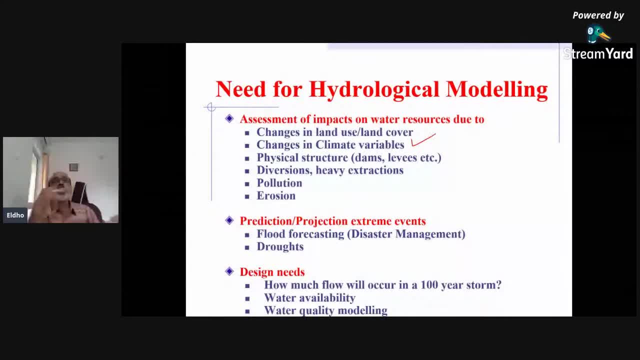 is in temperature, or all the parameters we need to consider. and then what is happening? so we have constructed, last few decades, so many dams, so many the, the systems, reservoirs, all are constructed. so what is its impact? and then diversion, heavy extraction, all these aspects, including the 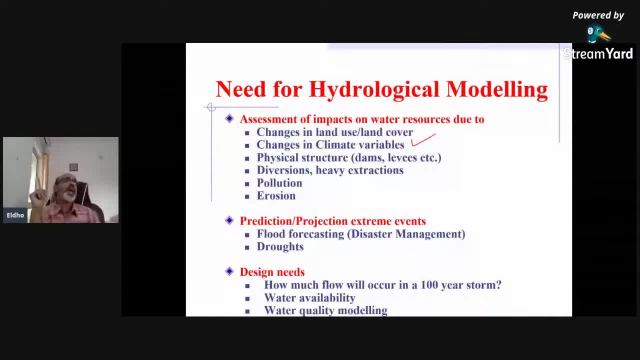 environmental pollution- that is also very important- pollution and erosion we need to consider while looking for in a hydraulic system, in a river basin scale or or in a watershed scale, and then when we look into protection, prediction or projection. so, as i mentioned, in hydrology one aspect is the 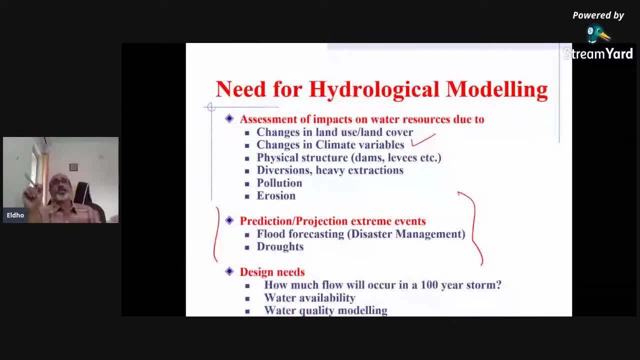 extreme, so that is spread. and second one is ground, so flood forecasting. so for disaster management, we need to say at least a few days in advance, especially cyclones or all these things, what is the possibility of flooding. we need to tell you a few days in advance so that what can? 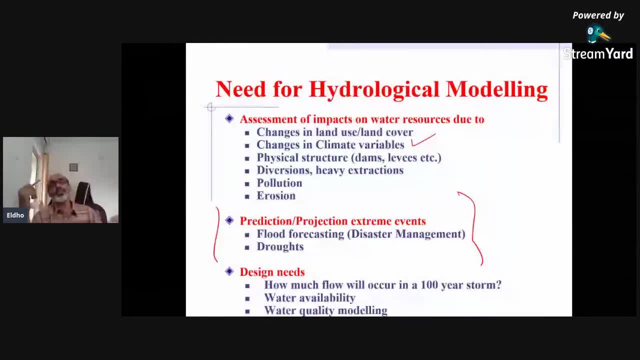 happen, we need to do some mitigation measures, we need to go for a disaster management. so that way forecasting is very, very important. and then droughts also. if you can say that what is going to happen, maybe in we can predict here in some time, some few months or a few weeks in advance. 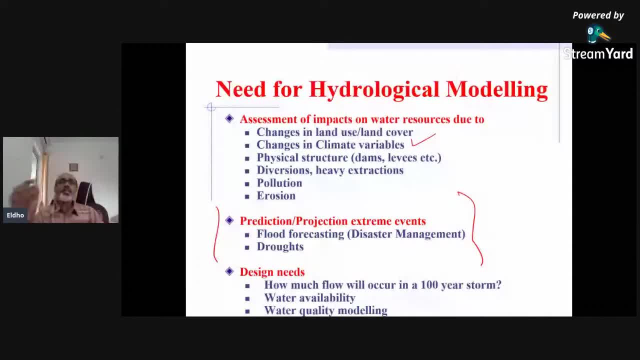 so many mitigation measures are posting. so that way, when we look into in these kinds of modeling we need how much flow will occur in, say, for example, in a long time, like 100 years, and then how much water is available. and then of course it is not only available, the quality of the water is also. 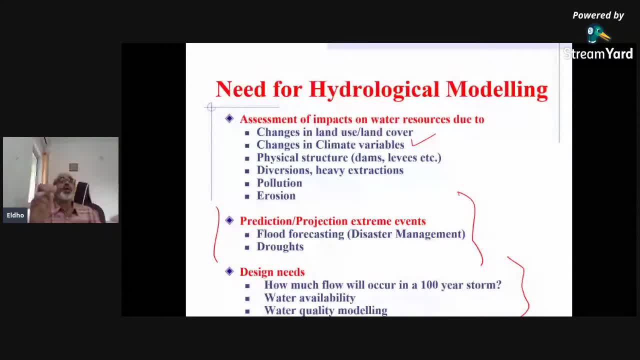 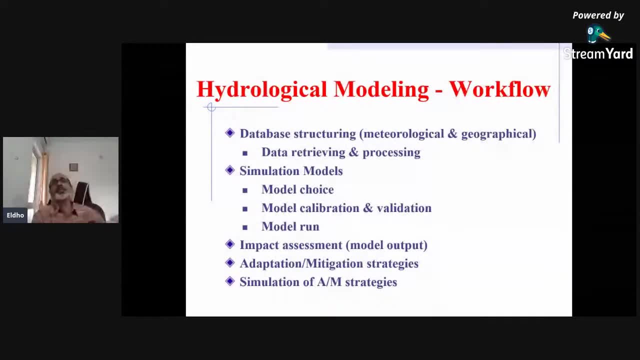 very important. so that way, when we look for hydrological modeling, all these aspects we need to look into. so now, as i mentioned, there is physical features of the watershed or river basin, and then we have got a meteorological or the the hydrological aspects. so that way we need a. 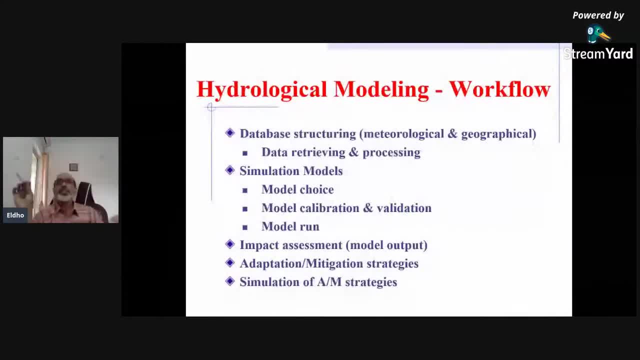 database, by considering all these things so that we can see that what is happening. so next 30 years, 60 years or 100 years, what way it is happening that all those things we can do and for all these we can have the simulation models, hydrologic simulation models, so hydraulic simulation. 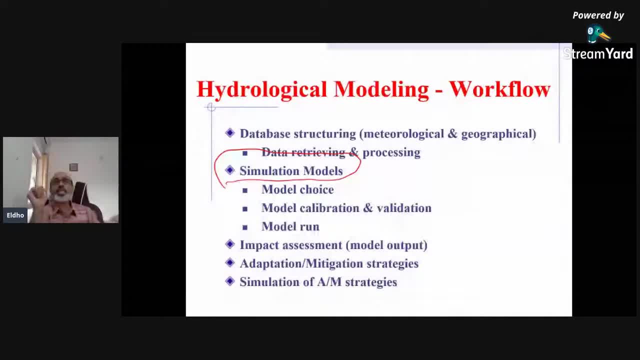 models like we are. we will be discussing one of the model like a swat here. so these, these models. so there is plenty of models. so last few decades, a large number of models are developed. some of the models are freeware which we can download directly and then use it. some of the models we have to pay. 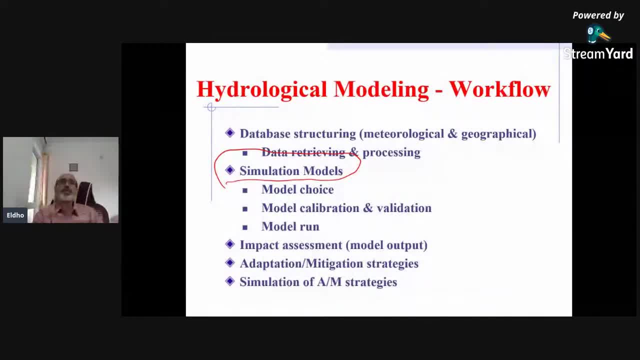 and use it. so some of the important aspects which, when we the models, especially to assess the the climate changing fact, we need to see what kind of model we are going to choose. so model choice is very important, whether we need to have a go for a lambert model, distributed model or black box. 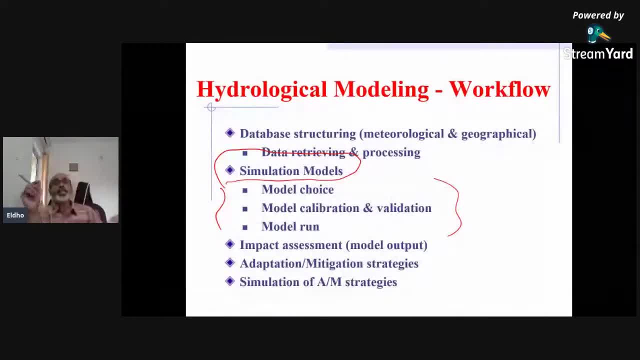 model, variety of models are available, and then how much calibration and validations we do, since, in hydrology is concerned especially, i have seen shown that what are the important aspects we need to consider? so that way we need to look into the various parameters which are influencing the hydrological uh. 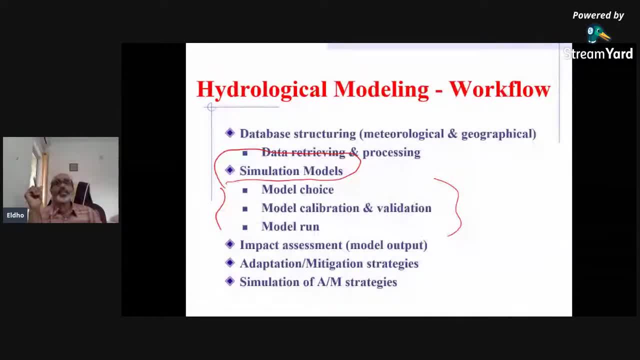 uh phones. so that way we need to go for calibration and then validation. so we need a data for that and then, once the calibration, model, validation is done, we can go for a model run and then, using that model run, we can go for impact assessment. so like climate change impact or the land use. 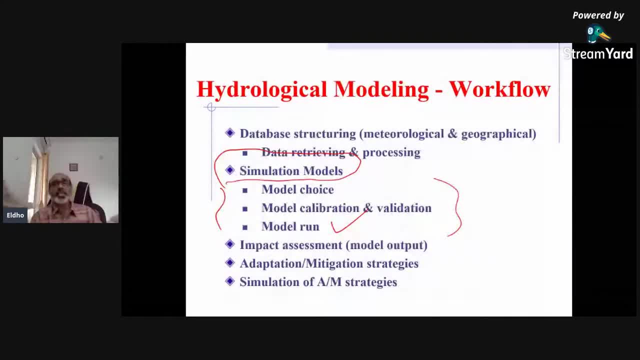 length or impact for the next 100 years or 80 years or near time, near time or middle time or long time impact assessments we can do and then, once we know that, yes, this is what is going to happen, then we can go for adaptation and mitigation strategies. so that way, all these adaptation, 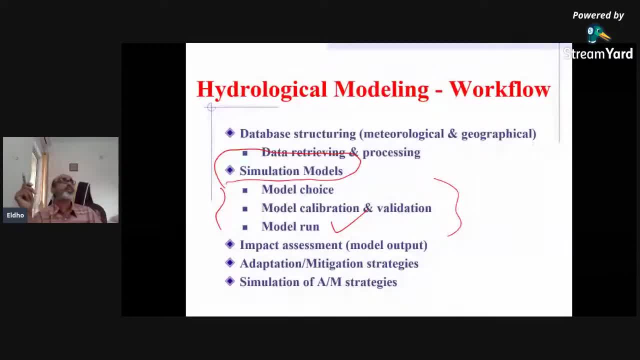 mitigation strategies needs the simulation. so simulation models are very important. so based upon that only we can say that what is going to happen in another 50 years or 70 years, for example. generally nowadays all the the climate change impact, hydrological impact- we generally do for. 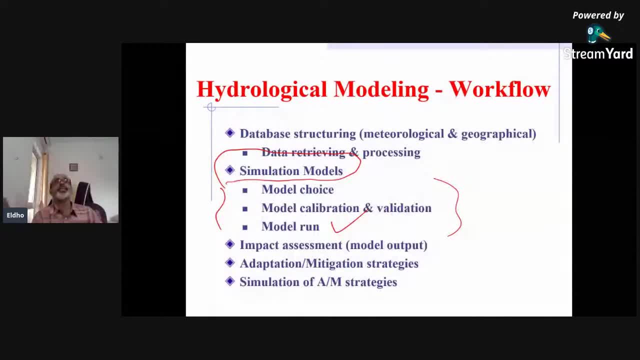 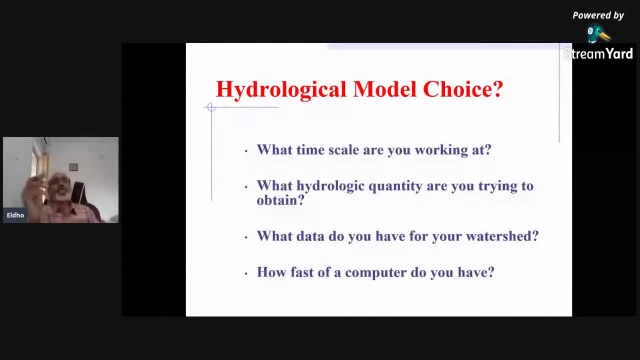 filters d100, so that next, to say, 80 years, what is going to happen? what are the possibilities? of course, as i mentioned, there is so much uncertainty will be there. so these are all mainly. we are projecting what is going to happen. so now i put a few questions. what kind of model we choose? so the 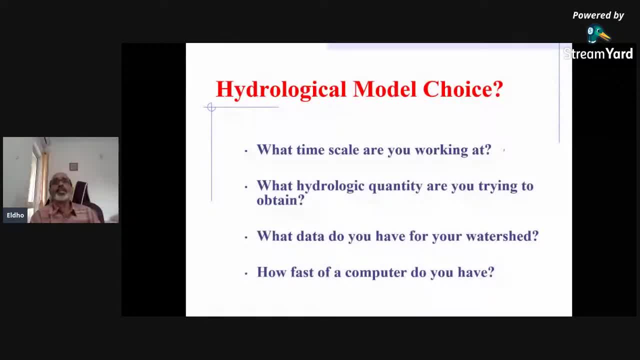 hydrological model choice. so what time scale are you going to work at so that the model questions you need to answer when? uh? hydrological quantity? so whether we need to catch the ground water and surface water or evapotranspiration or only runoff, what kind of quantities you are going? 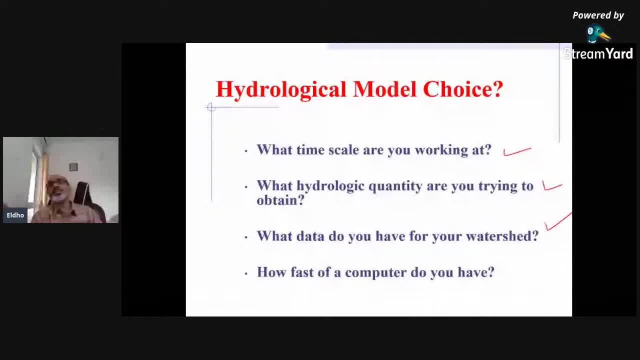 to capture and then uh, water data. so for a river basin disc dot center, you are having a good distribution of a rainfall details available, or whether it is hourly basis or daily basis, or the temperature variation, wind radiation, all the, how many parameters, all these details are available. 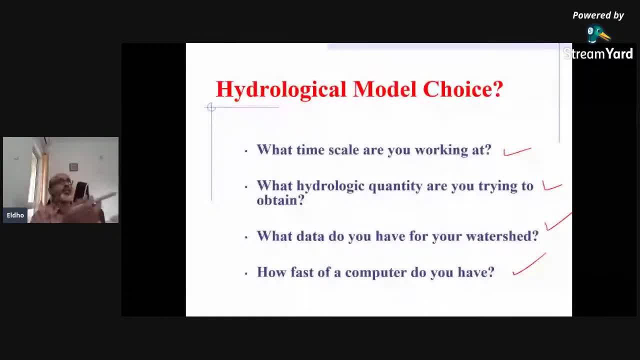 and then, of course, many times some of the phd students, maybe some of my pleasure also, maybe. So you can see that even if you want to run the model till 2100, we need to have a fast computer. So how fast is your computer? 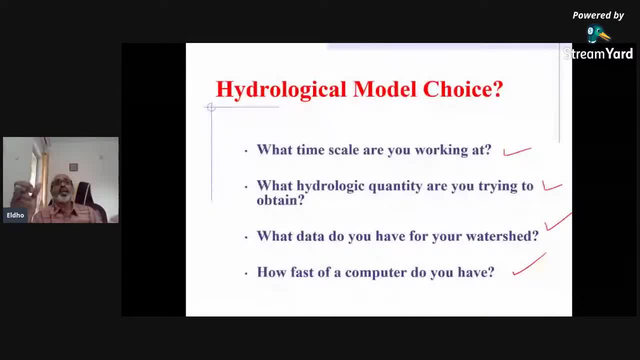 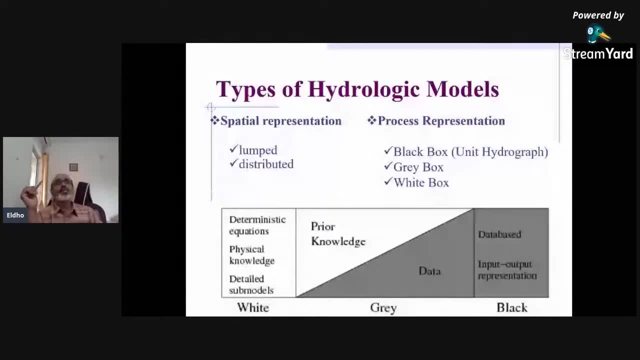 All these questions to be answered So that way we can choose the model. So, as I mentioned, hydrological models are considered. plenty of models are available, So this is somewhat like a lumped model: distributed models and then black box models like even. 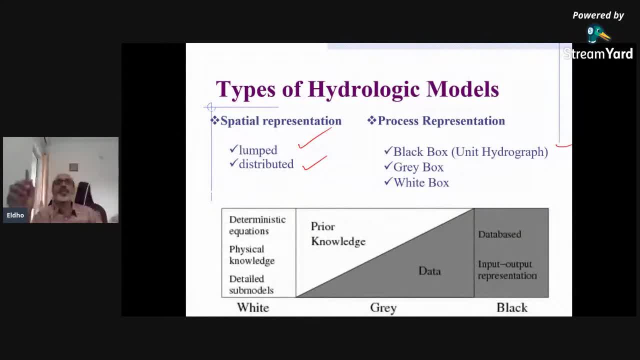 artificial neural network or the similar unit hydrograph model. There are grey box model, white box model. different varieties of models are available. So white box means deterministic equation, physical knowledge, detailed submodels are available. Grey means prior knowledge, only partial prior knowledge, and then based upon that we analyze. 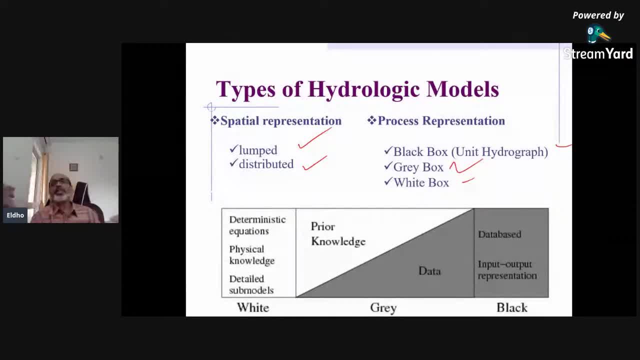 and then black box model means we are having only inflow- I mean the rainfall- and then runoff. So, based upon that, what is happening for the runoff you can predict. So most of the time to get an appropriate understanding of the model you need to have. 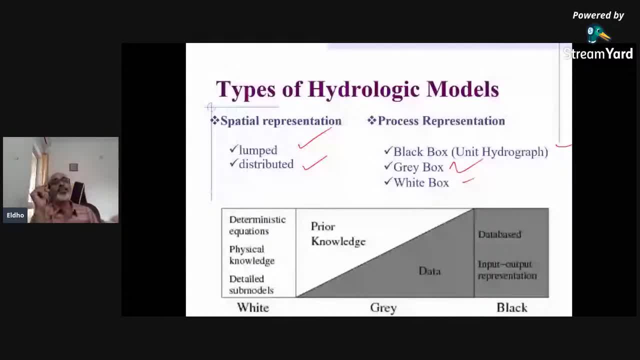 a good understanding of the model. To understand what can happen as far as the climate change is concerned, we need to go at least semi-distributed or lumped models. So, like nowadays, we are using SWAT model or VIC model. variable infiltration capacity. 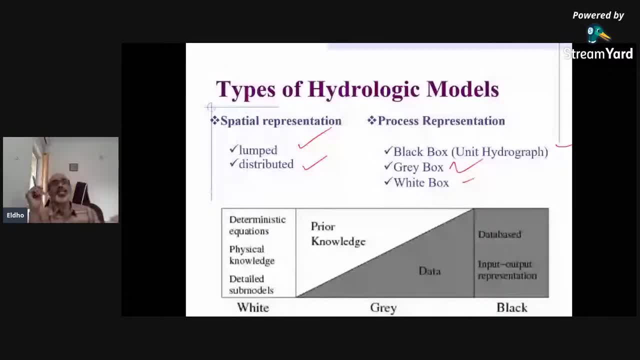 model. These kinds of models are clear, especially when we are going for large scale modeling, like a large Eurovision or for the India country or for a particular watershed resource. So that way a commonly used model for Eurovision scale can be SWAT model, soil water assessment. 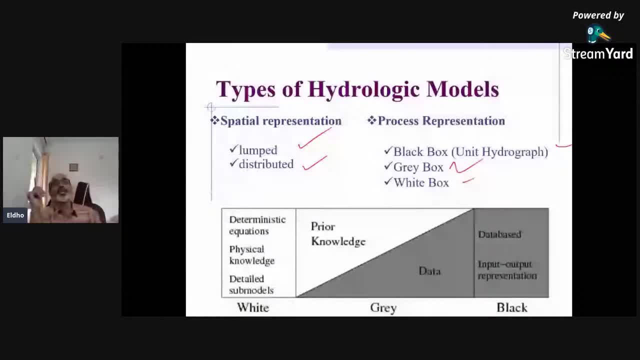 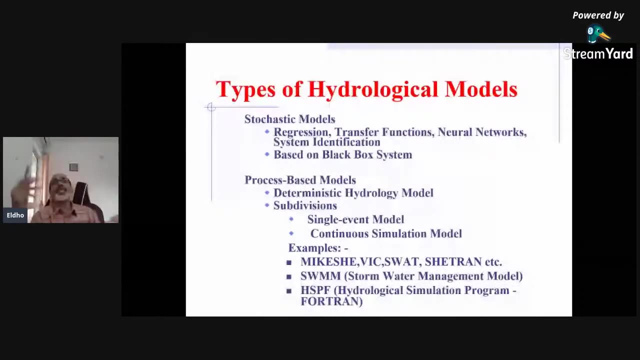 tool, For example, for a country-like model. a grid-based model can be a DIC model or even a Mike Shee or other kinds of models also. we can use it. So now, as I mentioned, there can be also different types of hydraulic models, like stochastic. 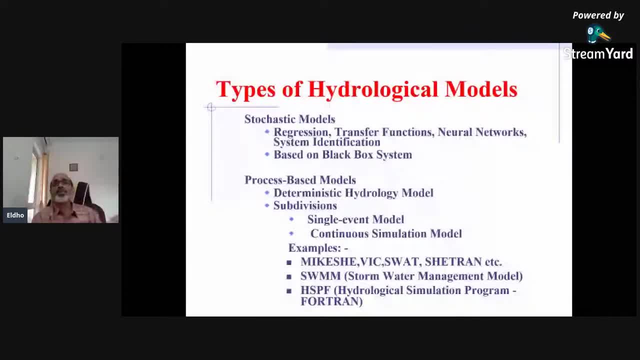 models where the regression or transfer function- all those things can be put in- or process-based models. So this is what is generally we prefer, like a deterministic hydrology model, a single-lead or even a continuous simulation model. So this is what we generally prefer as far as the climate change impact assessment is, 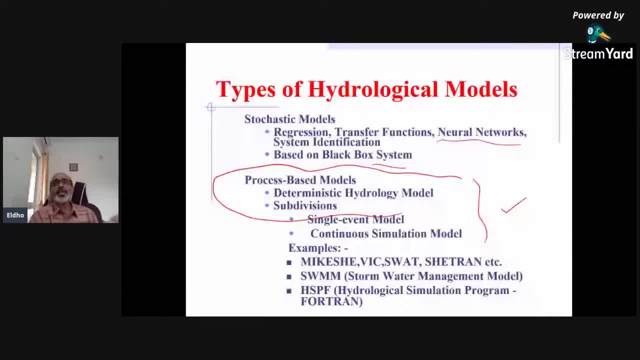 concerned. So, as I mentioned, Mike Shee, VIC, SWAT, Sheetran, et cetera. So this variety of models are available, And then stormwater management model, SWMM. So all these variety of models are available. as far as hydrological models are concerned, 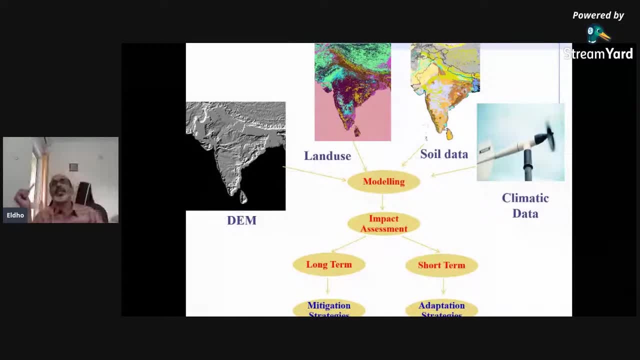 So in all this modeling- so here you can see that we need a lot of data. So we need digital elevation models to get a better understanding of the system, the physical system- We are seeing that a lot of data is required as far as physical system is concerned. 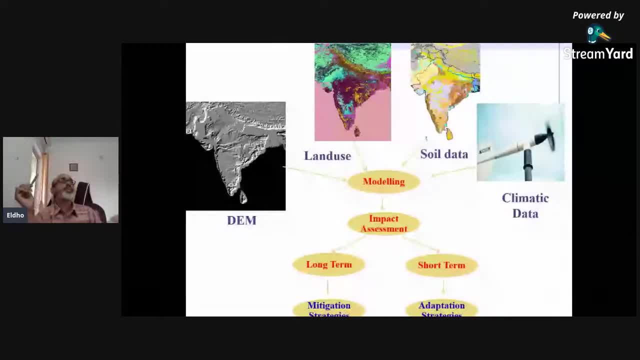 So that is called VEM. And then we should know the land use, land cover. That is also an important parameter. And then we need soil data, since infiltration and so many parameters are there. So all those things, all this data, including the climatic data like rainfall, wind temperature, 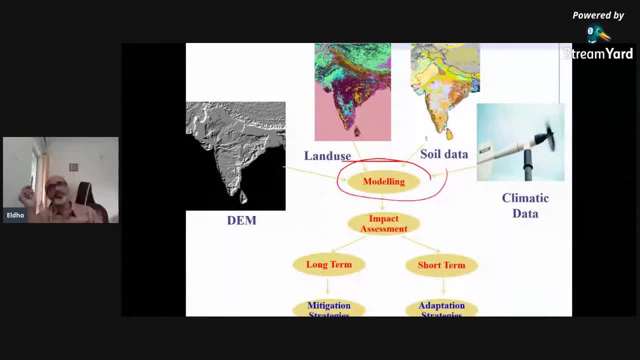 all those things should come And then we can have the modeling. So once the model is developed, And then we can go to the next slide, We can go for impact assessment. So impact assessment can be for short term, So like immediately say, for example, whether there is a possibility of running in this. 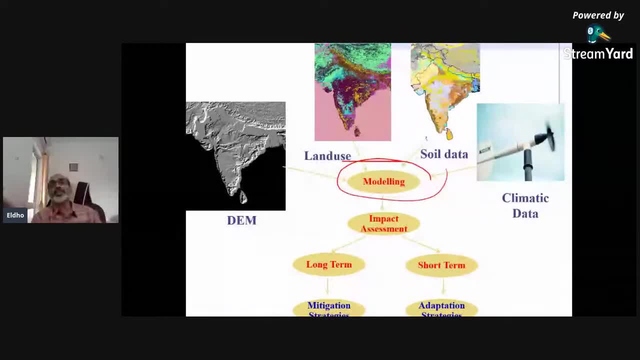 monsoon season, or in few days time or few months time, what can happen? But long term assessment, especially in climate change impact, we do long term assessment So that mitigation strategies or long term planning is possible. So the assessment can be long term or short term. 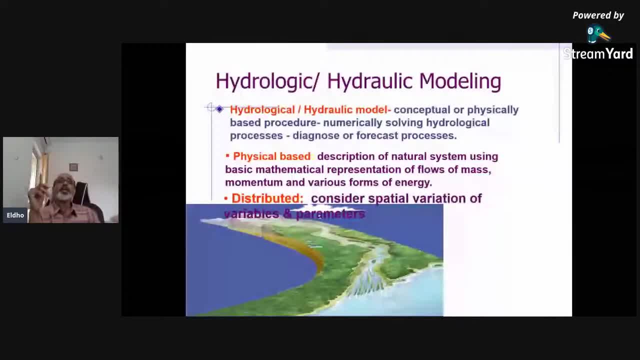 Okay, Okay, Okay. So now coming back to the hydrologic modeling. So hydrologic model, we can classify hydrologic modeling and hydraulic modeling. Hydrologic means so with respect to impact runoff, if you consider a particular overland flow or those things, and then all this will be contributing to the major river or the 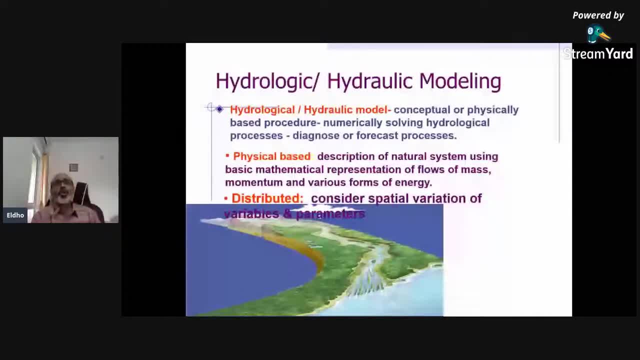 drainage system. And then we need to route this flow so that how it will be coming to the to be to a particular location or particular outlet of the watershed or the river basin. so we need to see So that way, as I mentioned earlier, we can compute it. 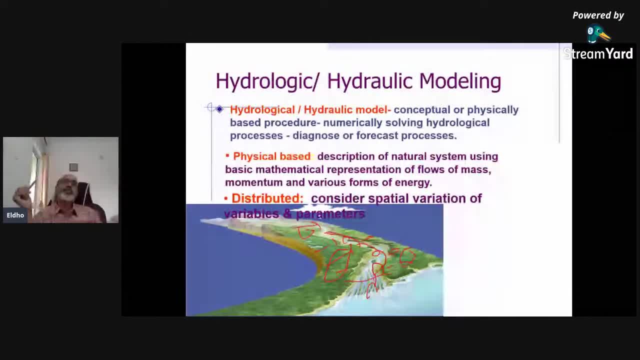 Okay, as I mentioned, at least we are looking for a semi-distributed model like SWAT or VIC model, so that we get a better understanding as far as the climate change impact is concerned. So generally the physically based model. that means we are using basic governing equations. 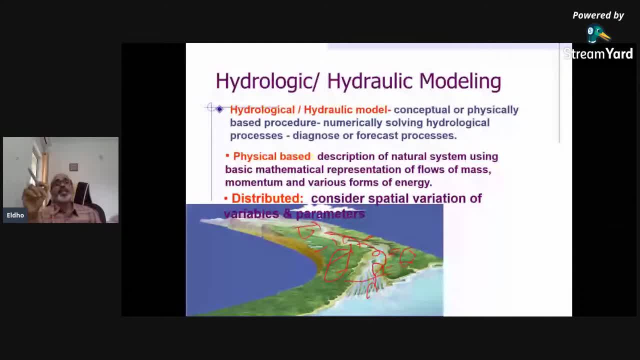 to develop the model. So, but that way, like generally, we use the same-reference equations, the equation of continuity or the construction of mass and momentum, But these kinds of models for long-term simulation it is quite cumbersome but still we can utilize. 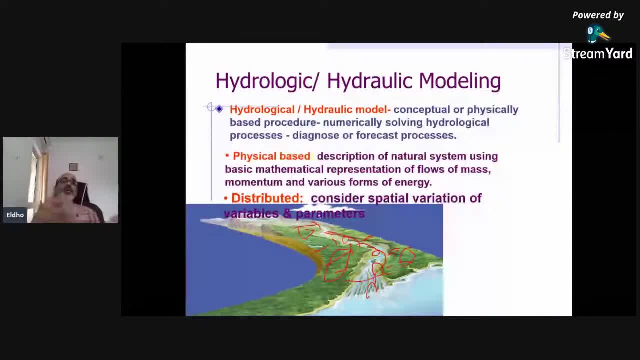 like, for example, SITRAN and MIG-C. all these models are using the physically based model and semi-distributed model, like which is using a CSK, CNKRO number method, that is, by using the SWAT model. 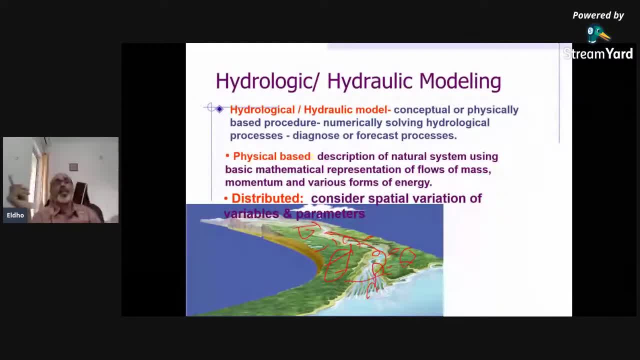 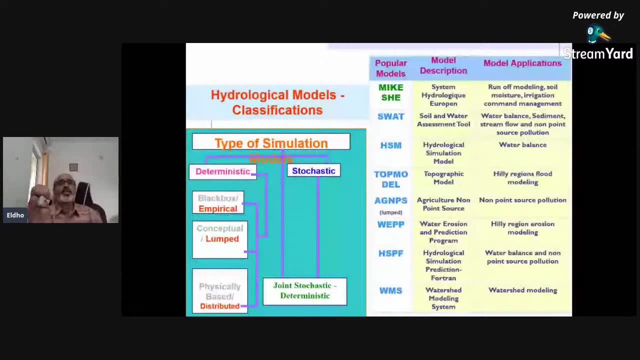 And then say various with respect to various compartments. we can use the VIC model. Anyway, we will be having a brief outlook into VIC and SWAT model. So now, as I mentioned this hydrology model, we can have a variety of hydrology models. 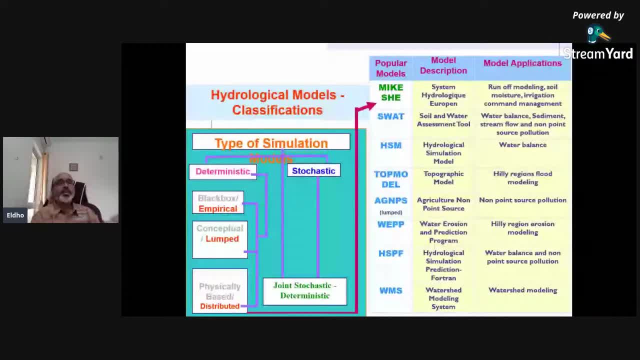 I have shown here what are the varieties that are available. So I mentioned again the black box model, Lambert model or a distributed model, and then stochastic- I mean the uncertainties, all those things can be also put into. so these are some of 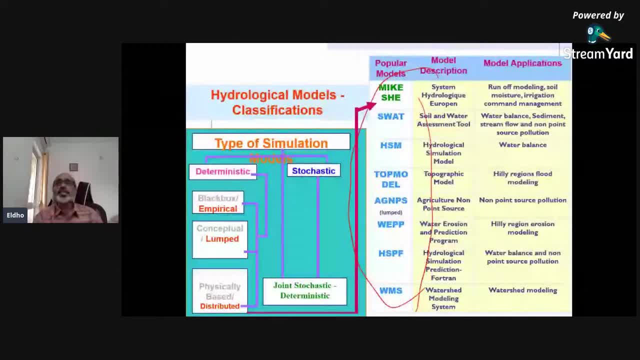 the models available, including- I have not listed here VIC, but VIC is a hybrid model, So this SWAT model is really available. And then these are other some of the models that are available. So these are some of the models that are available. 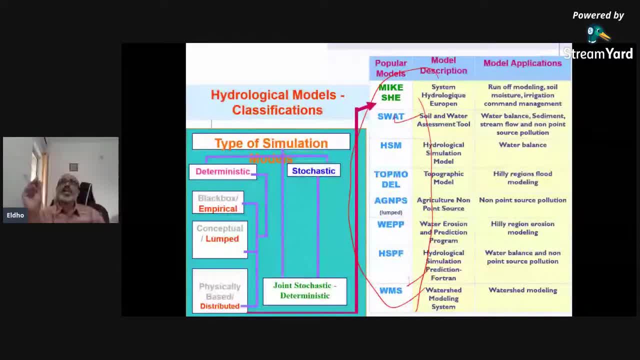 And then these are some of the other models. we need to pay And so, depending upon what kind of applications where, what is your objective, what way you are going to do the studies, accordingly we can use that particular model. So that is what we do generally, but climate change impact is concerned, we need to generally. 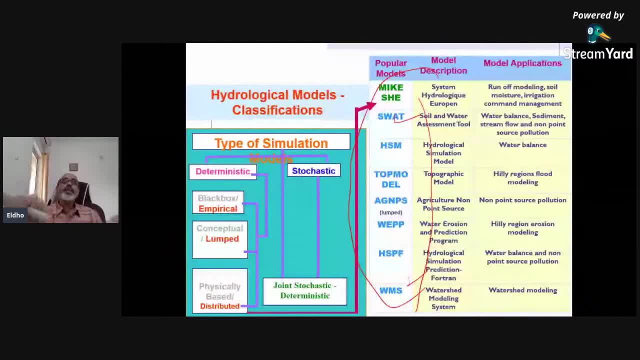 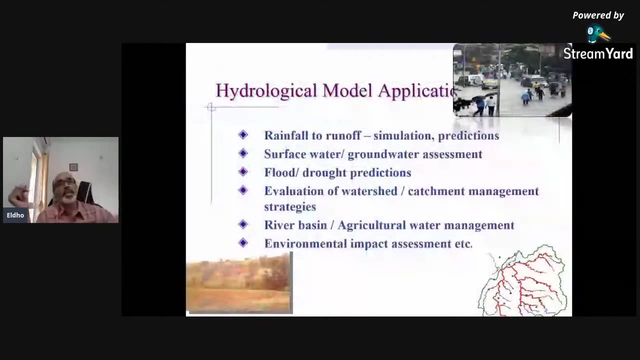 need to go for a somewhat large scale studies, So Minimum SWAT or Mike Shee or Sheetran, or we can go for the VIC model or HO8 model. So these are some of the important hydrological models which we can use as far as the climate. 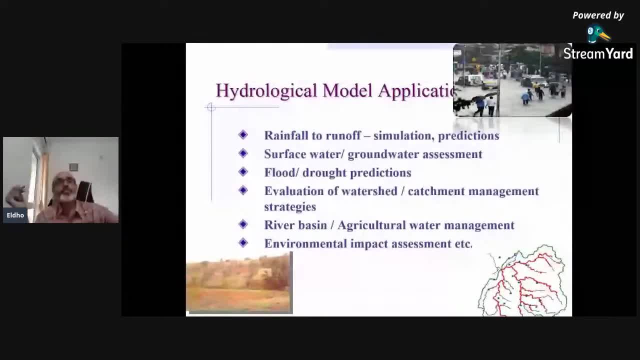 change impact assessment is concerned, Then, as I mentioned so far, we discussed hydrological models and its applications. So there is a large number of applications. So some of the important applications I have listed here, So rainwater runoff simulation and predictions, then surface water, groundwater assessment. 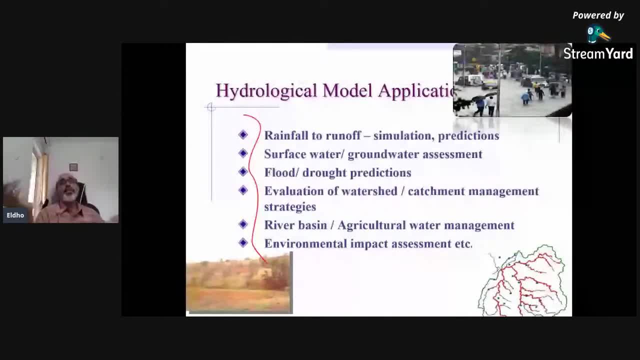 for the considered water pressure. So river basin is concerned, then flood and flood or drought predictions. we can use the hydrological models and evaluation of watershed or catchment management strategies, then river basin or agriculture water management, And then finally, we can also do environmental impact assessment. 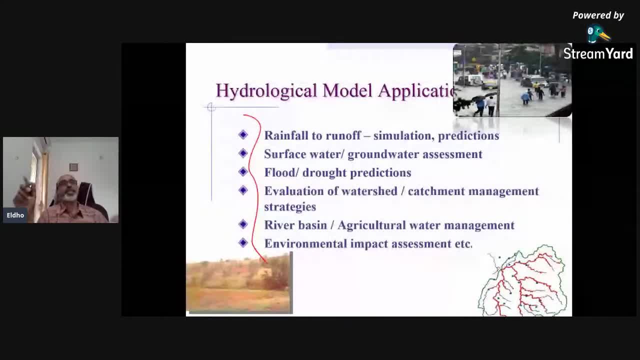 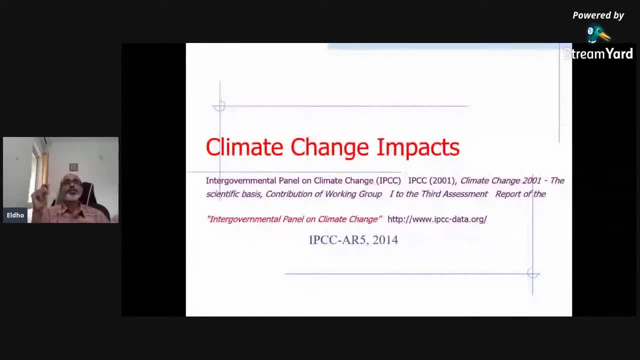 So these are some of the important model application as far as hydrological models are concerned. These are some of the important model applications, So now we will discuss some aspects. So first we will discuss climate change impacts and then how we clamp the climate change impacts. 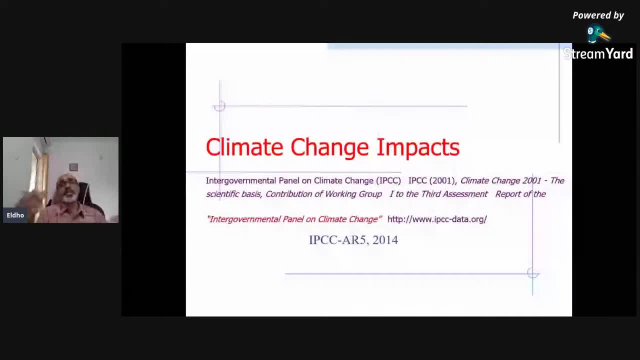 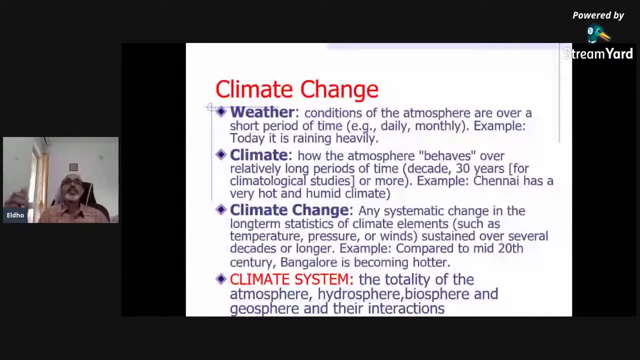 with respect to the hydrological model and then how we can assess the impacts as far as river basin or a particular area is concerned. So, since we have already attended two-three lectures, and then also, many of you may be, climate studies, you have done. 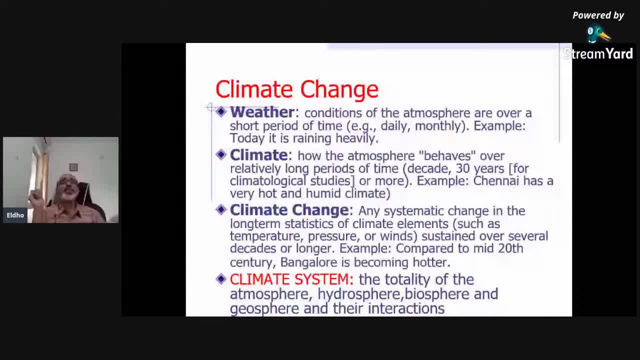 So climate change. so generally we say weather means conditions of the atmosphere which are short periods, say daily or monthly like that, But climate change impacts, so climate change impacts. So climate means how the atmosphere behaves for over a long time, a long period like decades. 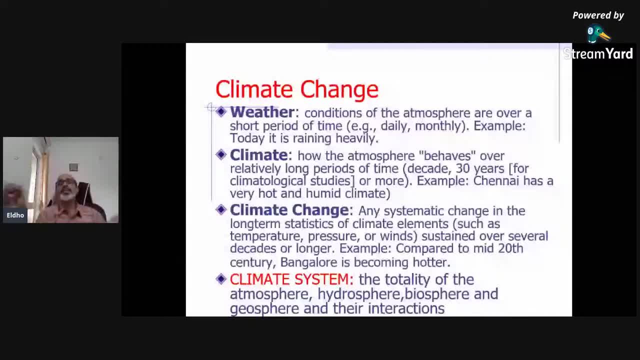 or 30 years, So like, for example, the Chennai has a very hot and humid climate. That means it is, say, 30 years back or 25 years back, that compared to that there is a large change. So that is what we mean as a climate change. 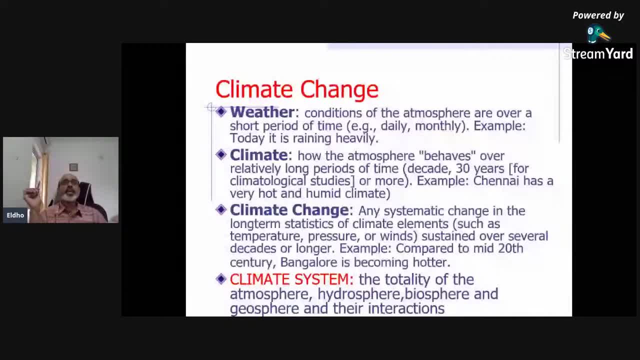 So that way, climate change means any systematic change in the long-term statistics of climate elements, such as temperature pressure range, then the rainfall pattern- sustained rainfall- and then the rainfall pattern will be sustained over several decades or longer. So that is what is say. for example, Bangalore is now becoming more hotter. 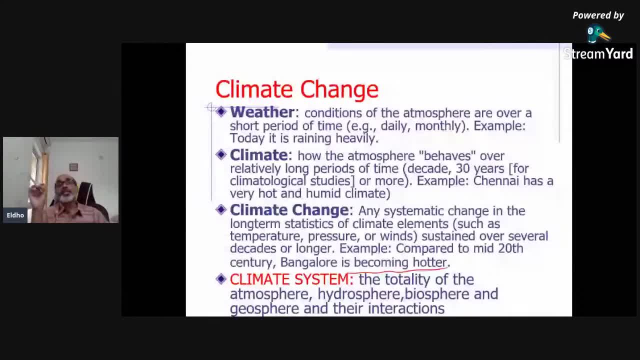 That means it is a climate change or the rainfall pattern. now earlier, say June 1st, most of the time there was a monsoon used to hit in Kerala. So now, if it is coming, most of the time it will be delayed: may be one week, two weeks. 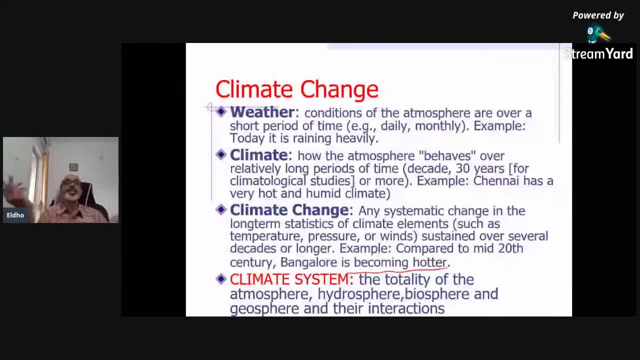 that change is taking place in the last few years, we can see, So that we can say that it is due to climate change. And then, same like that, we can say: the house, the land as well. So, so Like that, we can say that many, many areas, many places, so what can happen with respect to climate change we can quantify, and they say that there is a real climate change. 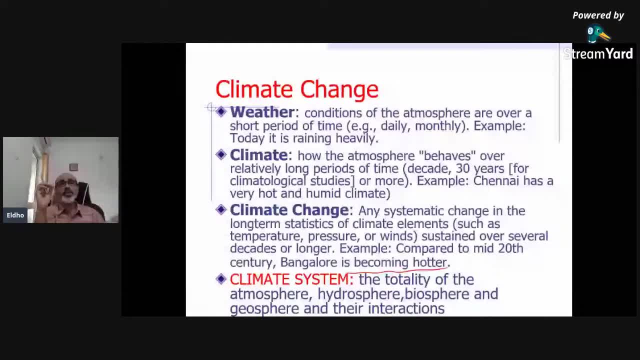 So now, when we want to capture the climate change with respect to hydrology, we need to take the system approach. the climate system, the totality of the atmosphere, hydrosphere, biosphere and geosphere- all these aspects we need to consider and their interactions to be considered. 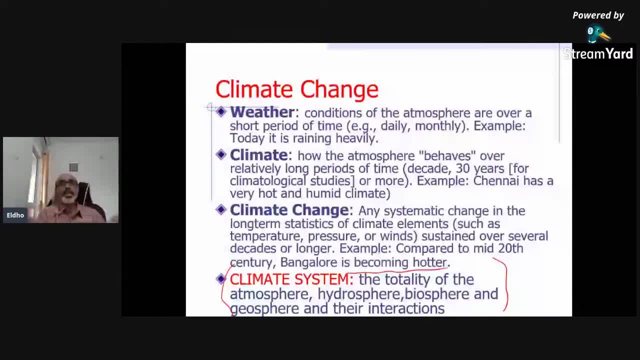 So, though in hydrology we are not going to directly do all those kinds of money, but many of these aspects we get from the general circulation model, GCMs, or global circulation model, whatever we call GCMs. So we get all this data. what can happen as far as the climate system is concerned? 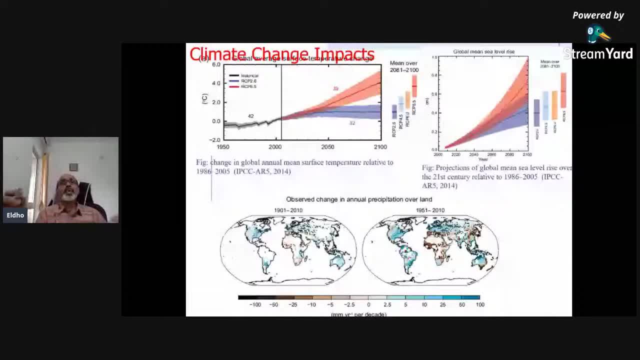 So now, as you have already studied this climate change is. we can see that if you take a long-term trend like, for example, global annual mean subsidence, So if you look at the surface temperature, you can see that if you consider in 2000 onwards, if you look into, the temperature is steadily increasing. the mean surface temperature is keep on increasing. so that you can see what is happening historically. we can see what is happening currently and then the projection by IPCC shows that it is going to increase. whether various scenarios are there, like 2.6, 4.5,, 8.5,, etc. are there, but so which all scenario we are going to choose, you can see most of the times the trend is going to increase. So we are going to see, most of the time the trend is going to increase, whether various scenarios are there, but so which all scenario we are going to choose. you can see, most of the times the trend is going to increase. 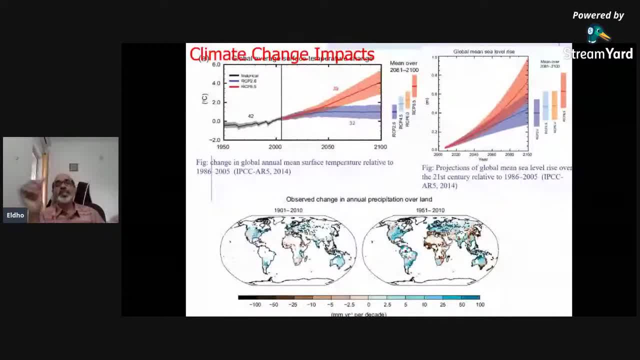 So we are going to see, most of the times, the trend is going to increase And similarly so since most of the time, as I mentioned, there is lot of interaction taking place with respect to the ocean, the third pattern, on the atmosphere system and all the other systems are concerned. 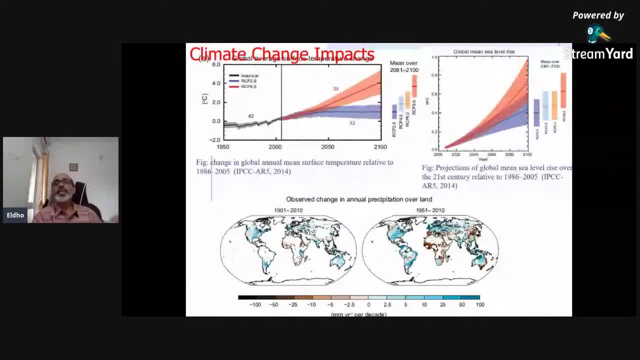 So that way it's also shown that there is a sea level also rising. so this shows that. say, for example, this trend, various trends are all pronted here, so you can see that it is a there is an increasing trend, though it is a very low level, but still it is showing that it is going to increase. 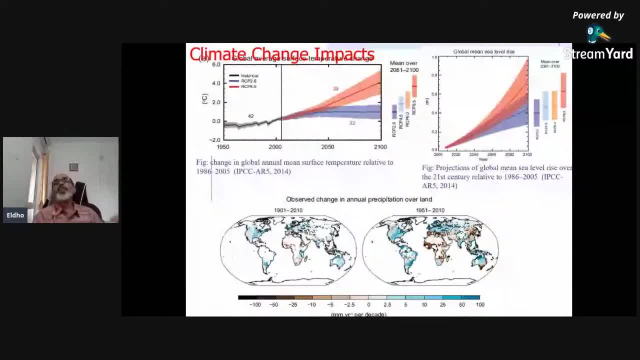 So we say that only with centimeter, but a global mean sea level rise we can observe, and that is already reported and that is documented. And similarly, if you look into annual precipitation over land, we can see that there is also, as I mentioned, many locations there is an increasing trend of precipitation. 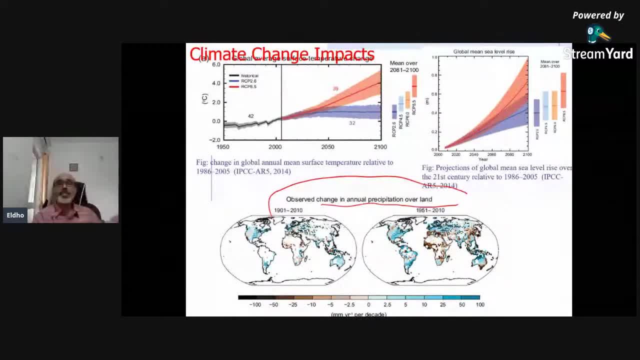 So that is why, as I mentioned, what are the impacts of that? you see that this shows the increasing trend and some places it is decreasing trend, But the most of the places there is a precipitation change from last 100 years or 110 years, you 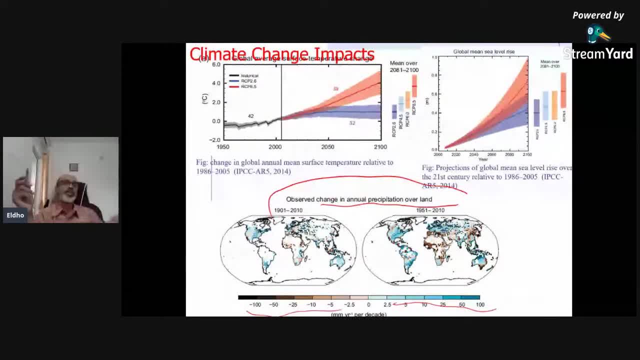 can see there is some increasing trend in many locations, So some places decreasing trend also. So this all indicates there is a climate change and it is indicated. So it can be in terms of temperature, it can be in terms of sea level rise or in terms 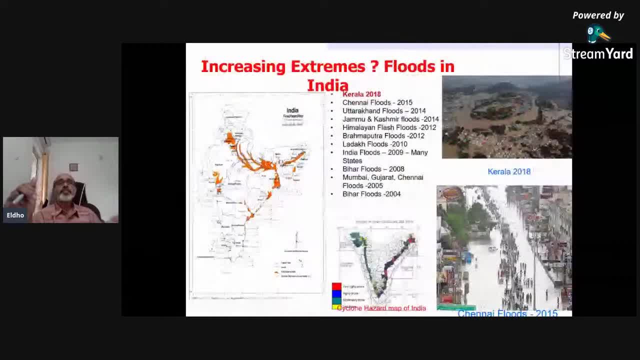 of annual precipitation over the land. So now, in terms of hydrology, If you correlate this and then if you study what is happening last 20 years, in India, So, for example, many locations you can see starting from 2004,. I have listed here number. 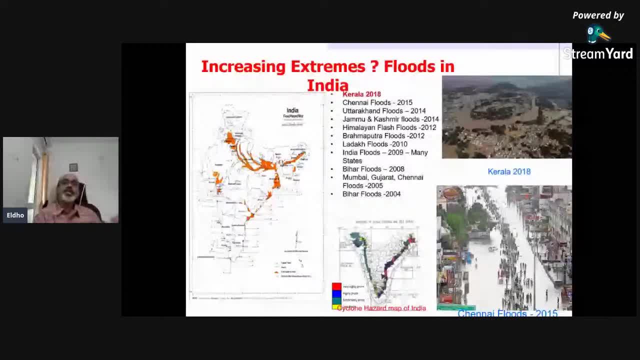 of, say, severe flood events. you can see that there is number of severe flood events, Though in a place like India, in most of the monsoon season there can be flooding, but severe flooding is observed in the last few years. Okay, 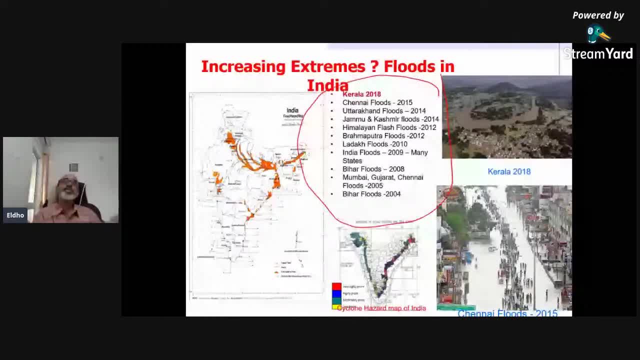 So at least every year we can see these kinds of phenomena. So the latest what I listed here is 2018, but say last year, and this year also, there was severe flooding in Bihar, Assam, etc. So but many times you can see this is some scenario from, say, Chennai flood, Kerala flood. 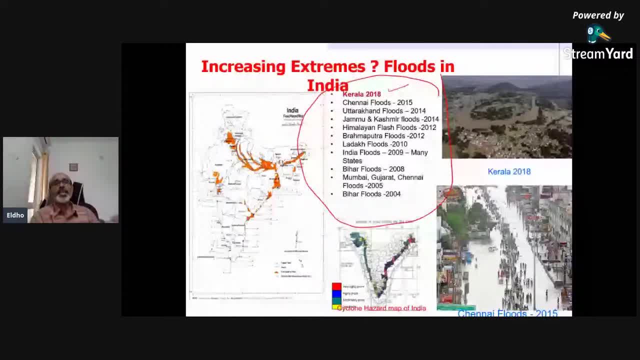 etc. So here and then- not only that- the cyclone intensity, you can see that these are all cyclone facades. map of India. So there also you can see that the cyclone activities also increased. So these are all, whether, when you correlate all those things, we can say that, say somewhat. 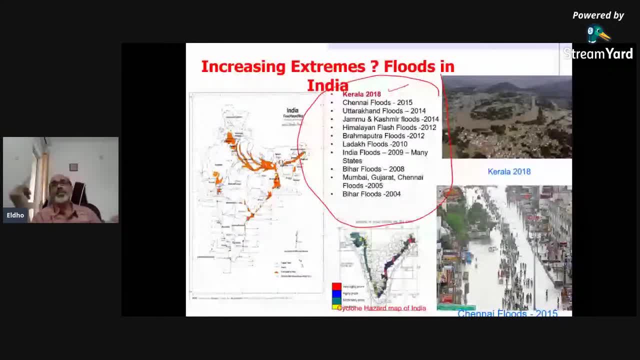 we can say that there is an impact. there is an impact of climate change with respect to the especially hydrology concerns in the flooding. the various other other problems are also increased. So then, this shows the increasing extremes. so, as far as India is concerned, 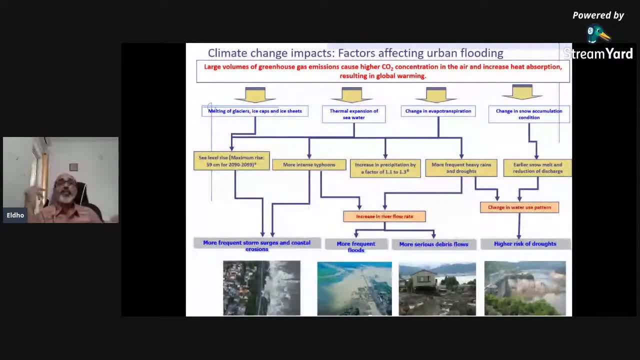 So now climate change impacts. factors affecting, say, for example, now flooding is is felt very severe, especially in urban areas. So you can see that when you look at the large volumes of greenhouse, the effect is very clear. it can be melting of glaciers, thermal expansion, seawater changing, evapotranspiration. 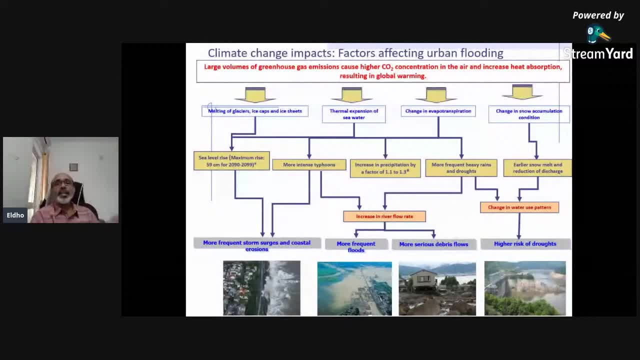 changing snow accumulation. all these conditions can say, come together And then you see that finally that can be increasing river flow rate and then there can be a change in water use pattern also, So that all lead to more frequent floods, More more serious debris flows and then high risk of droughts. 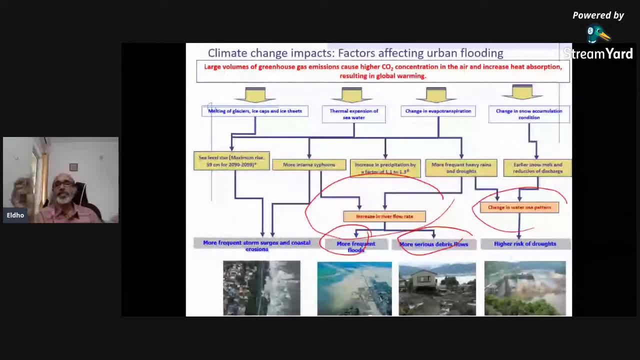 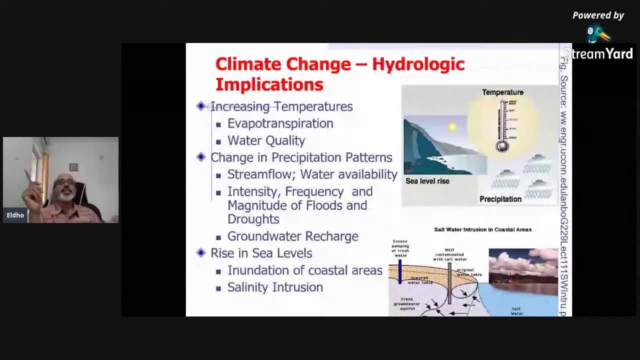 So these are some of the visible aspects we can see as far as the climate change and its impacts are considered. So now we can come back to climate change, the hydrological implications, So, as I mentioned, the increase in temperature, so that will be leading to evapotranspiration. 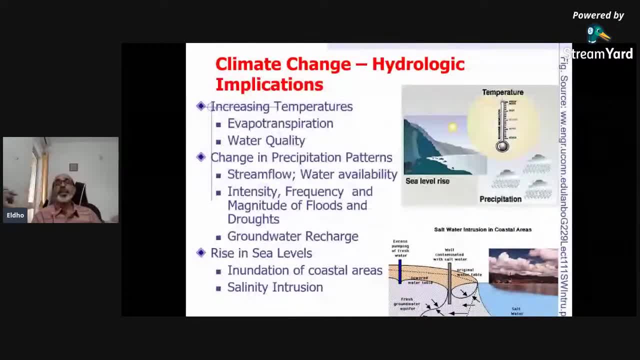 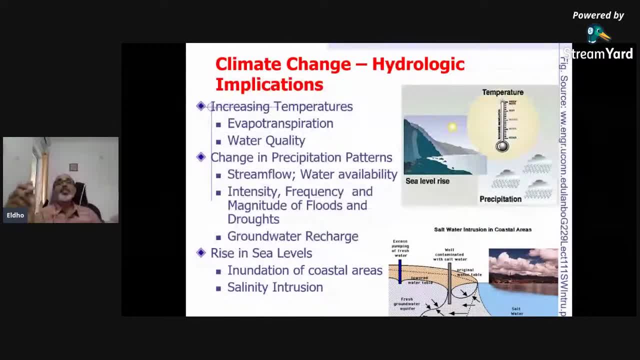 So that will lead to more evapotranspiration. There can be issues led to the water quality, So that will lead to more evapotranspiration, And then changing precipitation patterns So you can see the stream flow. the runoff can increase due to high wind and rainfall. and then water availability can change, So it can be density, frequency and magnitude of floods and droughts can increase, and then ground water recharge also can reduce. especially the rainfall takes place in short duration- high wind and rainfall, so there is no time for so much water to percolate down or we. 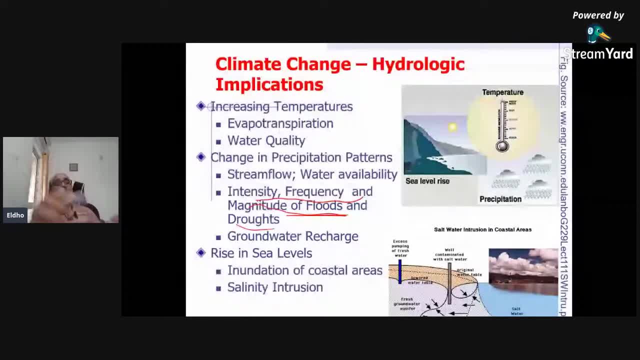 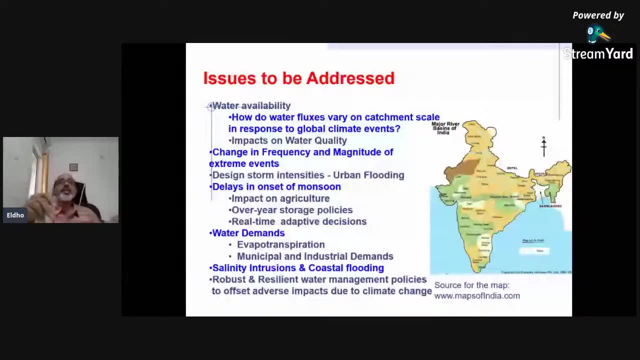 the recharge will be decreased, so that also can happen. and rise in sea level, inundation of coastal areas, and then of course, that also can go to and lead to salinity intrusion. so these are all climate change and hydrological impacts. so that way, when we look into, say, what are the main issues, as 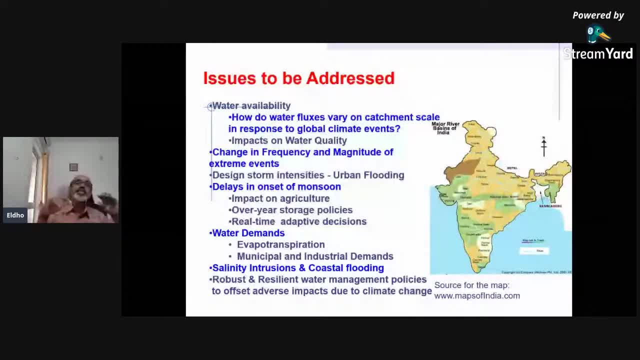 hydrologies. so when we deal with the, the changes the climate, the impacts of climate change, climate change with respect to the hydrologies constraints, where a number of issues we need to address, a lot of research work is to go in, and that can be either river basin scale or watershed scale, or 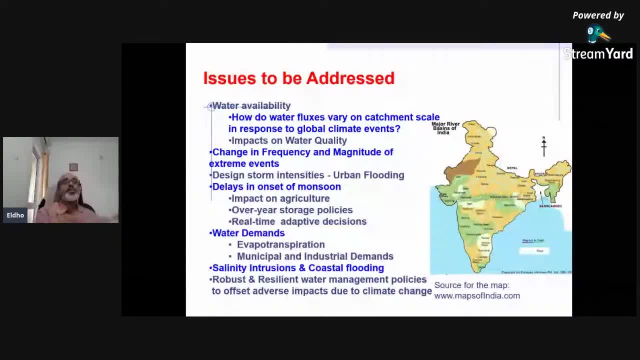 even the forest state level or the country level. so we need to look into. important aspect is water availability. so how do water fluxes vary on time catchment scale and then what are the changes in frequency and magnitude of extreme events? as i mentioned, funding is happening in many locations. 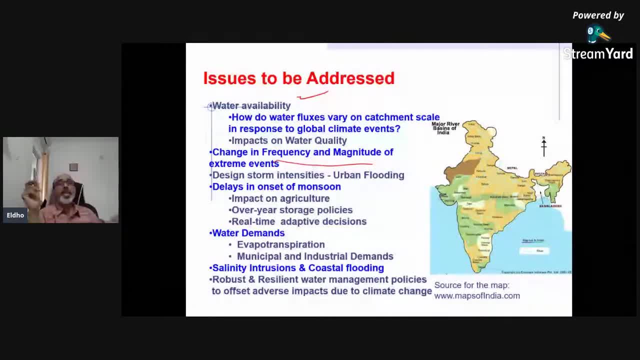 in most of the years. then what is what can happen? and then, as i mentioned, there are delays in onset monsoon, so the monsoon is delayed, so so most of us say in a country like india, so you say the farmers put their seed based upon the 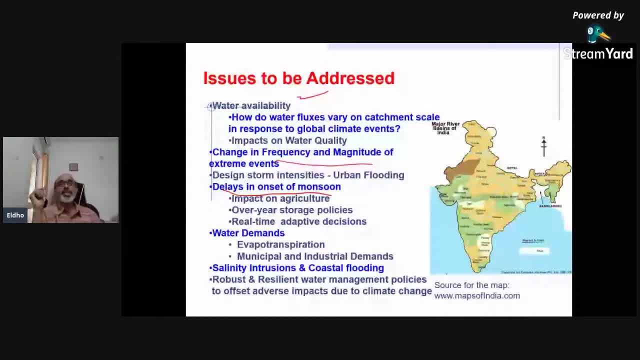 arrival of monsoon. so there will be impact on agriculture and over here storing policies, as reservoir storage will be affected, and then there will be so many changes that will be that will be new to account, and then water demands due to increase evapotranspiration. then there will be. 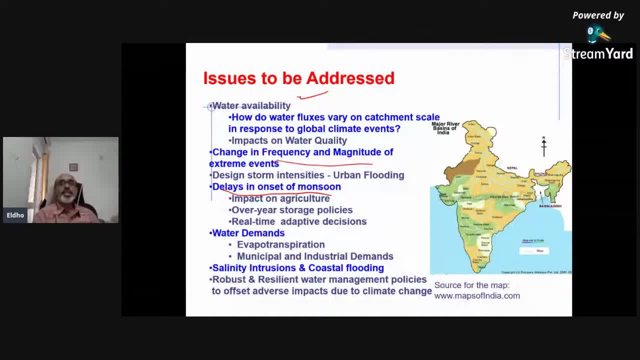 huge demand with simple and industrial demands, can change and then coastal region, especially salinity inclusion can take place, and then also the cost of funding. so these are the some of the important issues to be addressed as far as the, the climate change, that as far as hydrology is concerned. so that way, the climate change impact on water source. so, as i mentioned, hydrocyclics, so some of the important points i have listed here. hydrocyclics predicted will be more intense rainfall as well as increased drought, so the rainfall will be the rain fall, total rainfall. that happens in few events- high intensity. so that way the the there will be, then the drought also may increase, since the rainfall takes place in few years and then afterwards they will not be delayed and there is predicted increase of extra rainfall and intensity of daily rainfall is. 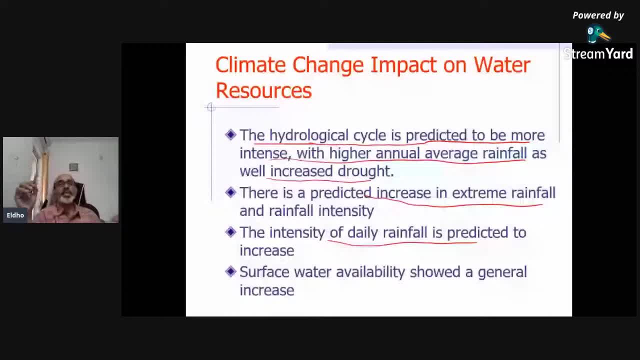 predicted to increase and that way surface water, which is showing general increase, but we can store these, all the water will be, say, will be going through the river and then the flooding will be the final impact. and that way, when we look into policies are concerned, we need 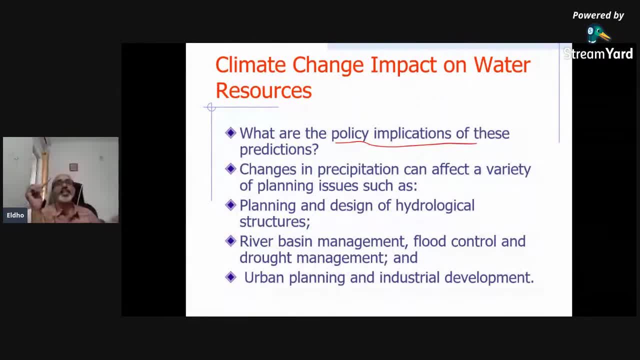 to make policy implications. what are the important policy implications? and then, so the change in precipitation can affect the variety of planning issues, such as planning and design of hydraulic structures. so we have a large number of dams. so if the dams are there, our reservoirs are there and 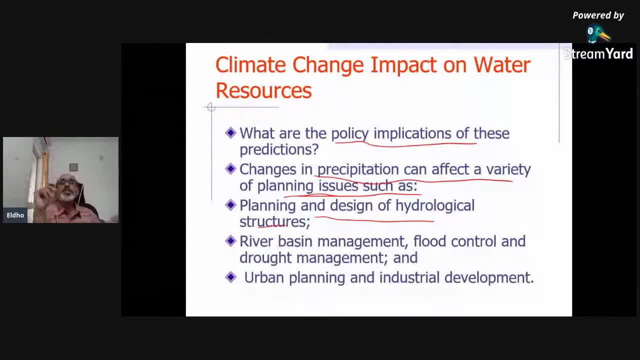 then if you don't have sufficient water, then what is the meaning? so we need to plan how we can do the changes with the climate change. we need to plan how we are going to operate the reservoirs and what will be its implications, and then, in a holistic way, what kind of river basin. 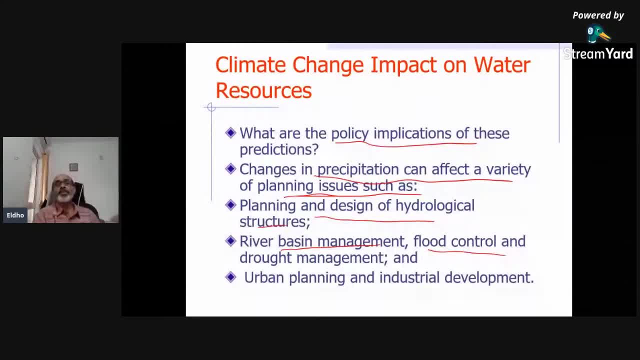 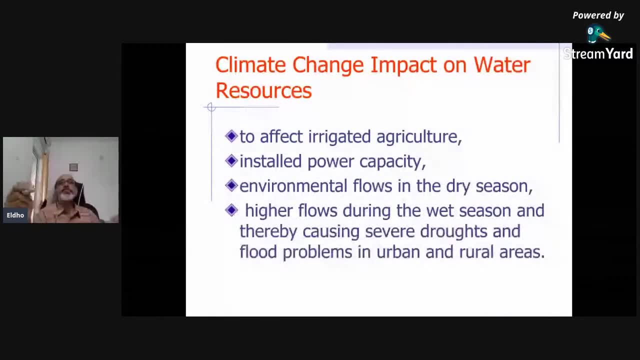 management. then, as i mentioned, flood flood is a major cause. flood control and drought management are possible. all these aspects we need to discuss in a in an effective way, so that way, climate change impact on water source- some of the important aspects where we knew i have listed here, so like to. 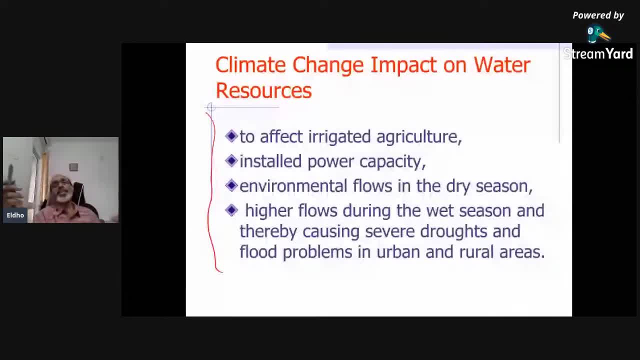 agriculture. so the country like india hardly. the irrigation is about 40 to 40 percent and remaining 60 percent is farmers are depending upon the rainfall, so that way a lot of impact will be there. and then we have got the power productions concerned: around 20 percent power is coming. 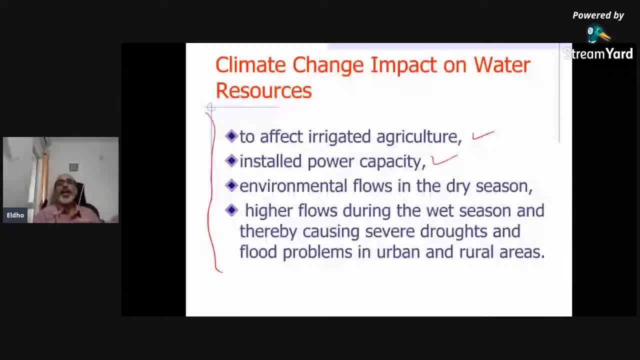 for hydraulic hydroelectric power projects. so that will be affected then environment and flow in the dry season. so that is another problem. so when the the number of events of rainfall will decrease, so then the flowing the river will be drastically reduced after the rainfall and then there will not be any. 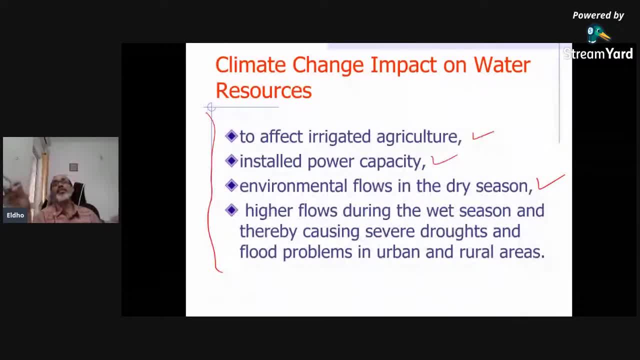 environmental flow that will affect the flora and fauna, the fish will be affected, the all the system will be affected, and then higher flows during the bed season, and that they're causing severe droughts and flood problems in urban and rural areas. so these are some of the important. 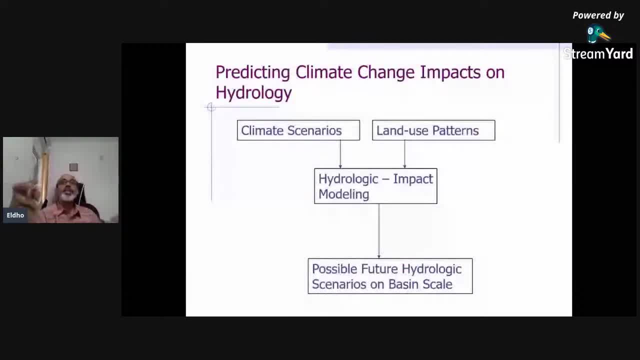 impacts as far as climate change is concerned. so that way, when we go for a proper assessment, we need to see and we need to predict climate change impacts on hydrology, we need to see the climate, various kind of scenarios, and then, of course, as i mentioned, the land use pattern is very important. 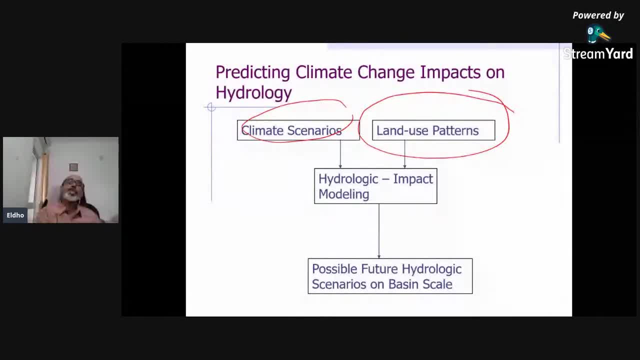 so land use pattern. both will be coming together. so these both aspects we need to consider to study hydrologic impact as far as the climate change is concerned and then we look for possible future hydrology scenarios on either a river basis scale or for the entire country is concerned. 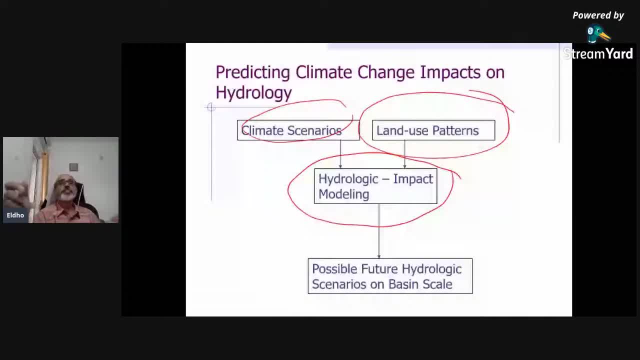 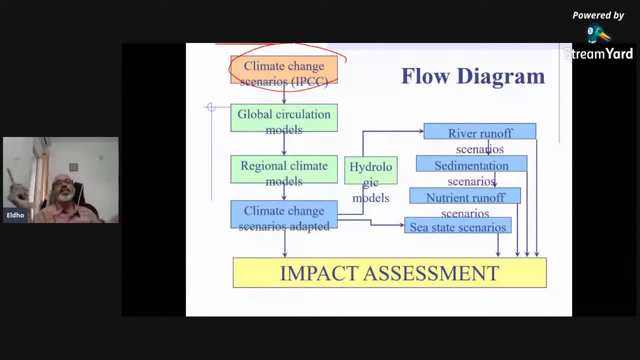 so that way we will do this kind of assessment. so this shows, so we have the climate change scenarios which we can get through the various gcms from ipcc or other area, other agencies, using global circulation models and then, or we can also have regional climate models and then we can assess. 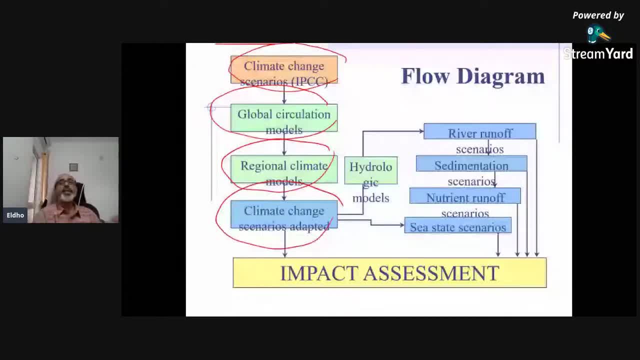 the climate change scenarios, uh, with respect to what is happening, and then that will be the input for the hydrological models. so, using the hydrological models- and we will be- we can identify how much is the river runoff taking place, and then sedimentation, nutrient runoff, the sea state scenarios, all those things we can do and that will lead to the impact assessment. 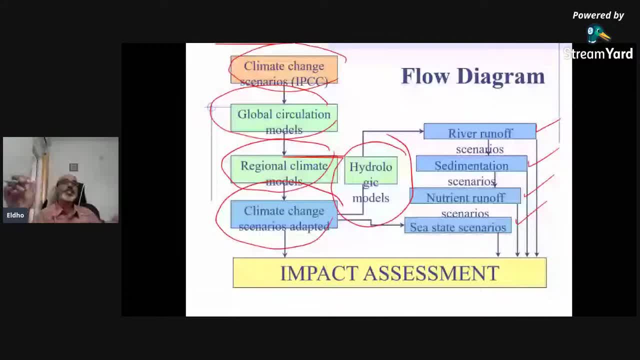 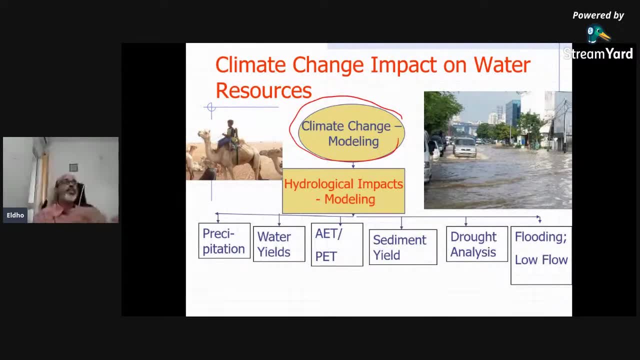 so that way we do the uh, the hydrological impact assessment, as far as the uh, the, the, the climate change is concerned. so here, as i mentioned, there will be climate change modeling and there will be hydrological impact model. so there, the, the input coming from the climate change. 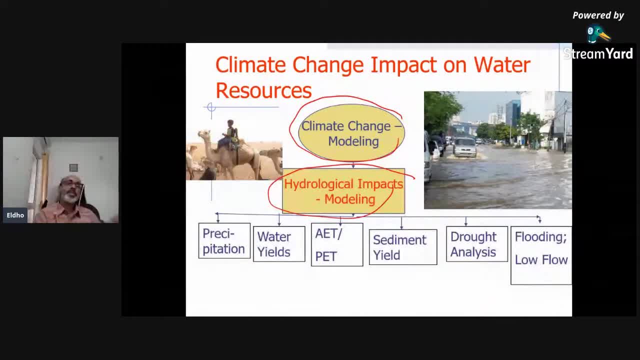 we put into hydrological model, and then that will give the precipitation with the input and from that water yields the runoff, then evapotranspiration, sediment deal, and then sometimes we can also go for drought assessment and flooding or all those things we can do in a similar way. so now, uh, we, we have seen the climate change and the relation between hydrology. 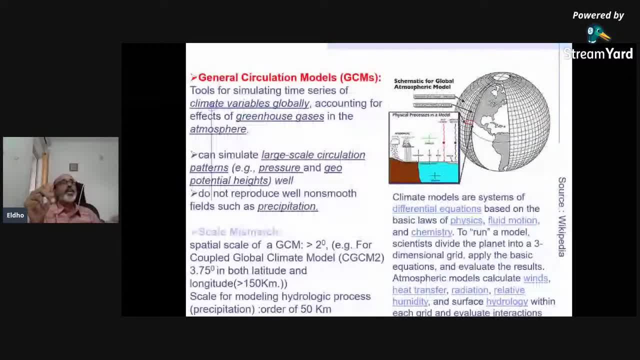 and now, climate change impact assessment, how we can go for modeling. so, as i mentioned, general circulation model is the available tool which we can directly utilize as far as the, the, the climate change impact assessment, is concerned. so this we can, the data getting from the gcms, we can. 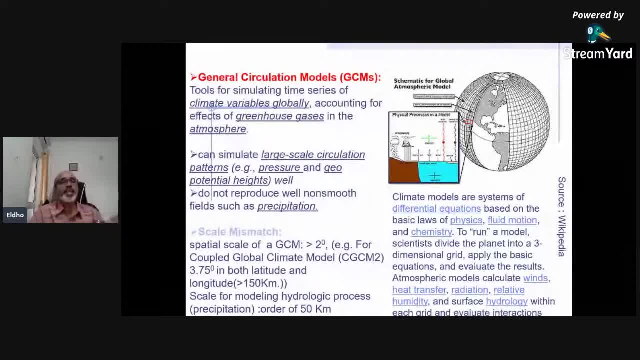 use for simulating large scales, suppression patterns, and then only problem is that the scale mismatch. so the the spatial scales in the gcm may be more than two degree, like that. but whenever we, if you want to have some uh, say reasonable, uh, the climate change impact on a river basin scale or on 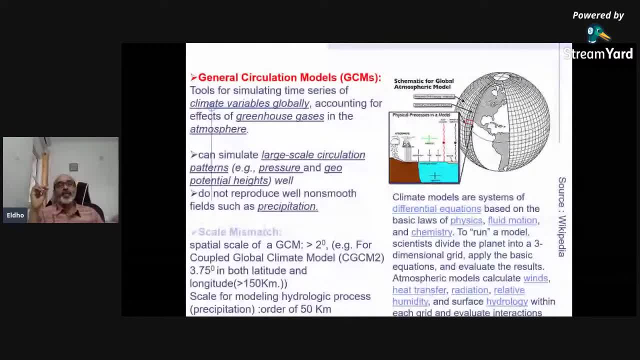 a particular area is concerned, we need to go for at least 0.25 degree or 25 kilometer by 25 kilometer. so that kind of assessment is required. so that is a, the scaling is a. scale mismatch is a major issue. so anyway, i know i am not going to the gcm data. gcm details you can see in literature. so it is. 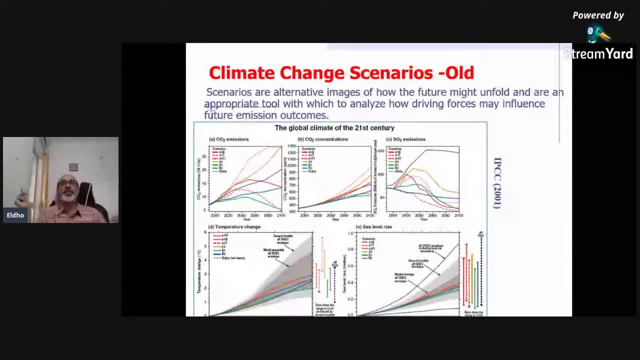 early to maybe also probably presented by some of my other colleagues. so in a climate change scenario used to have a scenario like a1, b1 or a1b like that very scenarios are there. so because i'm going to present the two cases, so one case will be based upon this. so all the scenario like a1, a2, b1, b2. so 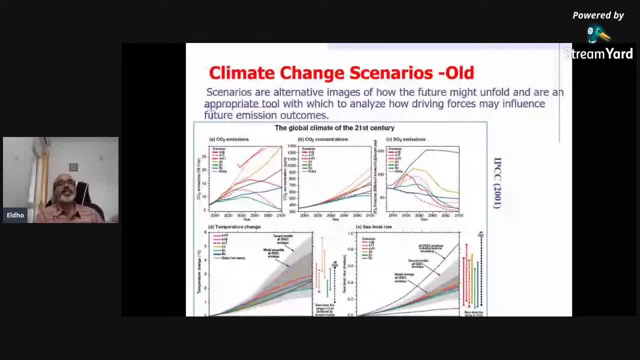 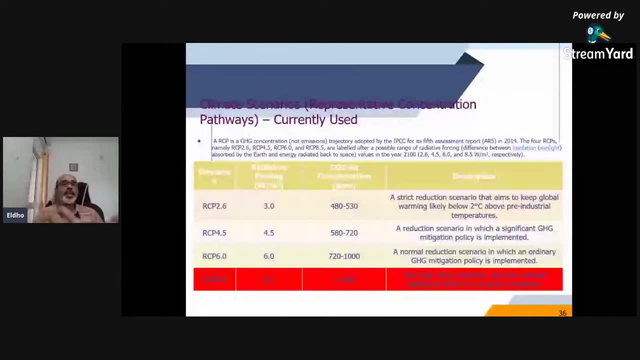 these kinds of scenario with respect to the climate, uh, the seawater emissions and its impact, so with respect to temperature and sea level rise. so that is one way of all assessment and currently used assessment is using the climate change representative concentration paths, which is so we generally use, like rcp 2.6, 4.5, 6 and 8.5. so generally i have optimistic way what can happen. 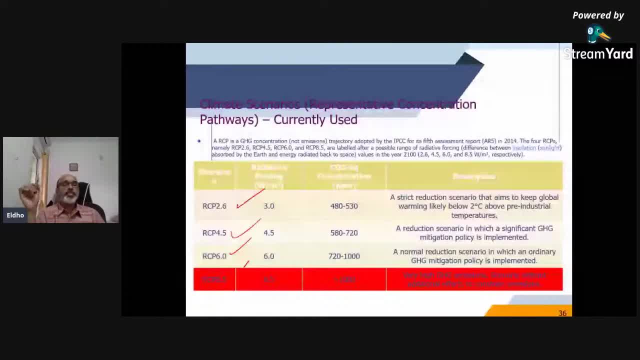 when you say for future projection is we can say with respect to rcp 4.5 and extreme cases, we can say that with respect to 8.5, i mean a lot of severe destruction, a very high gst emission scenario. without additional efforts, uh, to cut strain emissions takes place, then that is a severe 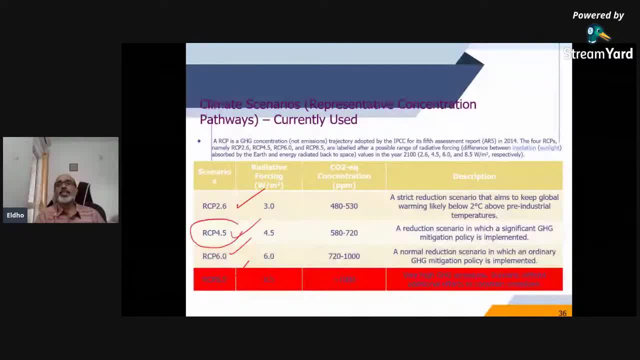 destruction: rcp 8.5. rcp 4.5 reduction scenario in which a significant dht and uh emission policy is implemented. so this is the most optimistic scenario and then, if you, the best scenario is 2.6, but that may not happen now. the current scenario is constant. so that way and now? 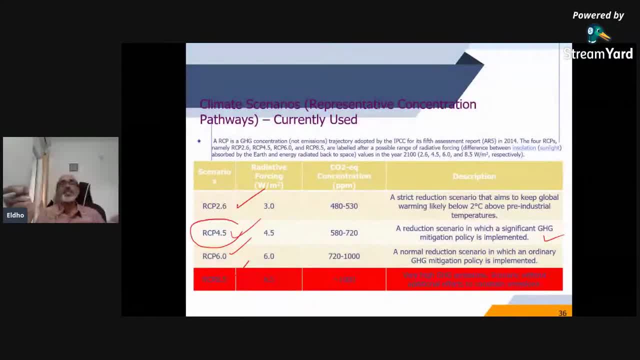 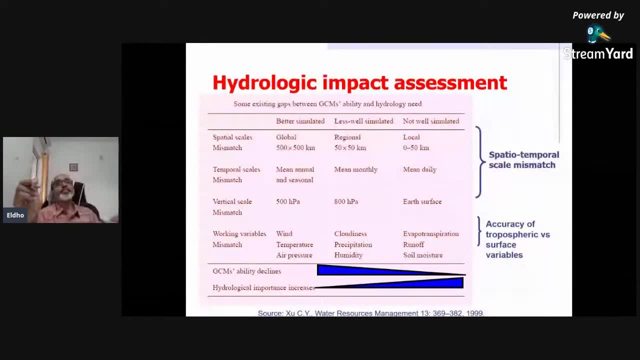 nowadays we use rcp scenarios for the climate change projections and then that is uh. based upon that, only the hydrological impact assessment also done. now, coming to hydrological impact assessment, as i mentioned, there is always a scale mismatch. so now the spatial scale, so you can see that um. 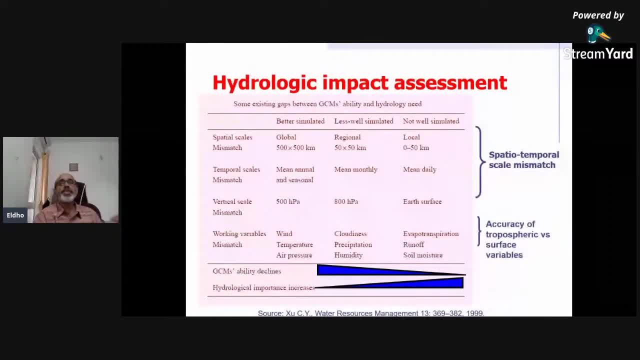 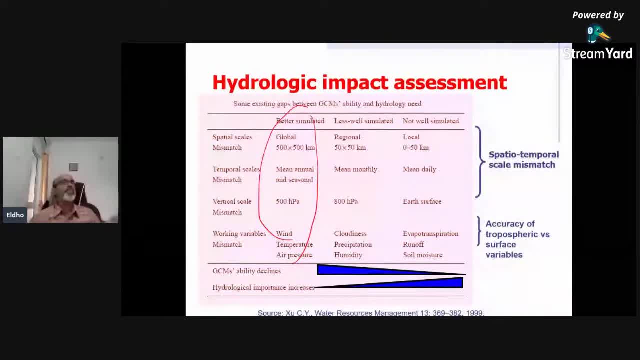 the area decreases. if you consider small river basin or this particular catchment is consent, then you can see that the ability of the gcm decreases. but hydrologist consent, if you say for the entire country or the for the global scale, then there is no meaning since we the hydrology. 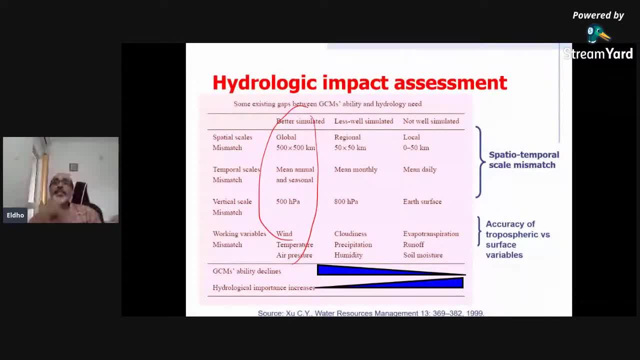 is what we are feeling: the rainfall, what is happening the runoff, what is happening the drought, what is happening all those things we need, the local we base so, for example, in the water sharing or a small river basin, or a large river basin. all those assessments need to be done so that way there is special temporal scale mismatch. so that is what is a 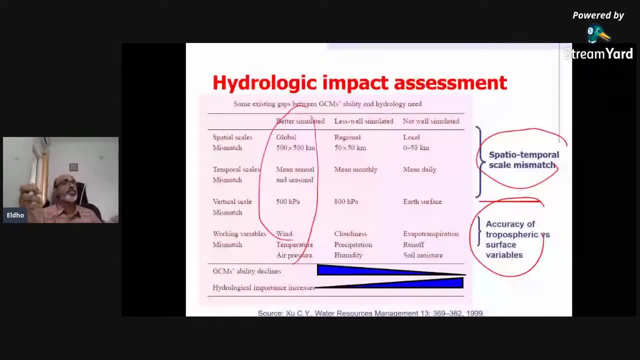 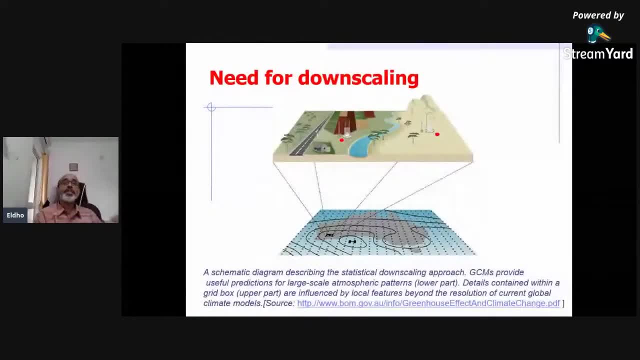 major challenge as far as hydrological impact assessment, as far as the, the climate change impact assessment is concerned. so we need to go for down scaling- so this is coming from the gcm- and then we need to go for a small river basin or a or a particular, uh, even a watershed scale. then 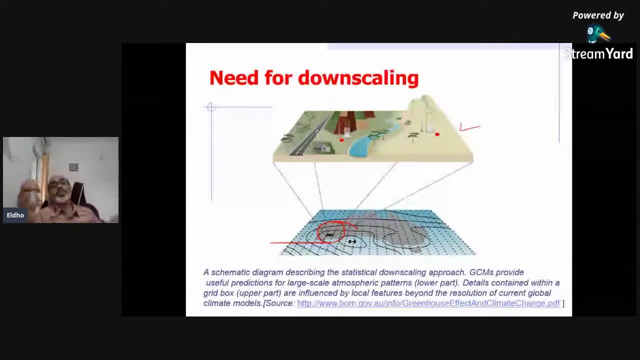 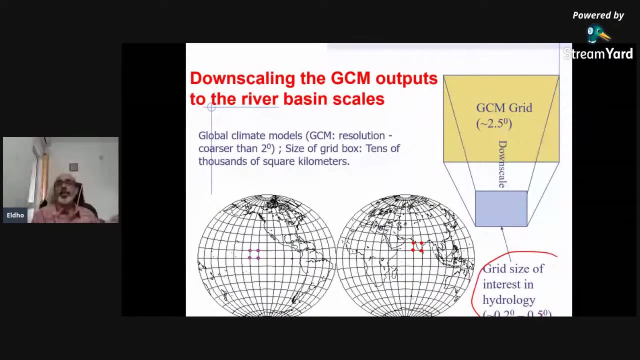 only we can say what is going to happen, and that will be only useful to society, useful to the people, only useful for the, for the planning and management. so that way you can see that, um the gcm grid, 2.5 degree, we need to go for 0.2 degree or even 0.1 degree, so this is the preferred grid. 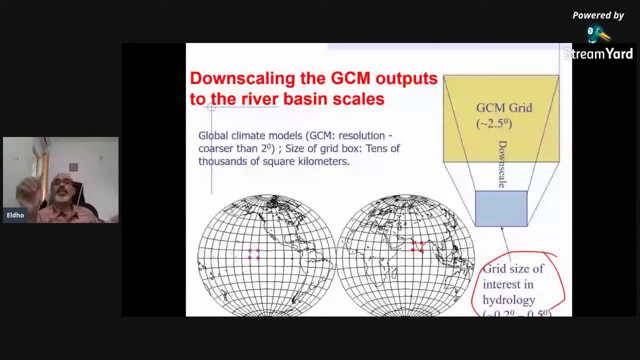 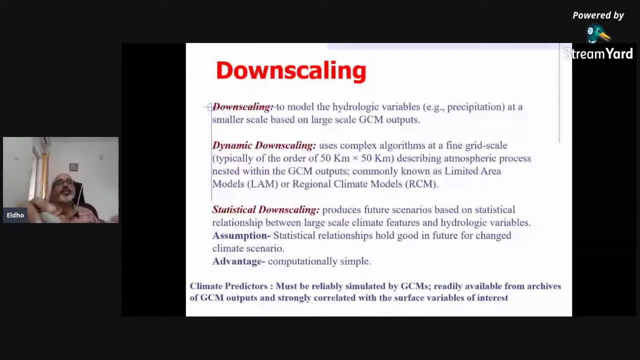 as far as the hydrological assessment is concerned. but the gcm grid is so like a 2.5 degree, like that. so then we need to go for, uh, down scaling. so down scaling, as um you know that there can be two types of downscaling, and second, only the statistical downscale, so, dynamic downscaling, we use complex. 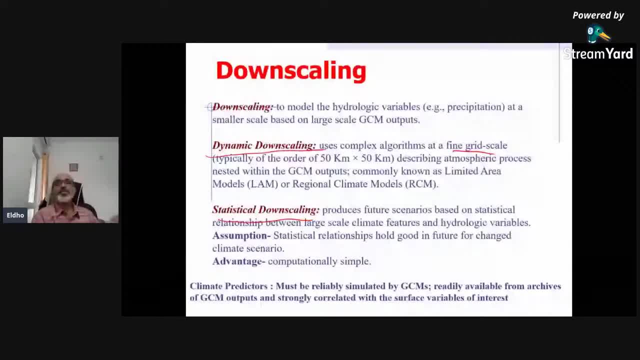 algorithm at a fine grade um scale. uh, so like if you put kilometer by 50 kilo discrete atmosphere process with the gcm output, and then we verify from with the past data, historical data, and then we can go for dynamic downscale. statistical downscale produces future scenario based on. 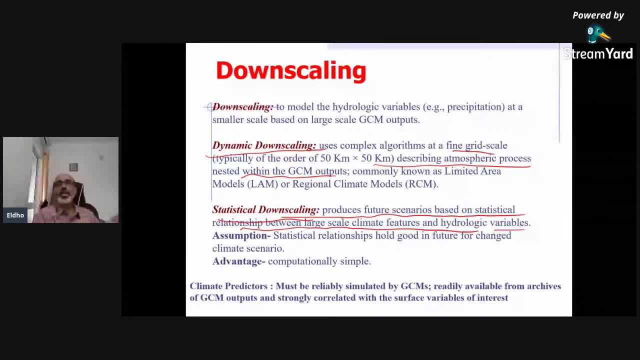 statistical relationship between large scale climate features and hydrological variables, and here we assume that static relationship will hold good in future also. and uh, so this is actually the statistical downscaling since the most preferred, since it is very simple, uh, compared to dynamic downscale, dynamic downscaling: we need to take so many aspects. 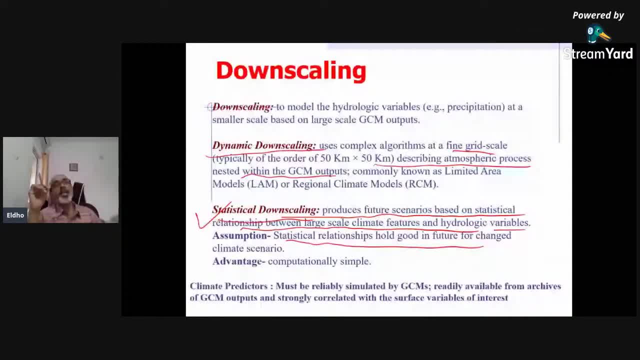 and then we need to put into and then we need to. for a particular region, particular area, we need to get the the details with respect to dynamic downscale, so generally we prefer statistical downscaling. by using the historical data, we can go for the statistical downscaling. 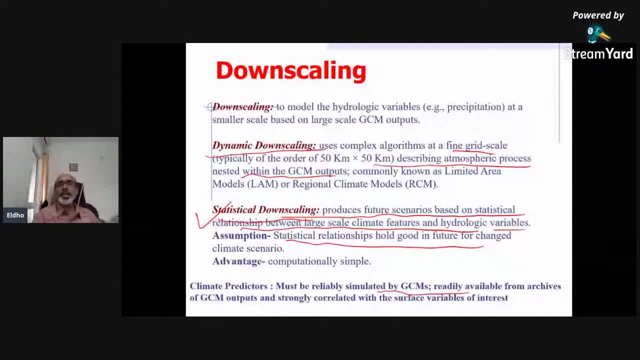 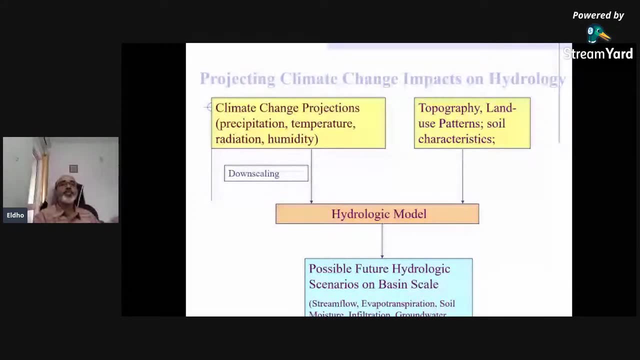 so climate predictors must be reliably simulated by gcm is readily available from our case and then strongly correlated with the various variables like rainfall, temperature and all other parameters. so now coming back to projecting climate change impacts of hydrology. so climate change projection, like precipitation, temperature, radiation, etc. uh, we project and then we are having the data set like a topography. 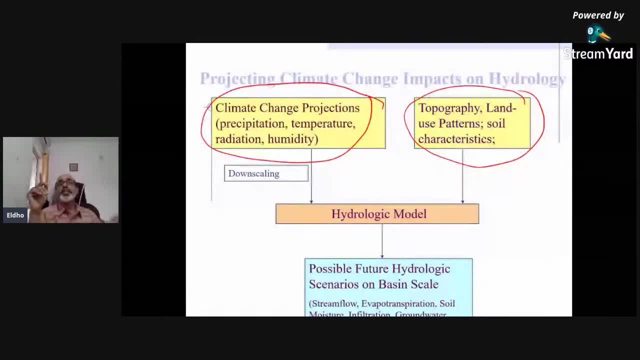 land use patterns, soil characters developing. so that will be the database we need for hydrology. and then these data, the downscaling from the downscaling, this will be coming and that will be coming to the hydrological model, the type of which model you use. that will be coming and then 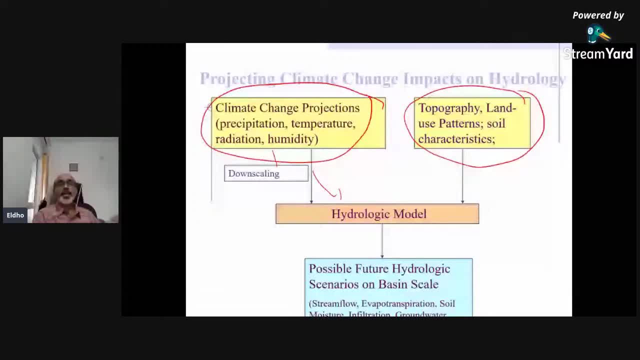 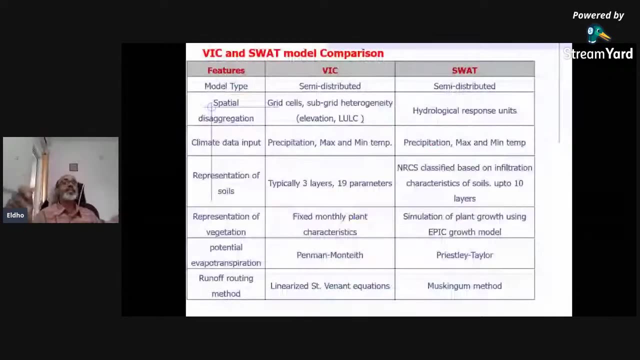 further use the hydraulic model for future hydrological scenarios on basic scale or a particular area, wise. so that is the way we do. we do the uh hydrological modeling with respect to climate change. so generally, as i mentioned, there is a variety of hydrological models are there for the 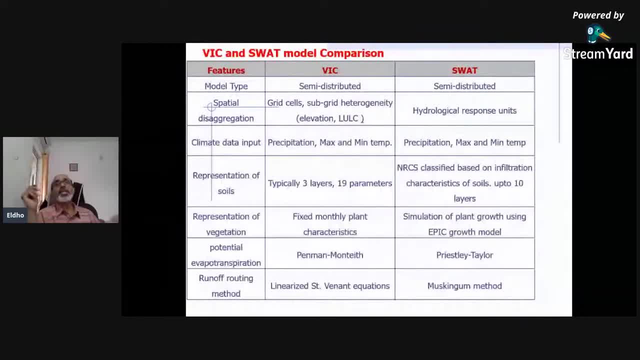 so commonly used one grid device demand for large areas is called a variable infiltration capacity model, vic model, and for river basin scale or even that also used for even for a large scale also it is used. it is a smart model, soil water assessment pool or vic model. so a comparison is given here in 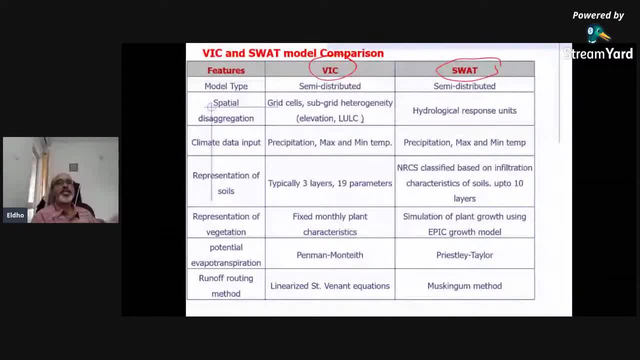 this table. so like a model type. so special disaggregation, um disaggregation like a semi-distributed grid cells: here the grid cells are used here and the hydrological response unit is used. and then climate data input: here precipitation maximum minimum temperature. here precipitation maximum measurement temperature. then representation of 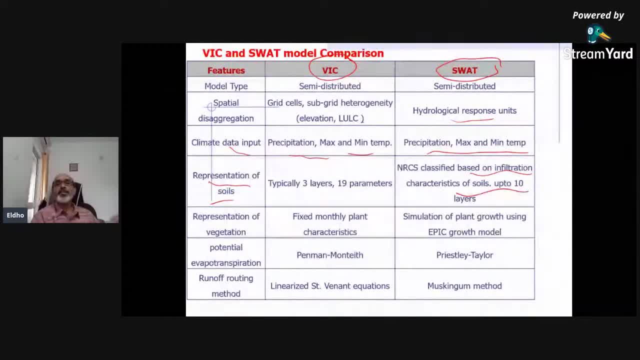 soils typically layer. so here we classified based upon the 10 layers. we can take into then a representation of vegetation pixel monthly plan. so all these aspects, so we can do a vic model or swat model. so here i am going to show some results from one of my behavior using the SWAT model, so that will be. 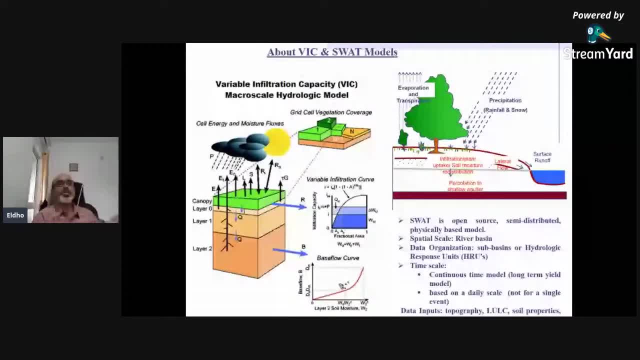 discussed. so here this is what is happening in the vic model, so we will be taking view twice what is happening in a layered model system. so you can see that with respect to the interaction, with respect to rainfall, then then also the evapotranspiration and with respect to infiltration. 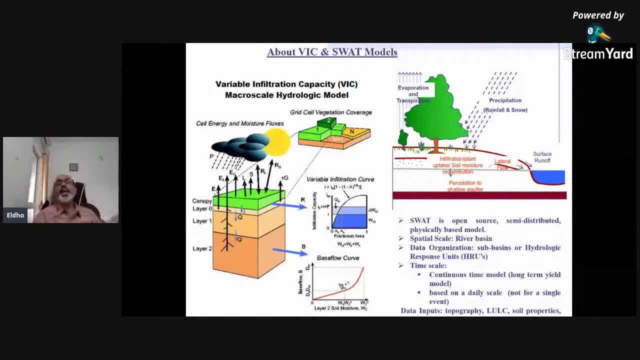 what can happen. so this is the essence of vic model, but in a swat model. so that is an open source model, semi-distributed model, so it is based upon a hydrological response unit and then the time scale: continuous time model is available, based on daily scale also, we can do the simulation and input is topography, land use, land power, soil. 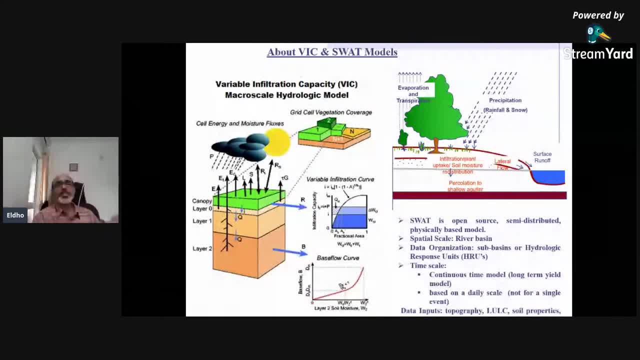 properties, weather and land manual practices. so this is the way the difference between one is a grid based model and another one is a, the hydraulic response unit based model, said heavy based model, so vic and site model. i am going to present here some of the results using 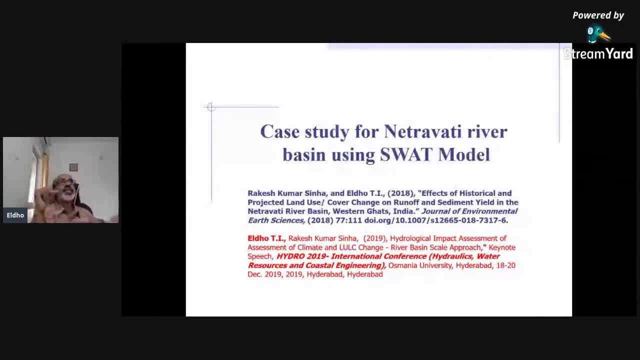 SWAT model. so now i am going to present here a case study. so that is for a river basin, initially, and that is by one of my phd student there, uh, dr ragesh kumar simha. uh, that is for the network. so these days you can see in this publication of environmental science which is already published, to work. 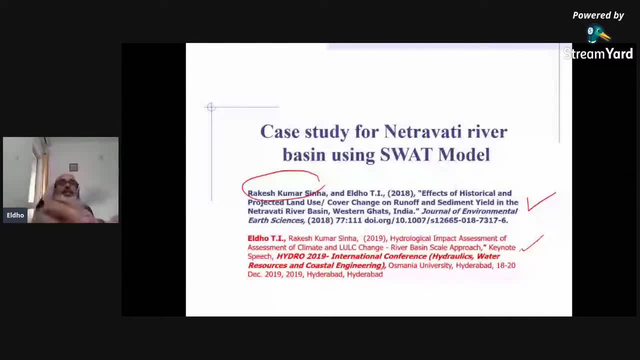 and then this was also present in the conference, and then a few more publication by ragesh kumar simha, you can see, related to these studies. so now the network, your basin, so this is actually. you can see this is located in a karnataka region, so this is in the 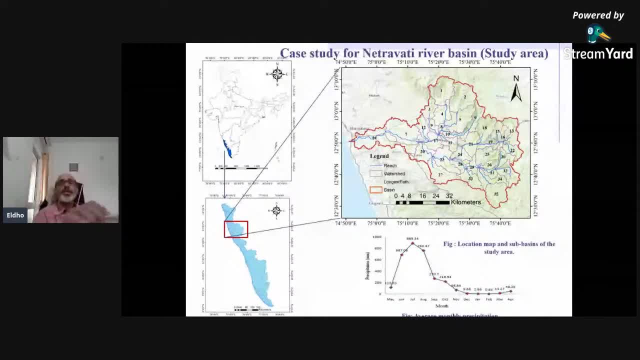 spot of the standards. so this is where the location. so here you can see there. this is the, the, the river basin. so the major river is going to the arabian sea, falling to the arabian sea, and this shows the average monthly precipitation. so, being western guards, the rainfall is around 3000. 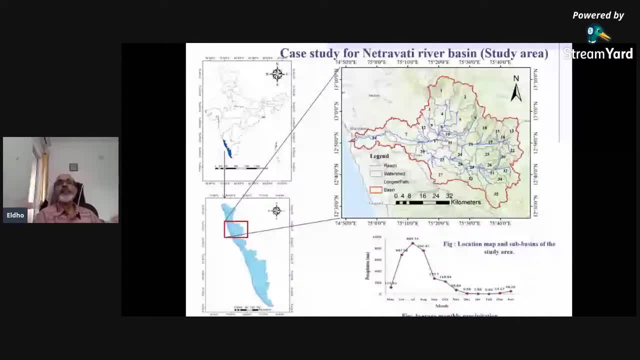 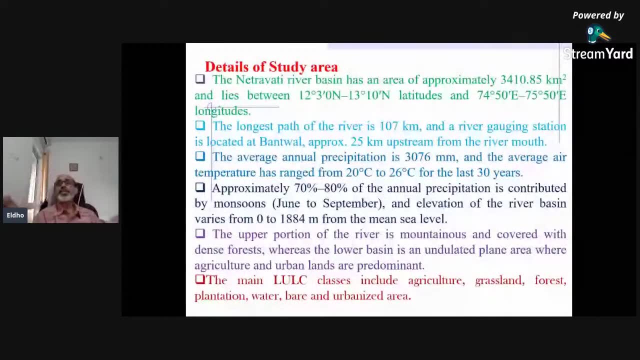 millimeter per year high rainfall area and the western parts of india, so that other river basin has an approximate area of 3410 square kilometer. and then the longest path of river is about 107 kilometer and approximately there is only one weight station, which is by controlled by central water commission. 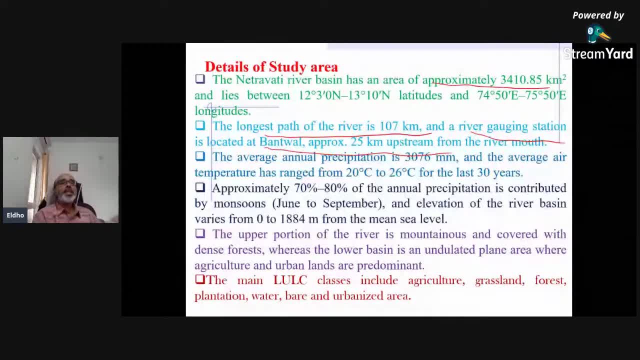 of india and the 25 kilometer stream on the river mouth. the average annual precipitation is around 3000 millimeter, and then the temperature is varying from 20 degree to 26 degree. approximately uh 70 to 80 percent of the annual precipitation is during the mud zone season, june to september. 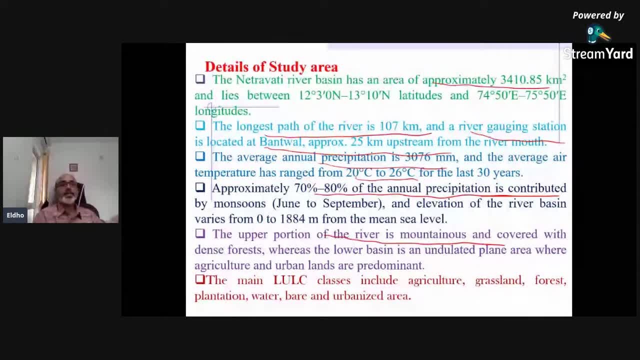 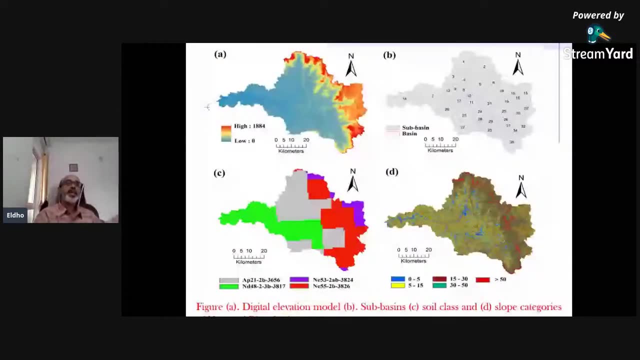 and the upper portion of the river is mountainous and then covered with that forest and the main land use. land classes include agriculture, grassland, forest plantation, etc. so here you can see various aspects. so this is this figure shows the little elevation. uh, this is the dm you can see. 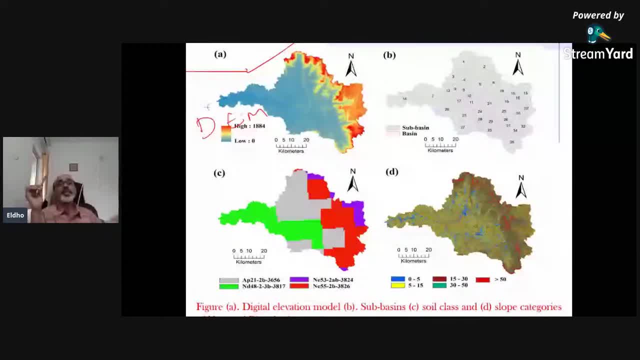 that the, the, the height is varying from 1800 meter to almost uh, the c, that's zero. and then this shows the right soil type in the third basin which we use in the sword modeling, and this figure, see, shows the soil class, various soil class, which we consider this river basin and this shows the. 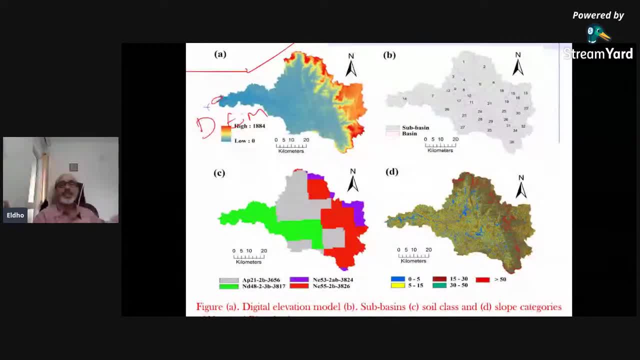 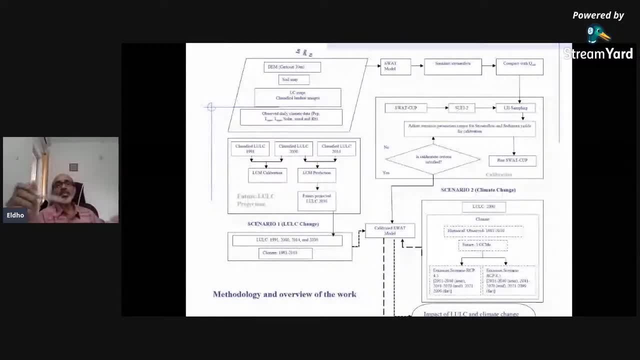 slope categories and with respect to the. well, we considering the uh modeling. so these are some of the results derived as far as the studies get sent, and this is the methodology which was developed by dr ashcal maxinha. so here you can see. um we start with the, the um, the uh pigs for the garden. 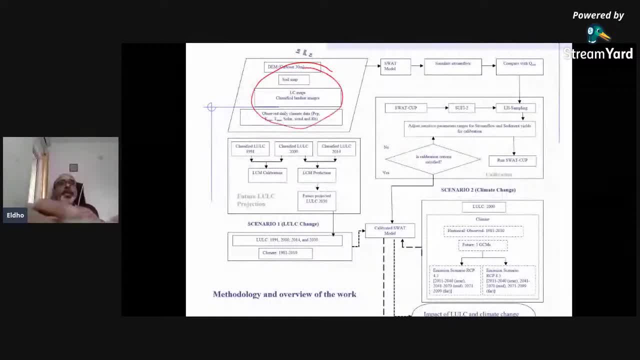 DEM, then soil map and then daily rainfall, and then we identify the land use, land cover for the past, land cover, land use- and then also we go for projection of the LULC till 2030 or even later- he has done up to 2100 also, that is with respect to LULC- and then 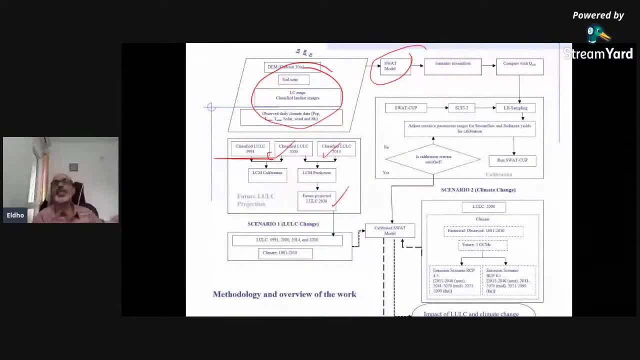 SWAT model is here, and then we try to simulate stream flow and then compare with the runoff measured runoff. So SWAT cup is used for the using Suki algorithm, we use for the parameter of the SWAT model and then, once it is calibrated, so, climate change is concerned, the LULC 2000 is considered. 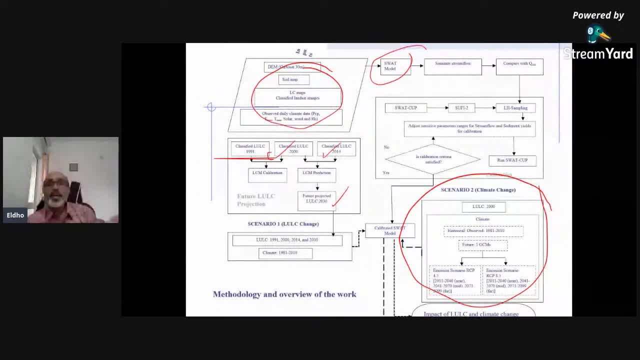 to assess the climate change- historical climate change- And then we used to hear 5 GCMs. emission scenarios are RCP 4.5 and 4.8.5 is shown here. So these are the scenarios which are simulated using this in the study. 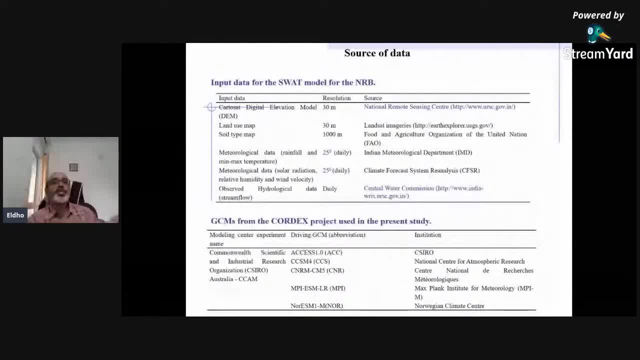 So some of the input data for the SWAT model so you show here, input data like DEM is obtained from national remote sensing center and then land use map about 30 meter resolution extracted from Landsat, So all type data is obtained from it. 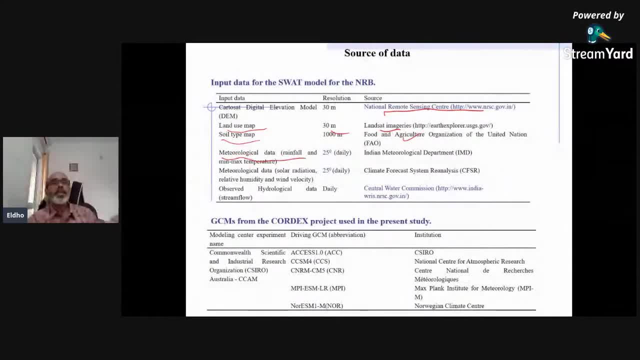 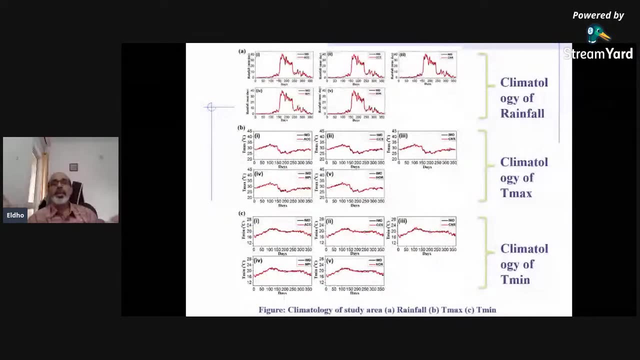 Okay, Meteorological data, IMD, all those things are shown here and here it is. he has used the context GCM data, So the details of the GCMs used are also shown here. So now say we did the assessment, climatology of the study areas assessed with respect to 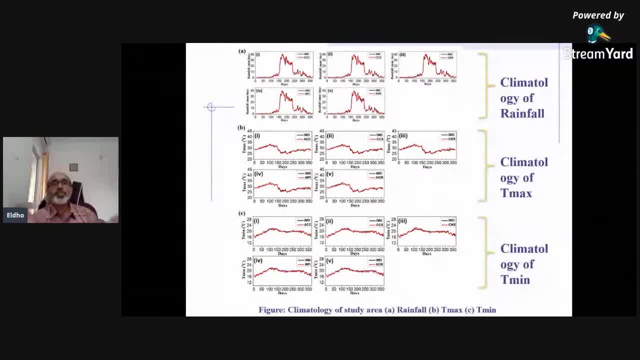 rainfall. maximum temperature: minimum temperature. So this shows, with respect to, say, past 30 years, the various conditions are assessed. So we can see that this is the data. So we can see that this is the data. Okay, 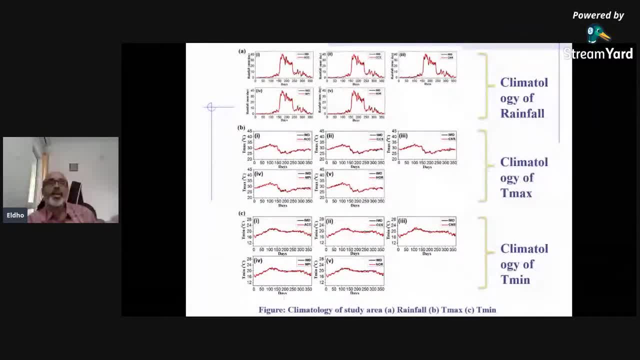 So this is the data that was assessed and then also by using the various 5 GCMs which he mentioned, that also assessed. So this shows the climatology of rainfall and T max and T minimum. So this way we can do the typical assessment and this show the diagram for rainfall T. 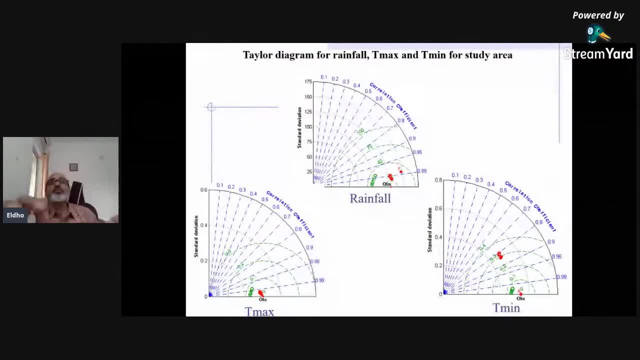 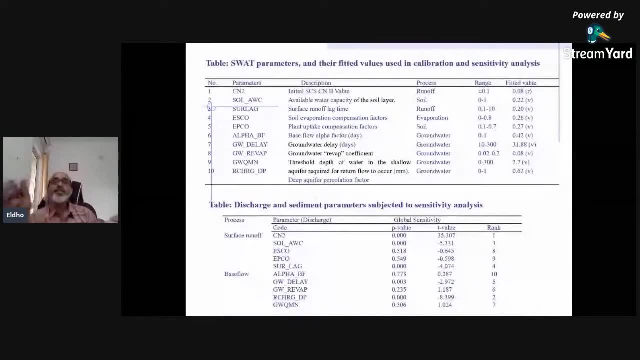 max and T minimum. So with respect to the IMD dataset, the comparison was done and then we got satisfied results. And then the SWAT parameters. where is important? there is about 30 to 35 meters of index value, So we can see that. 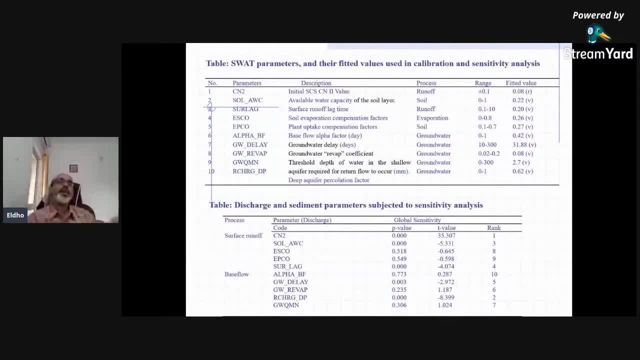 is about 32 parameters are there after that from the leaflet, and we have these 10 parameters as the most important parameters as far as the runoff prediction is concerned, and then sedimentation is also done. so these are the important parameters as far as the sedimentation is concerned. so these 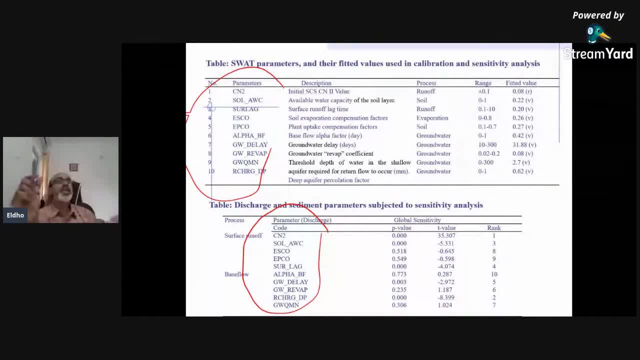 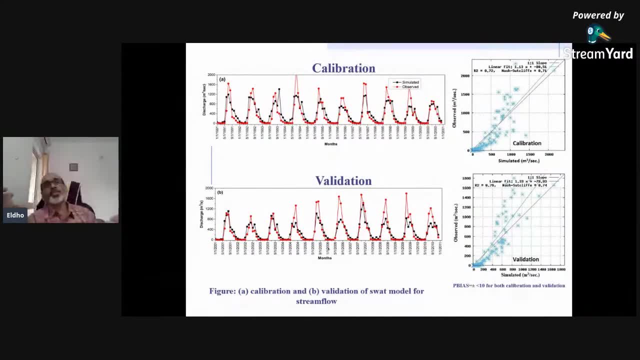 are all. generally, those are using SOAD model. this is the standard procedure which we adopt. so then, of course, since we are using the SOAD model, we need to do calibration, since a number of parameters are there. calibration validation, since when we obtain the satisfactory calibration, then it was validated. the model was validated using those parameters. so you can see that some 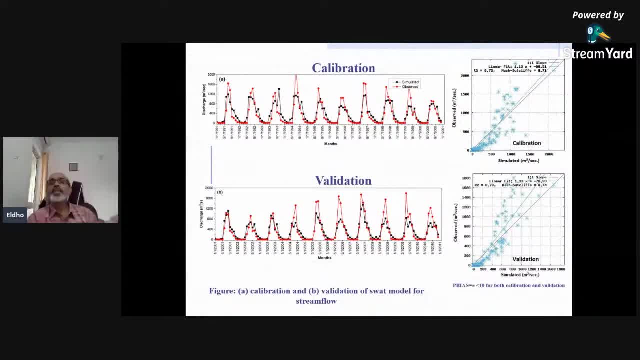 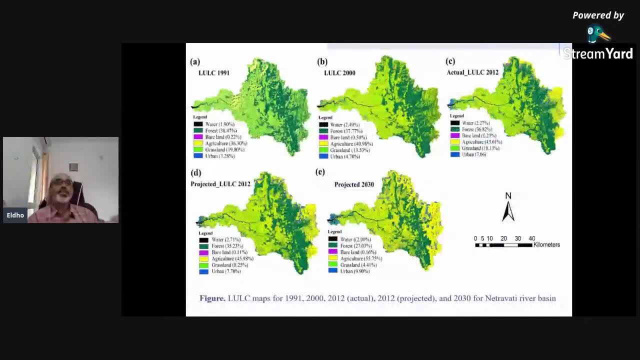 reasonable, say NARSAC-LIFI coefficient about 0.71, that is obtained. so that way calibration and validation is done as far as this model is concerned. so then you can see. this slide shows the land use, land cover, say, for example, 99 leaflet. 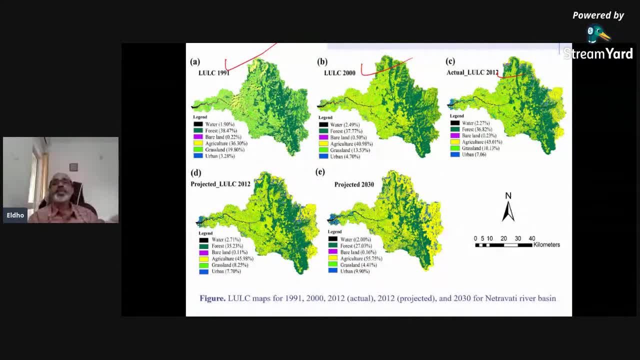 0.71, 2000, 2012, and then he projected for the 2012 using the actual land and then compared the projected and the land change model. LCM is used for projection. so this shows me for 2030 and formerly projected up to 2100 also, but here I presented only for until 2030 and this 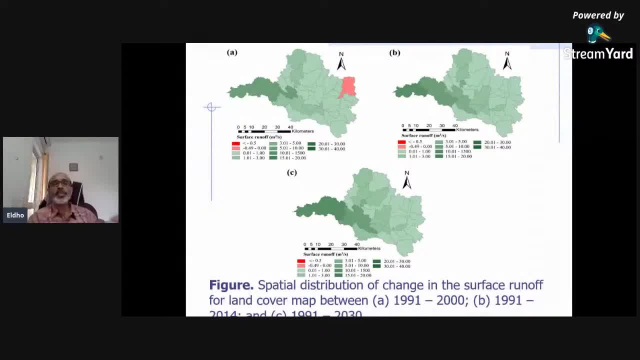 shows spatial distributional change in the surface runoff for a land cover map between 1991 to 2000. bigger a and then is for 1991 to 2014 and then it shows with respect to 1991 to 2030. so you can see that. 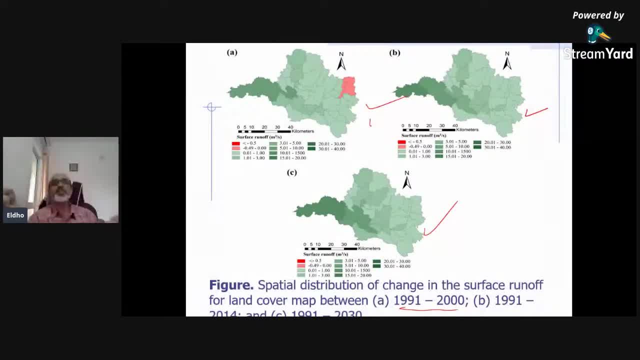 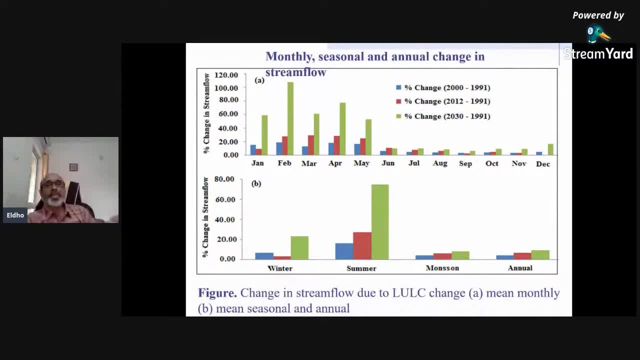 a large scale variations you can observe in these figures. and then also we assess the monthly, season and annual change with respect to stream flow changes- streamflow due to land use land cover change. so initially a change with respect to land use land cover change is assessed. so 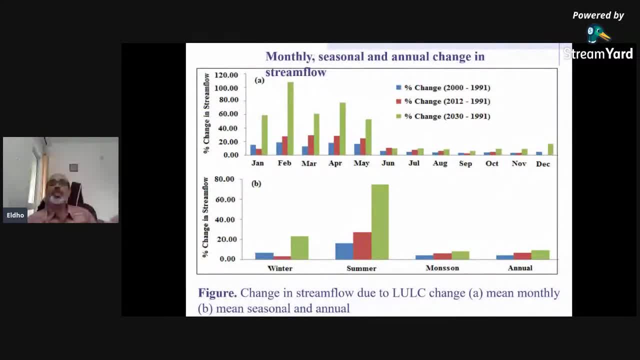 present day change is shown here, like in 2002 with respect to 1991, 2012 with the respect to 2003, and then we assess the change with respect to the end year, the change with respect to the total time period of the year, since I told you the fact that the range of the duration of the 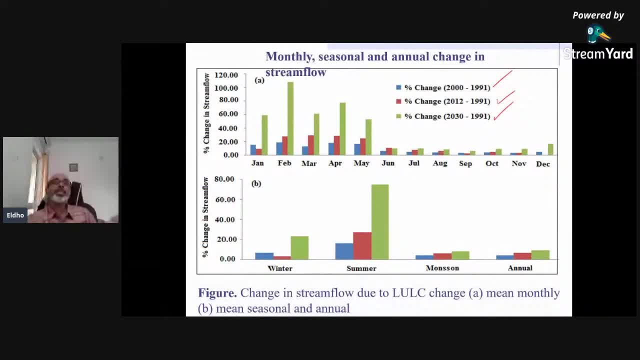 You can see this keep on increasing the changes. that means the land use, land cover is drastically changing And then correspondingly you can see also season-wise, also winter, summer, monsoon- all these changes, especially this region, summer changes will be severe. 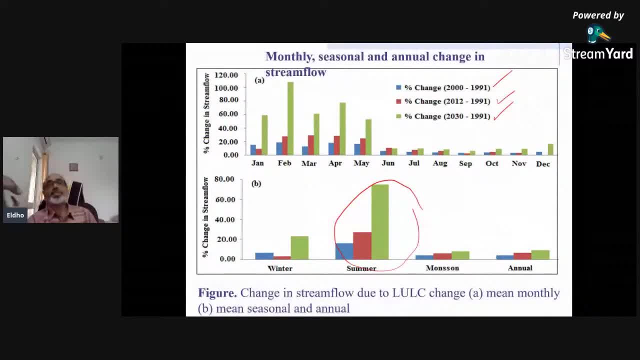 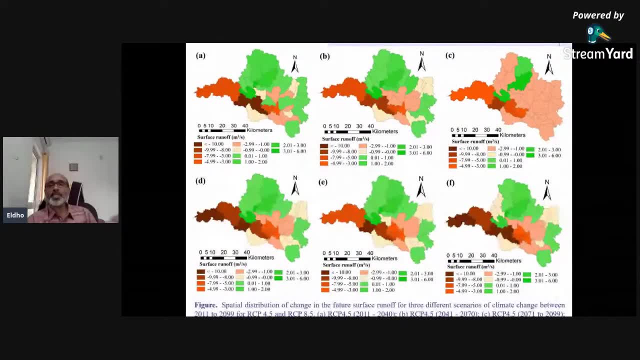 So that is what is shown, the historical as well as the projected, And this shows the spatial distributional change in the future surface runoff for three different scenarios of climate change between 2011 to 2099, for RCP 4.5 and 8.5.. 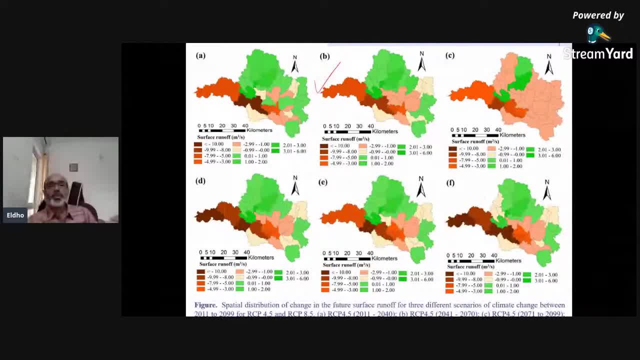 So, first figure: this figure shows RCP 4.5 between 2011 to 2040, the near future. And figure B shows: this figure shows the changes with respect to 2041 to 2070.. And this C shows 2071 to 2029.. 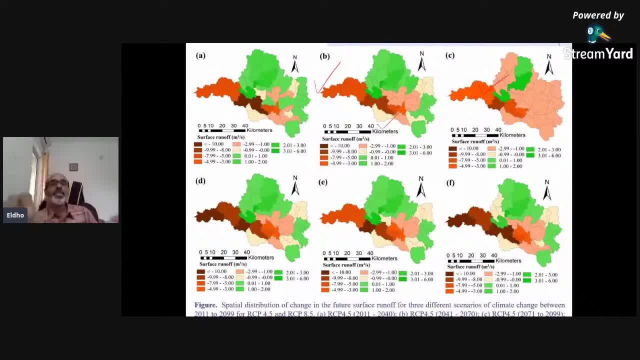 So near future, mid future and far future, what is the impact? So you can see that This is always. there is a huge change. you can see it is minus. it is many places, though the rainfall is increasing. many places are decreasing as far as surface runoff is concerned. 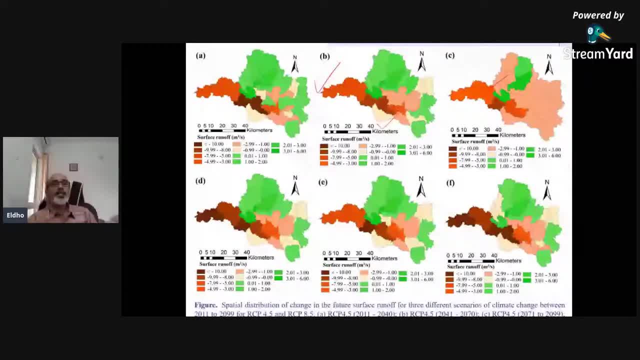 You can see the total impact. you can see. So, similarly, this figure shows the near future, mid future and the long future up to 2100.. So here for long future, all these things we used in 2013,. and land use- land cover. 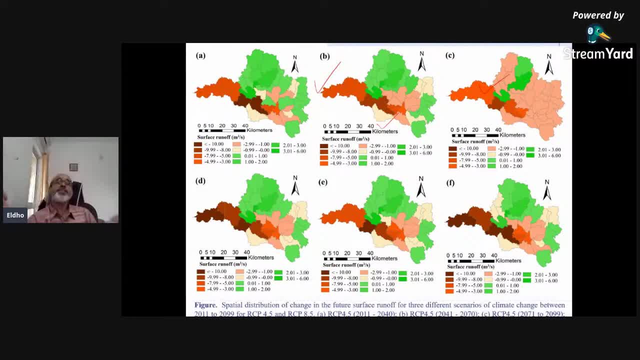 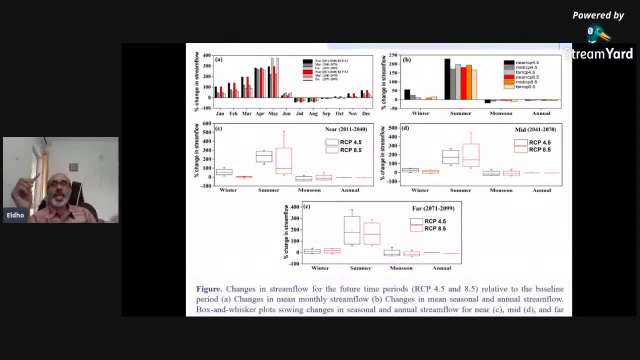 use whatever is considered, And then the impacts is quite visible you can see. So that way we can do this kind of assessment and this figure shows changing streamflow for the future time periods with respect to RCP 4.5 and 8.5.. 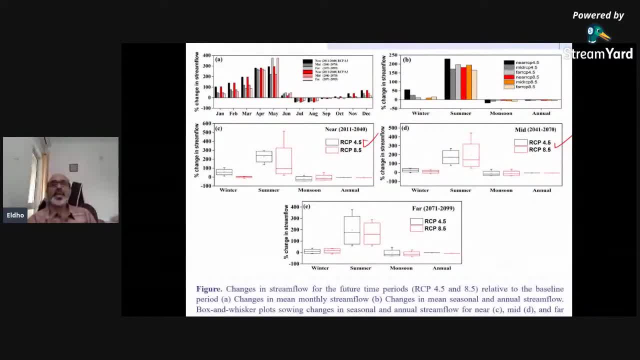 So this is related to RCP 4.5 and 8.5.. For the near future, mid future and the far future. So, with respect to lead you to baseline period, it is: baseline period is up to 2011,. the change: 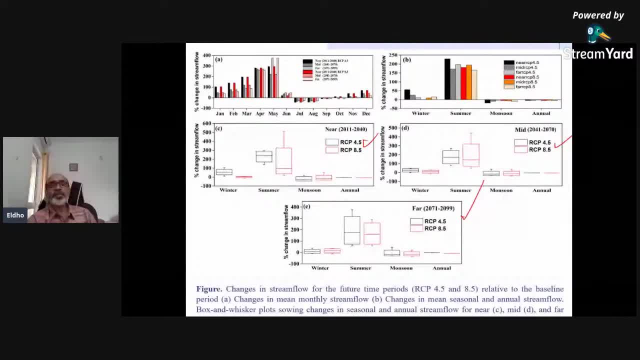 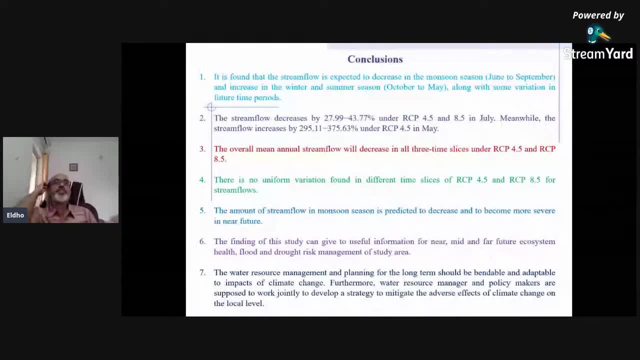 in mean monthly streamflow Change in the year in the year, So that this figure shows mean seasonal annual stream flow, so that way we can see what are the impacts taking place. so for some conclusions from this study, it is found that stream flow is expected to decrease. 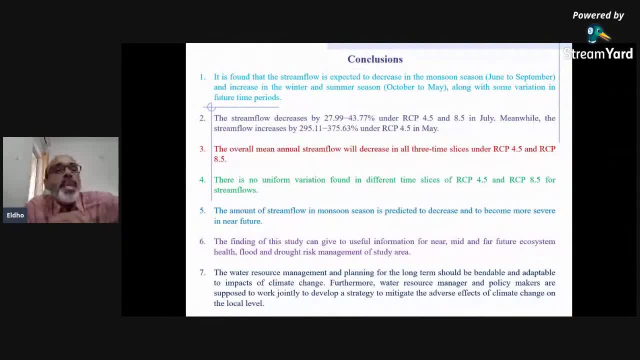 in the monsoon season and increase in winter and summer season. the stream flow decreases by around, say, around 30 percent or 35 percent under rcp 4.5 scenario and rcp 8.5 scenario, in july this 37 to 43 and then the overall mean annual stream flow will decrease. 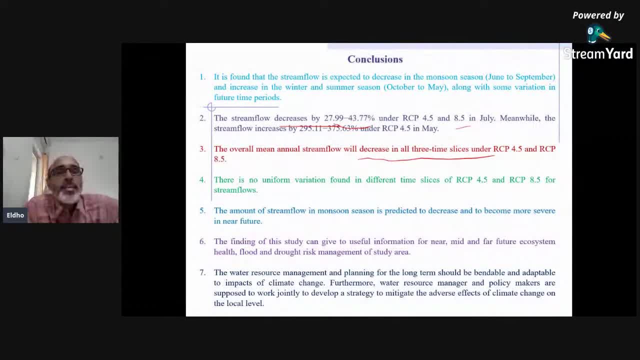 in all three time slices: rcp 4.5, 8.5. there is no uniform variation on in different time slices and the amount of stream flow in monsoon season is predicted to decrease and to become more severe in near future, and finding out the study can give up useful information for near and mid future. so 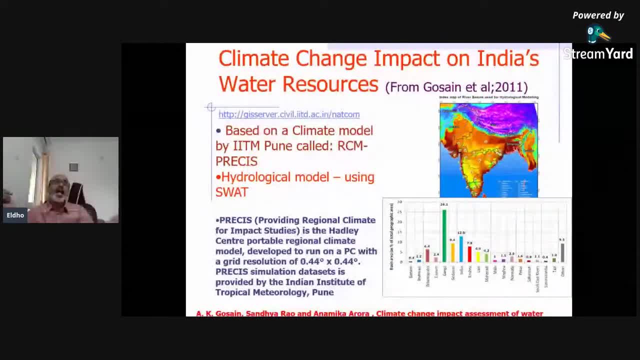 that way a river basin scale assessment we can do. and before closing few slides, i should just say that the stream flow is expected to decrease in the monsoon season. So this study I have taken from Professor Gosain, who has done for the entire country, for the entire India. his team used ILTM based RCM- precise climate change model is used, and then again he also used the SOAD model. 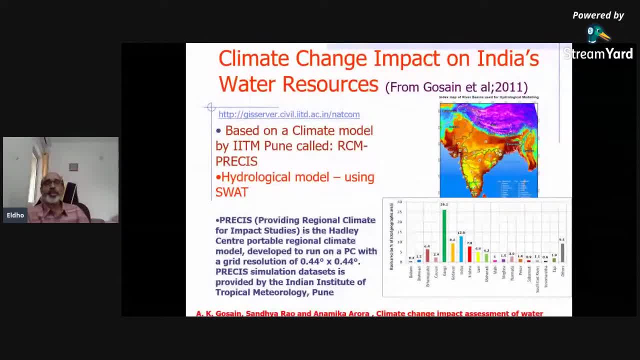 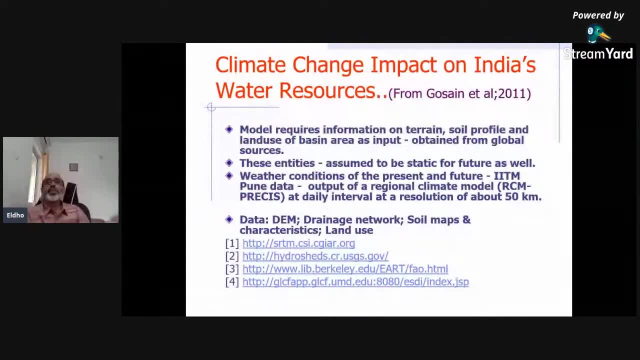 So precise climate change model is used and this is available in current science, the details are available. So various river basin scale changes have been shot. So model information, terrain, all those things- SOAD model- we have already seen. So this data is very similar to what we have seen in the previous case. So that is climate change impact for the entire water resource. 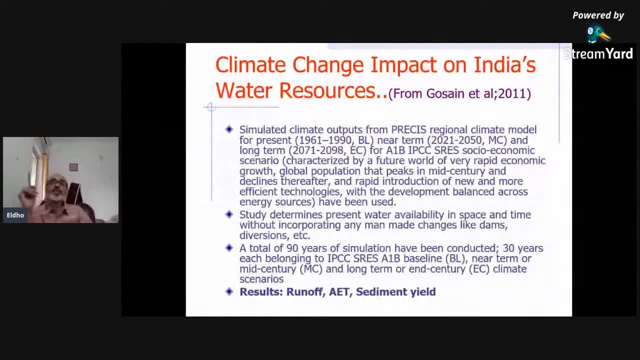 So the simulated climate change is very similar to what I have discussed for the natural river basin here, also Near future, like the historical and the near future, 21 to 50,, mid future and 21 to 50 and the near future and 71 to 98.. So, like that, various scenarios were projected and study determined the present waterway between space and time and total of 90 years of simulation was done and this is now published work all of you can refer. and he has estimated runoff, AET, evapotranspiration and sedimentation. 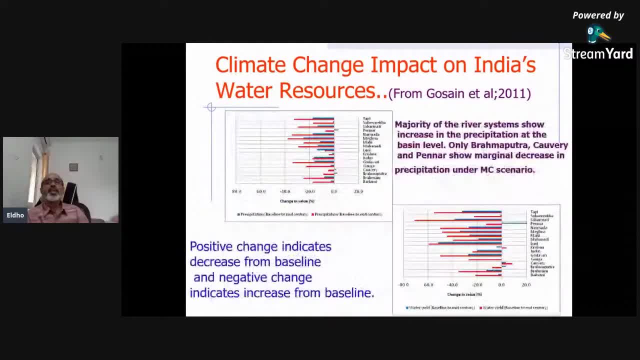 So I will just project some of these results given in this paper. So here, a possibility change indicates decrease from baseline. So this is the baseline, so this is the baseline and this shows possibility change shows a decrease from baseline and negative change indicates increase from baseline. 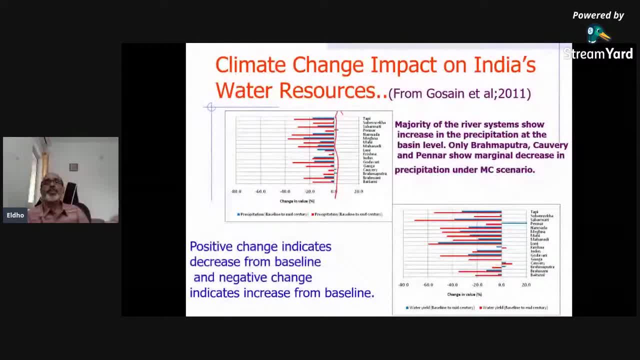 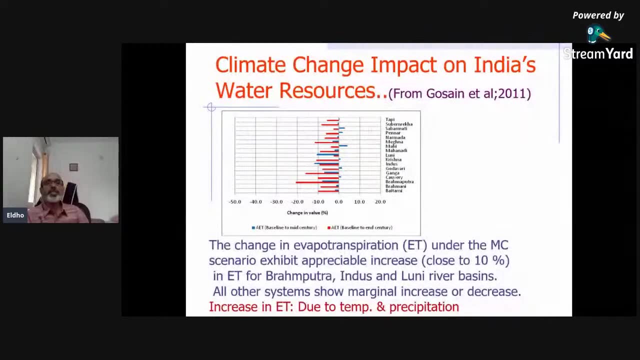 So many other river basin, it has decreased. majority of the river basin system shows increase in precipitation at the basin levels. Only Brahmaputra and Kaveri and Perna show margin decrease in precipitation under mid-century scenario And then change in evapotranspiration under mid-century scenario. excavator appreciably. 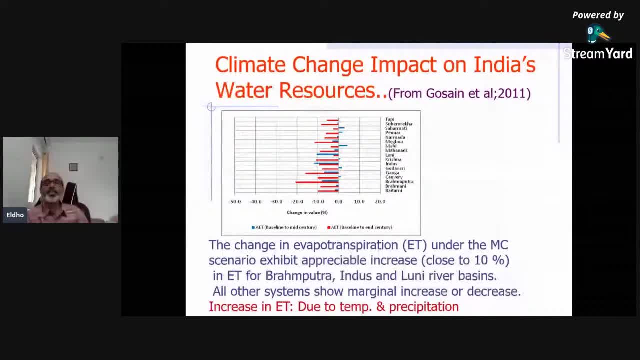 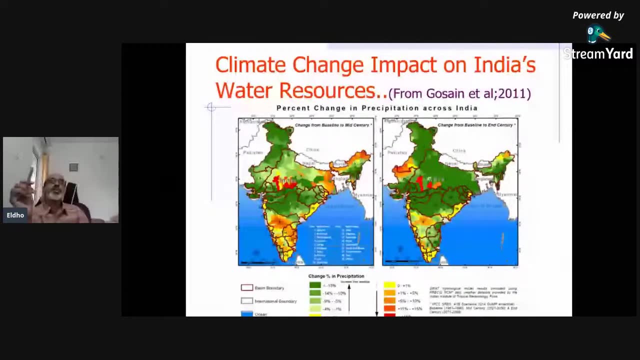 increase in evapotranspiration in Brahmaputra, Indus and Uni river basins and increase in ETs due to temperature and precipitation. So this shows climate change impact with respect to various river basin. So then, this shows few slides and just to completely finish it off, 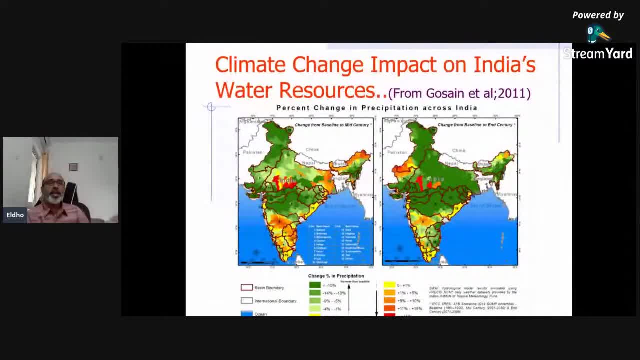 So percent change in precipitation across India. So you can see that this color shows the increase in French and this red and other colors shows decrease in French. Most of the places it is shown that, with respect to this study, the change in precipitation is increasing and a few places it is decreasing. 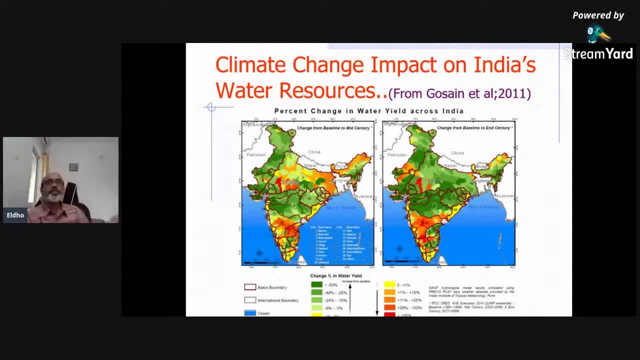 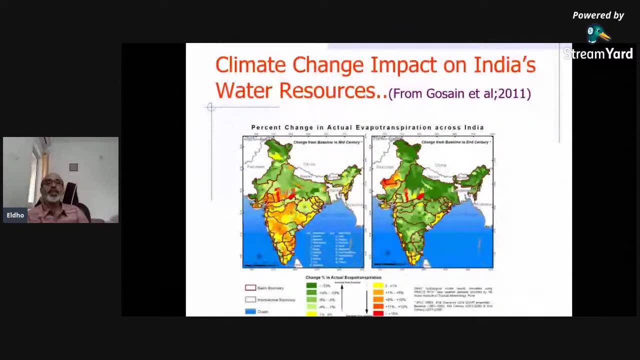 And then automatically you can see the percentage in water yield also. In places water yield is increasing and some places like this, Maharashtra, Telangana or this region, it is a decrease- in French is shown And then correspondingly, since the temperature is increasing, actually evapotranspiration also. 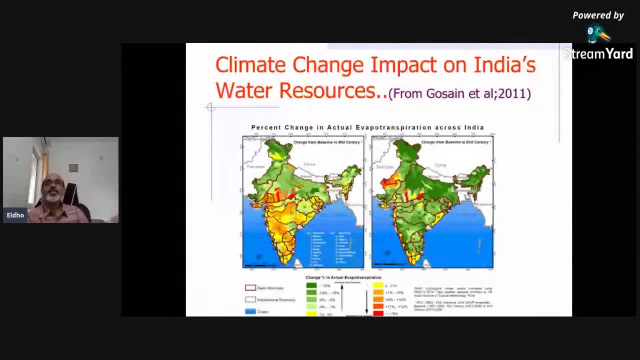 you can see that most of the places is keep on increasing. So this is change from baseline to end-century. So this is change from baseline to mid-century. So, mid-century, when we come to the end-century, 2100, it will be, the changes will be drastic. 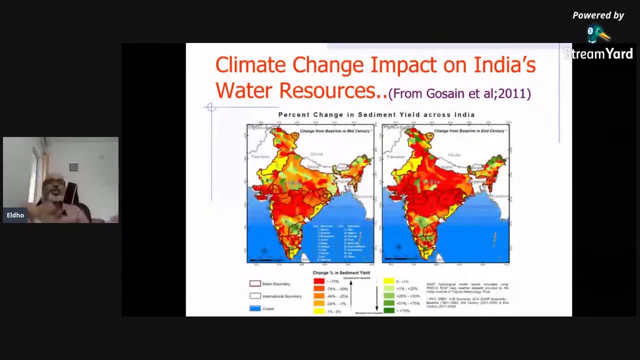 due to the increasing temperature. So now there will be scenario. So that way I mean corresponding to even RCP 4.5, currently what we are using. that means that the same trend continues. what will be impacts? So then of course the, since the rainfall is increasing and then also the runoff is increasing. 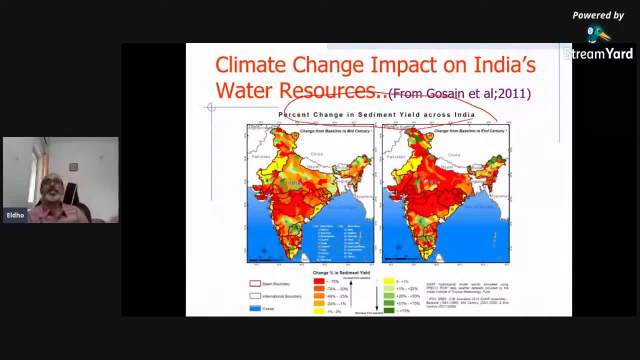 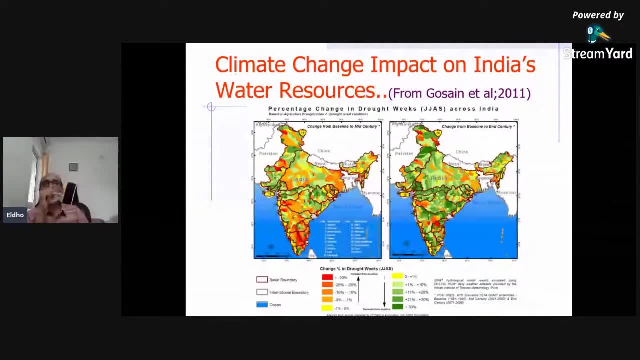 definitely sediment need across India is increasing. So you can see there is an increase in trend in most of the places. So that is what is observed here. So similarly drought needs. So obviously the drought also, drought conditions also will be increasing. So that is what is shown here. 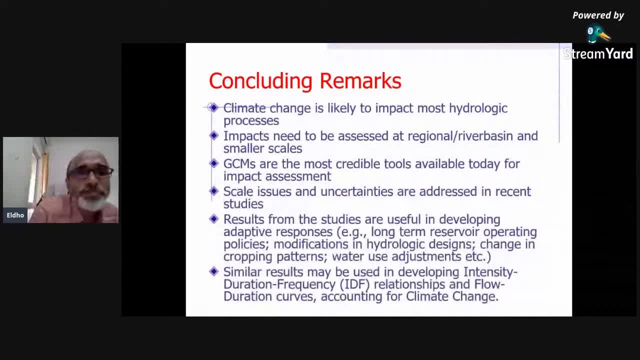 So now, finally, to conclude this study, conclude this discussion, Thank you. So climate change is, as I already mentioned, there is a huge impact is there on the hydrology, So impacts need to be assessed at regional and river basin scale, small scale, 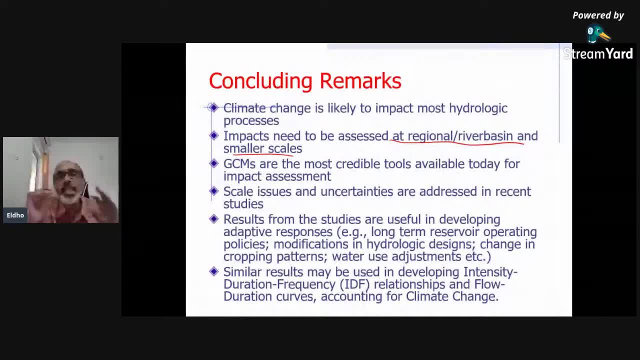 So when we say GCM or the total large scale is concerned, it is from that we need to come to a smaller scale, the river basin scale, regional scale- And of course we are currently also we are using GCM- is the most credible tools. 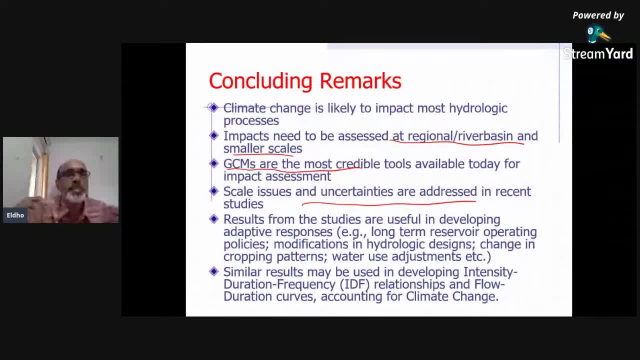 So scale issues and uncertainties, lot of uncertainties. you can see which GCM we are using, What kind of data you are using. everywhere uncertainties are there. So including model uncertainties are possible that all we need to account in these kinds of studies. 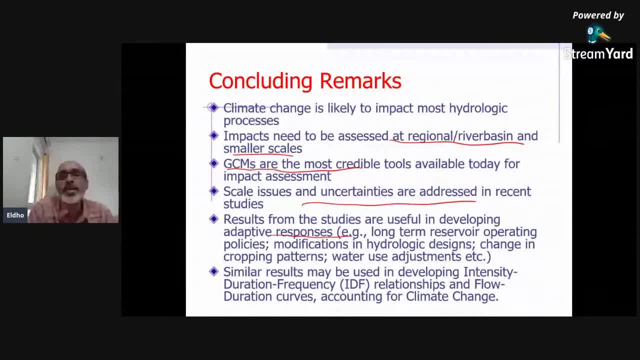 So research from the studies are useful in developing adaptive responses like long term reservoir operating policies, modifications, regulation design, change in cropping pattern, etc. And similar results may be used in developing idea of care for further flow duration care and accounting for climate change. 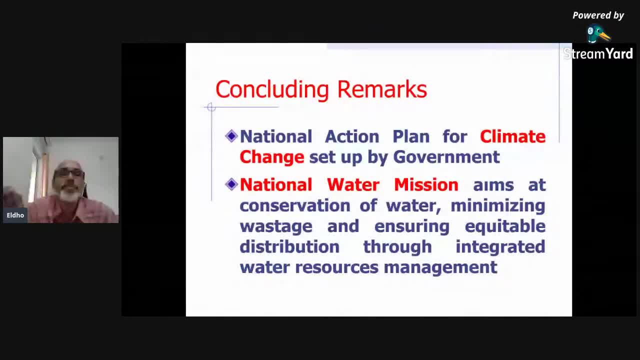 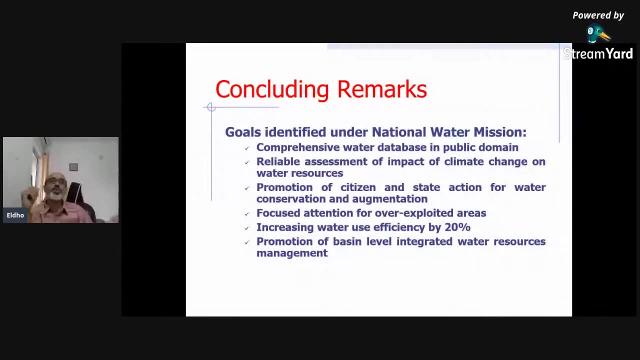 So in India, National Action Plan for Climate Change is set up by Government of India and water machine is also there. it aims in conversion, conservation of water, minimizing wastage, ensuring equitable distribution, etc. so some of the important goals identified under this national water machine include competency, water database in public domain. so so much of work is happening. 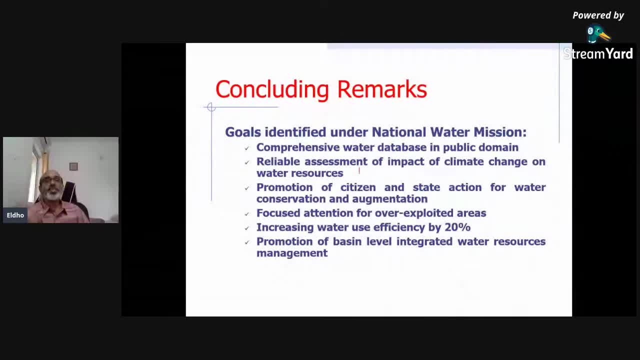 and reliable assessment of impact climate change on water source. so this is: we need to do the assessment for the entire country and then also we need to do river basin scale assessment. the promotional citizen and state action for water conservation organization focused attention for over exploited areas, increasing water use efficiency, etc. we need to look into so that way. 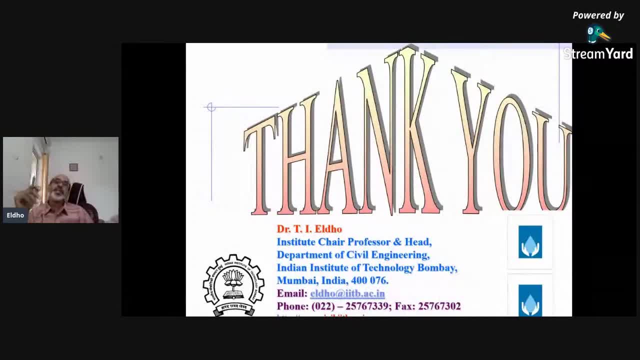 the climate change, as far as we can see that there is a huge impact on hydrology, so that we need to assess it properly. so it is not only for the country we need to assess for the, the river basin scale also, so that we we can have a reliable understanding. 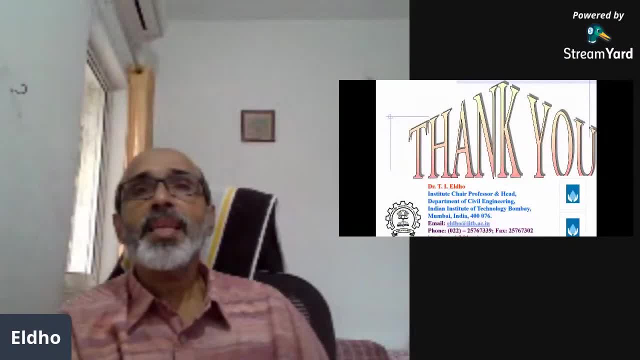 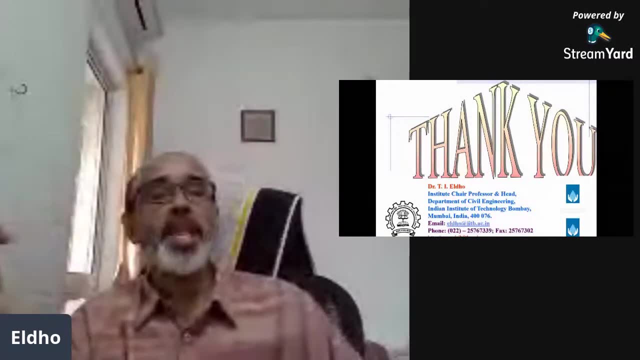 of what is uh presently happening and what is going to happen in future. either it will be until 2030, 2050 or 2100 in future. also, we need to assess it the the climate change impacts on hydrology. so that way, we need to look into all these aspects and then- and we have to- 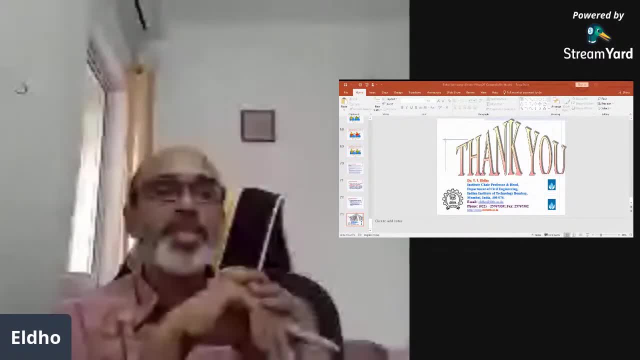 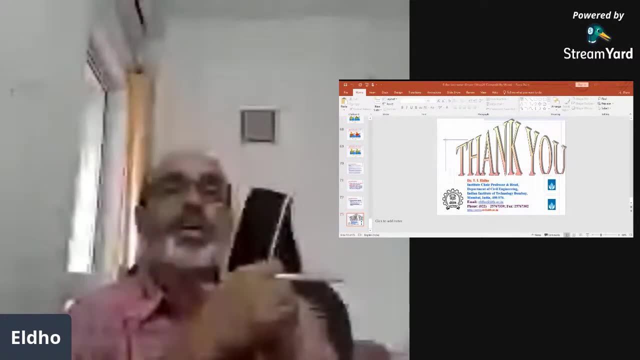 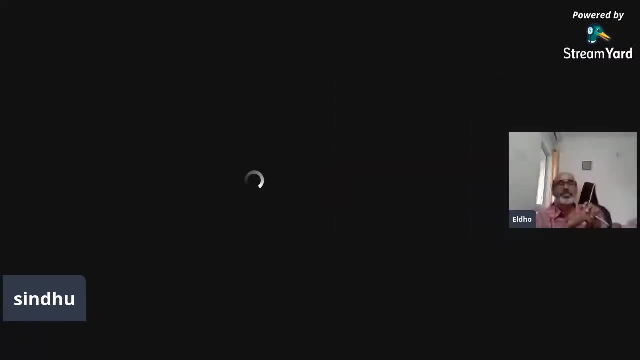 say, assess the climate change impact as far as hydrology is concerned, on a river basin scale or for the entire country's concern. so with these i stop here. uh, so you know what all questions are there. now i'll be happy to answer the possible. thank you very much. thank you, professor, for the presentation. 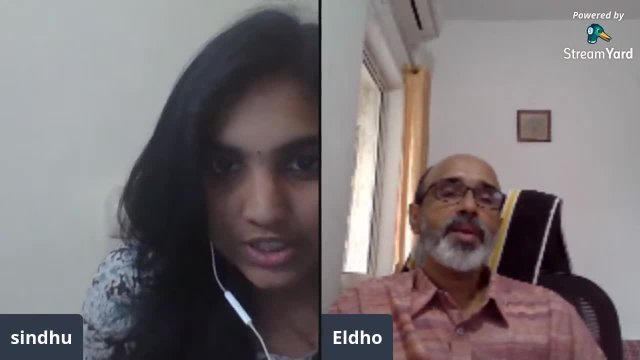 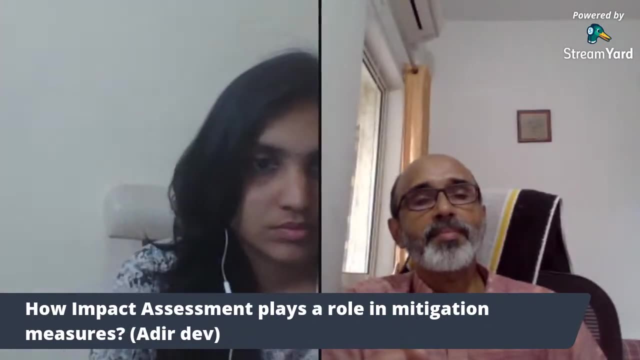 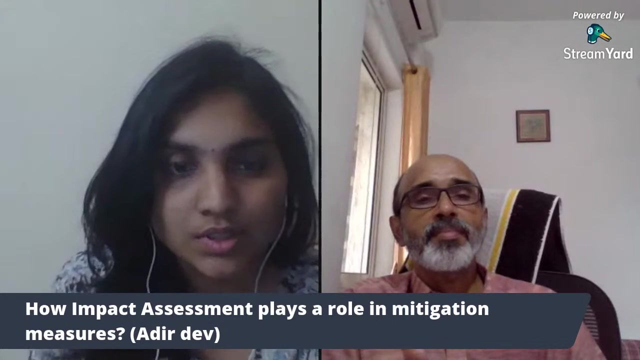 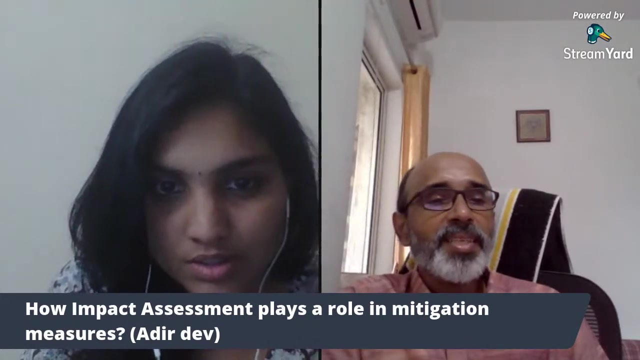 uh, we have received few questions from the viewers. shall we display it on the screen for you? yes, please, so can you see the question? you are in the show. everyone can see and hear you. that is what is coming. how impact that doesn't play a role in mitigation machines. 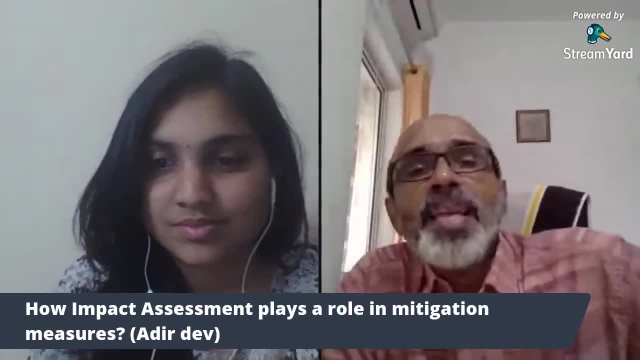 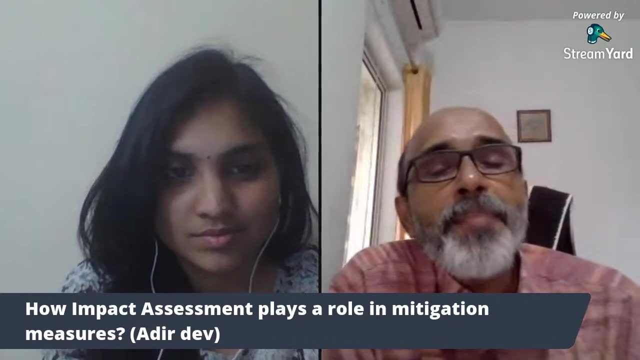 so in fact. so you see that mitigation measures are concerned, for example agriculture is concerned, or the, the power production using the hydroelectric power projects are also all concerned. so you can see that um, For example, in the common trend. say, for example, if you take Kodavari River Basin, 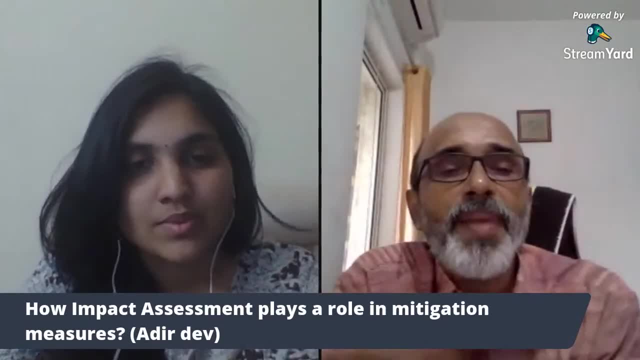 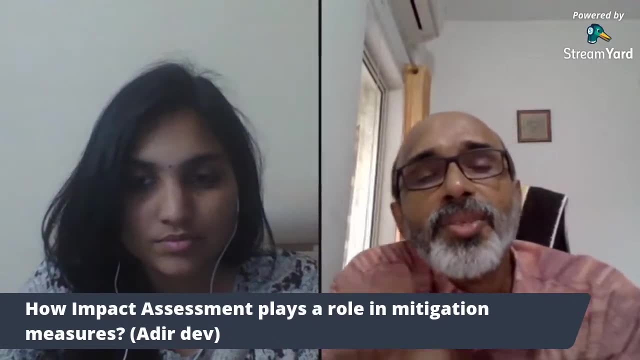 or a particular river basin is concerned, what is happening in the systematic way: the past, what has happened, and then in the coming future, future decays, what is going to happen if you look into that, So then we can come with the planning, like mitigation measures, like how to do the water. 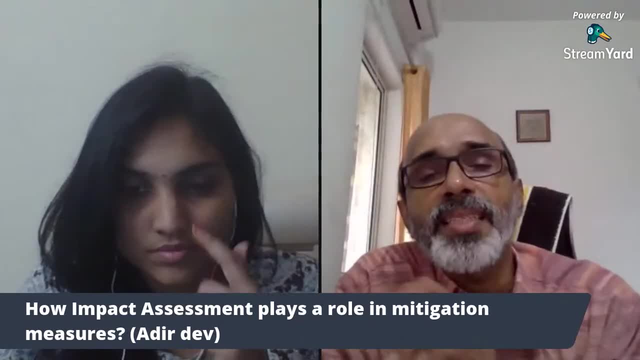 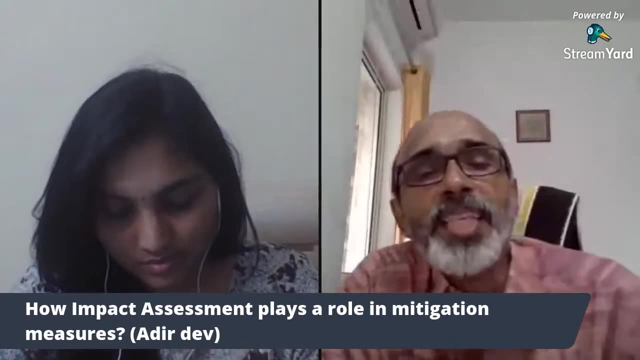 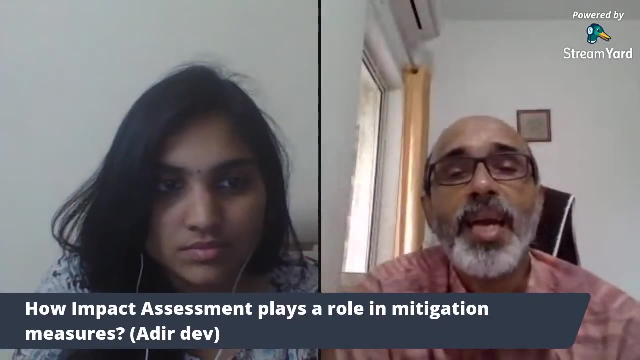 allocation policies. The policies can change, So how much water is to be allocated for a particular sector or a particular region? all this can be done, And then especially severe impacts is concerned, like flooding or droughts are concerned. So that way also we can look for further, say for example the land use, land cover, 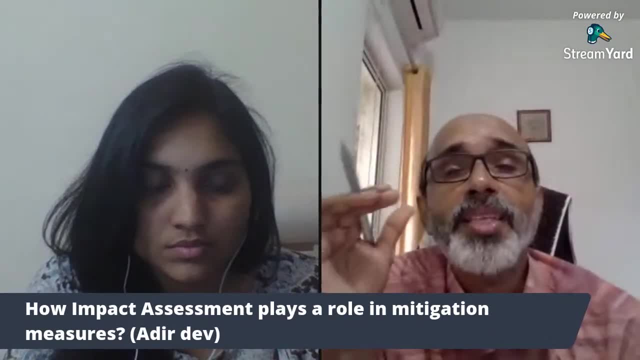 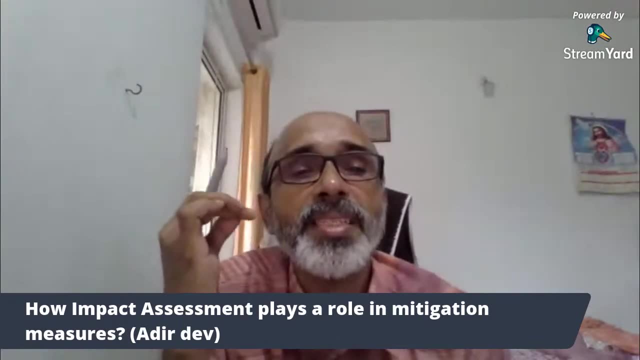 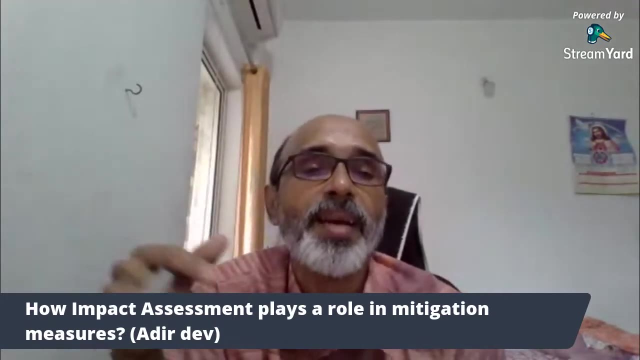 change. we can put some control over that so that there is no further development on the flood plain or the rivers. So that kind of things we can put it so that the mitigation measures directly is possible by considering the hydraulic impact assessment. So that way, the near future or mid future or far future, say till 2100, this kind of 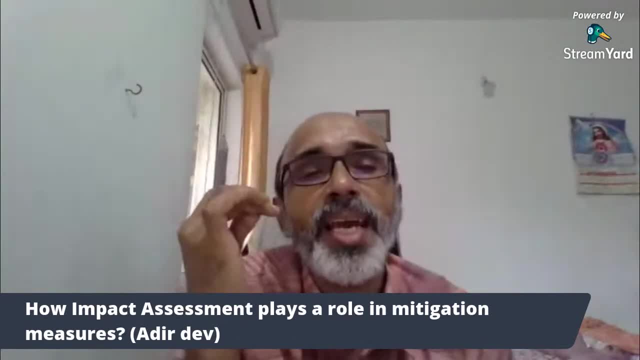 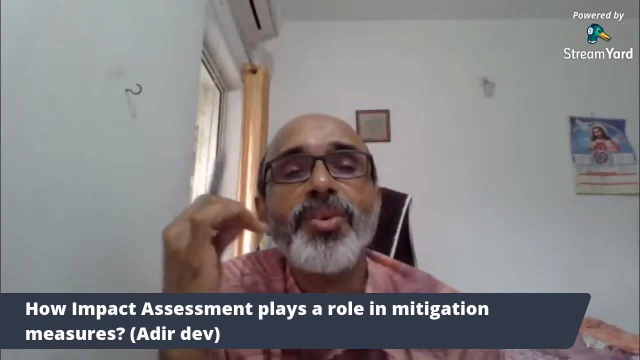 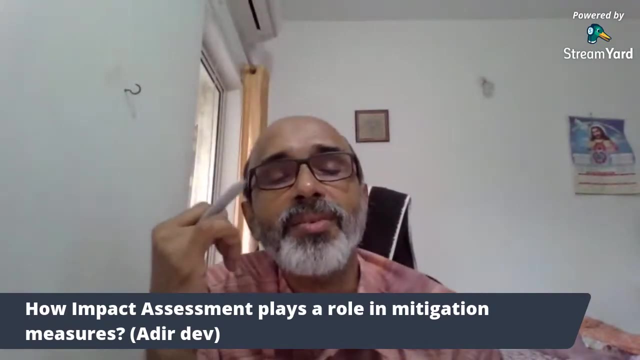 assessment is possible. So this kind of assessment can be definitely put in our policies so that the impacts can be, the mitigation measures can be taken by the decision makers, So we can have a long time planning. Planning is concerned with respect to the water utilization, efficiency in water utilization. 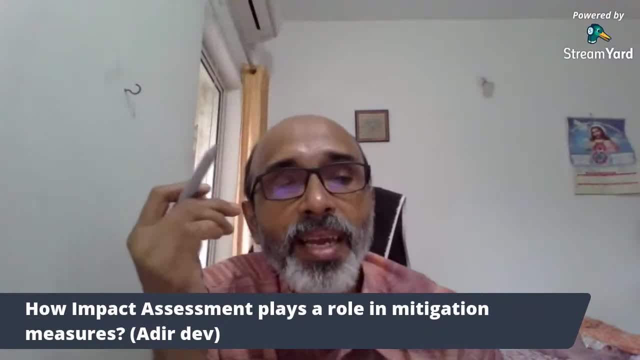 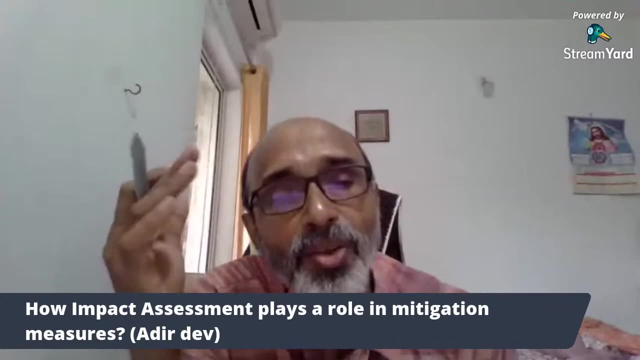 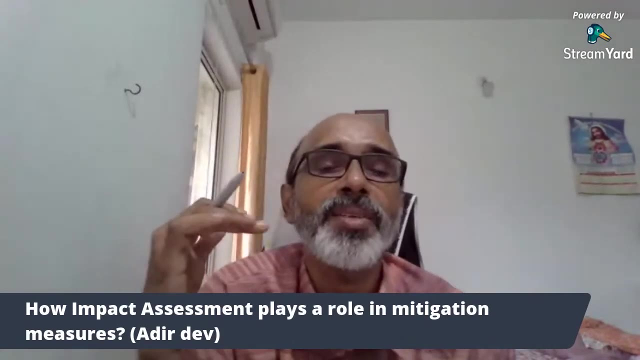 And then we can go for even say: you see that in a country like India almost 65 to 70% water is used for irrigation, So how we can reduce that, Reduce the irrigation and then have a scientific farming and then promote the farmers to use. 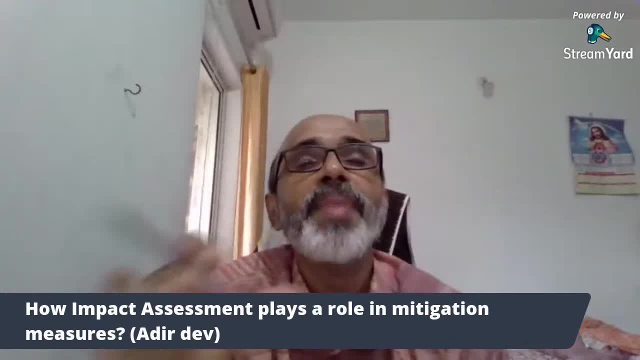 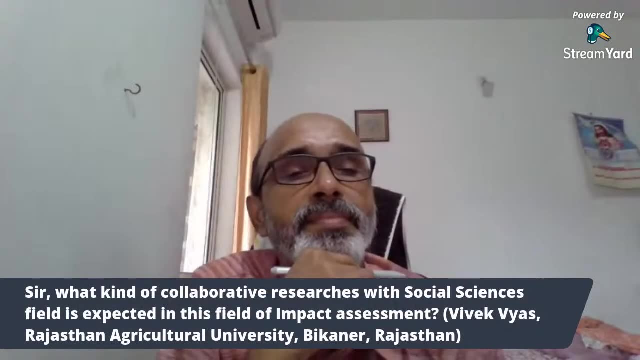 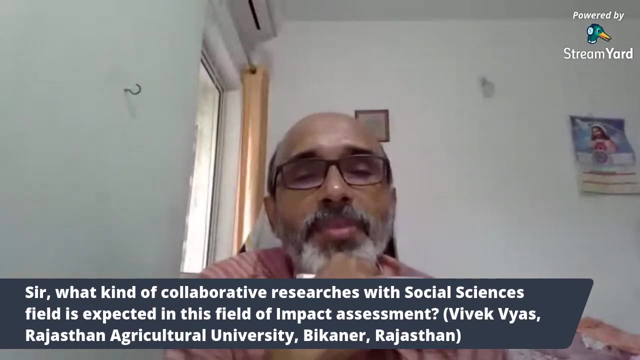 for scientific farming and then reduce the use of water so that the effect can be reduced, So that way we can go for long time planning. Yes, please, Next question. Okay, So the question is what kind of collaborative research with the social science field is? 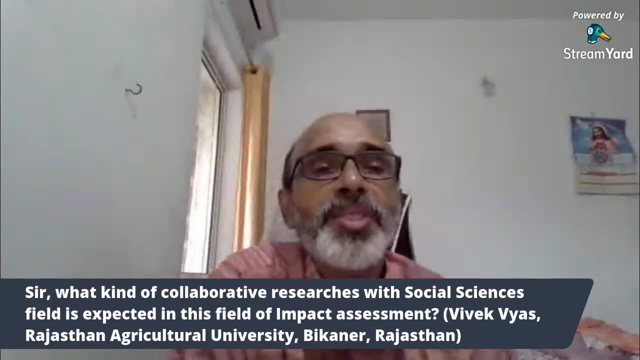 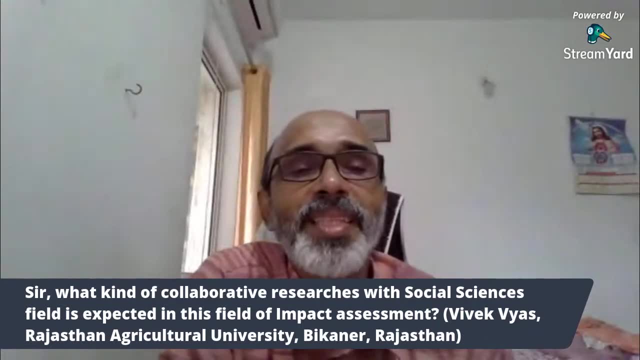 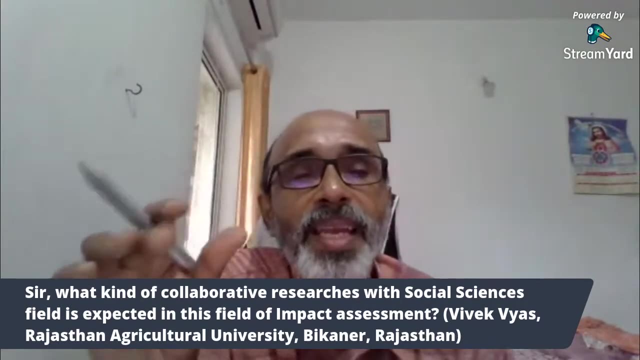 expected in this field of impact assessment. So of course you see that, Yes, Hydrology is very much a social science dependent, since the operation growth, the way the people, I mean what kind of employment they are having, what kind of the way they are doing the farming. 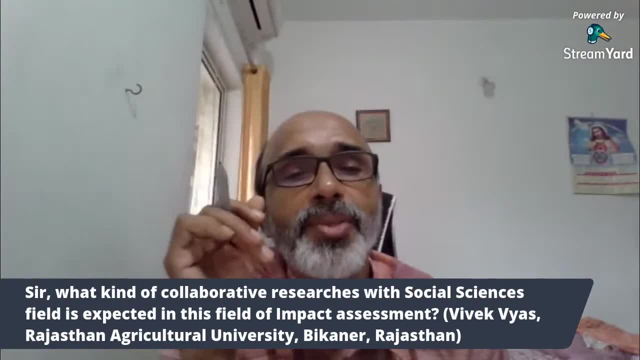 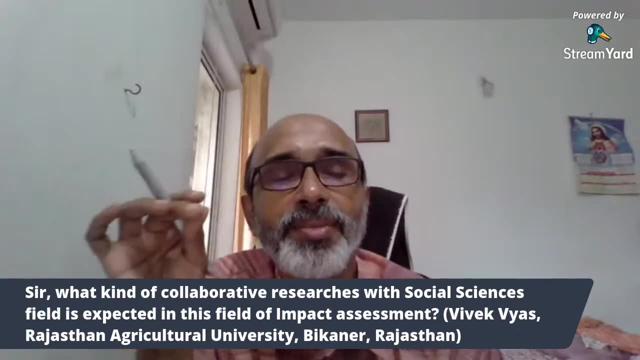 all those things are interdependent. So that way the sociological, social science people can give the various details with respect to the what kind of changes taking place in the river basin or in the state level or whatever the region is. Okay, 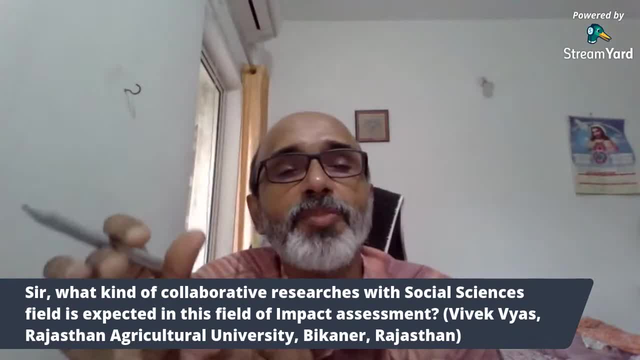 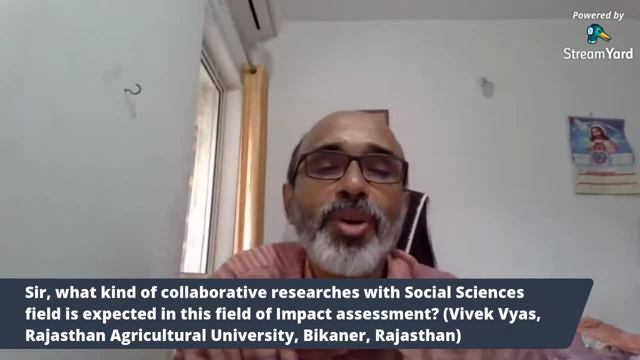 Thank you. So that's the first question which you're considering and that can be correlated with respect to the way we are using the water, especially in allocation policies, especially water resource allocation is concerned. It is, for example, in Maharashtra Godavari River basin. the Jakewater Dam is there. 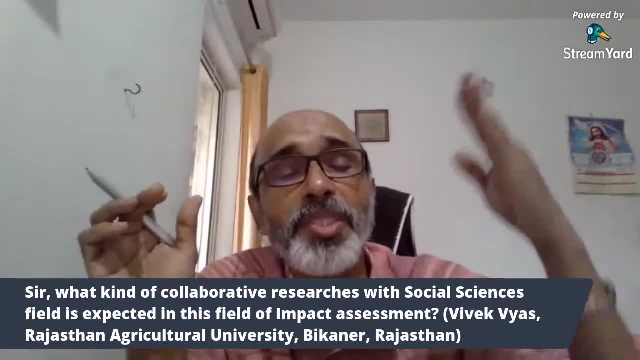 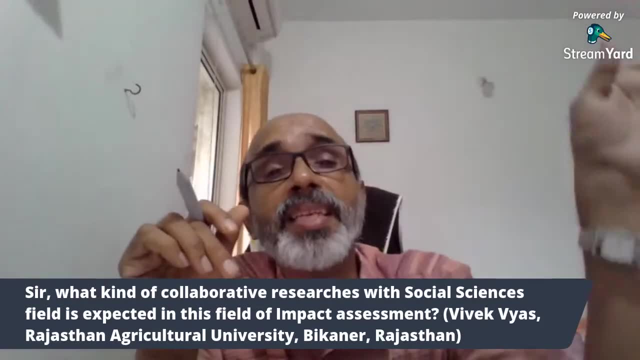 So that is a very large reservoir and then a lot of five-state space between various region in Maharashtra, so that the allocation is concerned. So there the social scientists can say that, okay, this is the way it is happening, This is the way it is evolving. 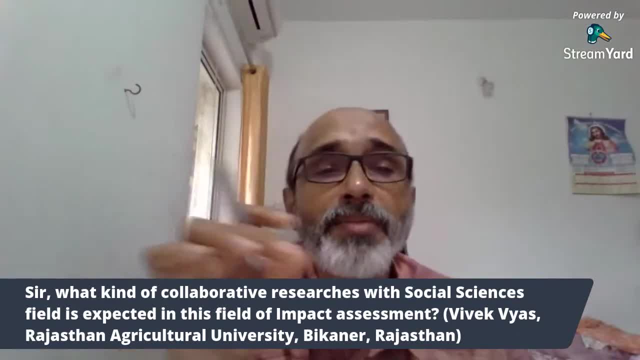 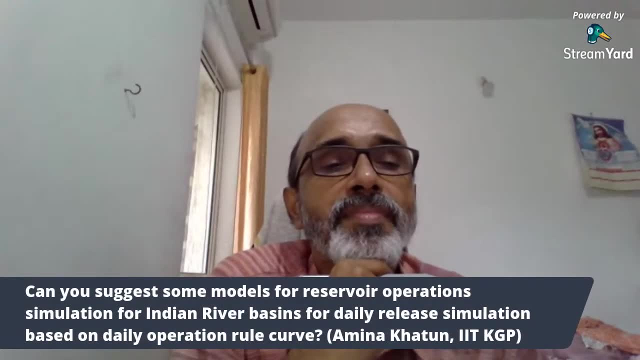 And then we can come to the solution. Okay, we can come with appropriate planning with respect to the hydrologic impacts is concerned. so next question: please can you suggest some models for reservoir operation simulation for in their over basin, for daily release simulation based on daily operation rule curve? so this is 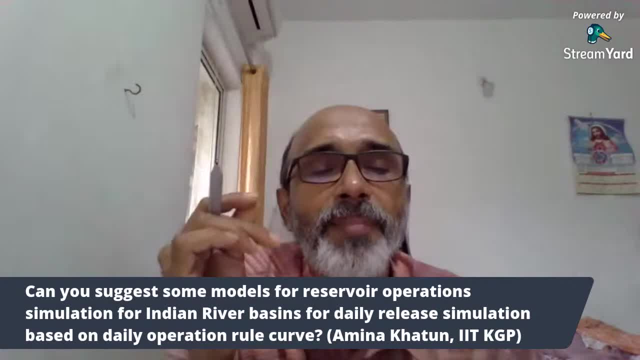 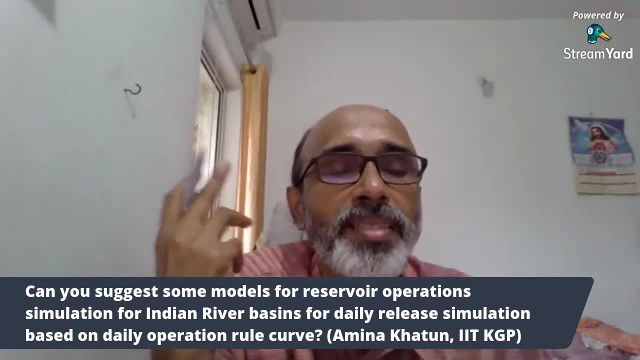 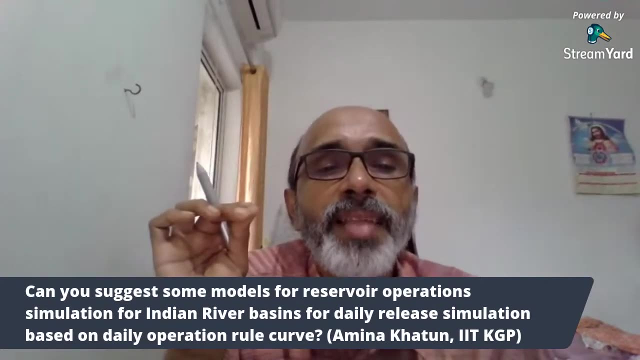 concerned. say, for example, say when you consider for a river basin is concerned, so the total like to take, what are your basin? or if, depending upon the, the area, so that we need to assess what is happening in within that river basin. so that way we need to get much better assessment for the. 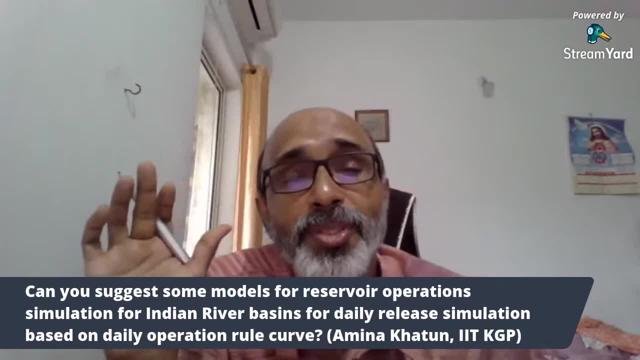 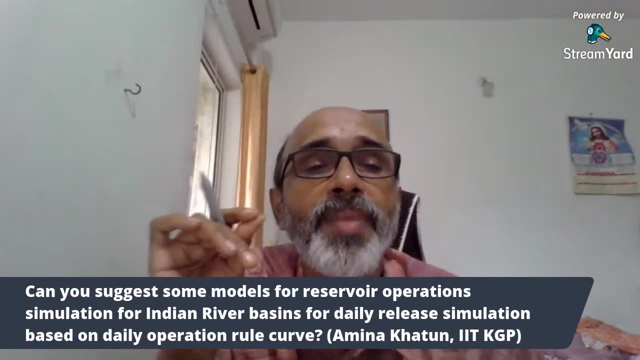 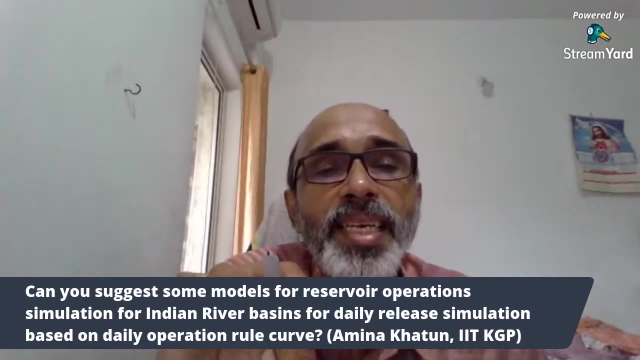 reservoir operations. so of course nowadays most of the engineers they are using rule curves, all those things, but this rule curve itself, that policy can be changed by using this kind of hydraulic impact assessment. so there are models like a sheet run or model like can be effectively utilized and integrated in such a way that daily pattern can be captured. so, for example, 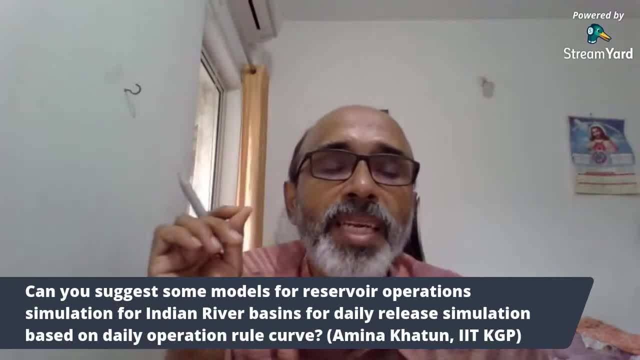 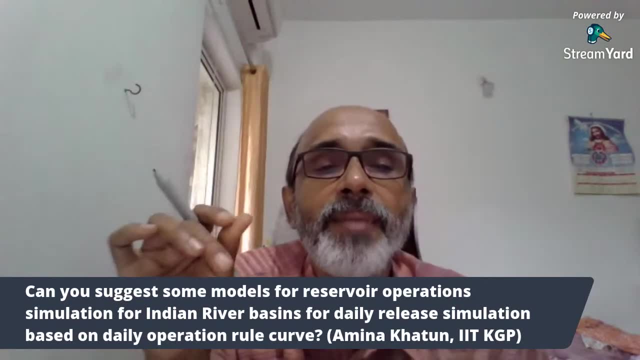 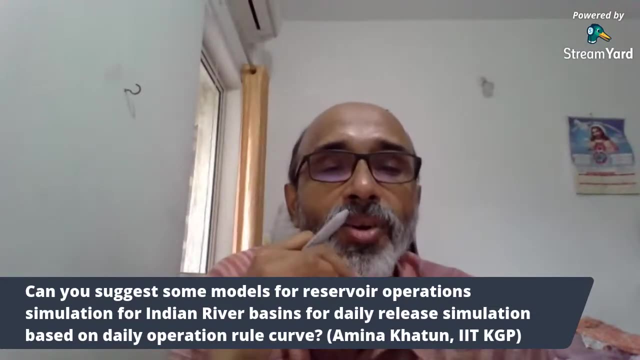 in a model like BIC, that kind of details may not be able to get it, but in sheet run or maxi, that kind of models we can get to the what is, what is the way changes taking place and that can be daily basis we can correlate with. with respect to daily release or the reservoir simulation is concerned, 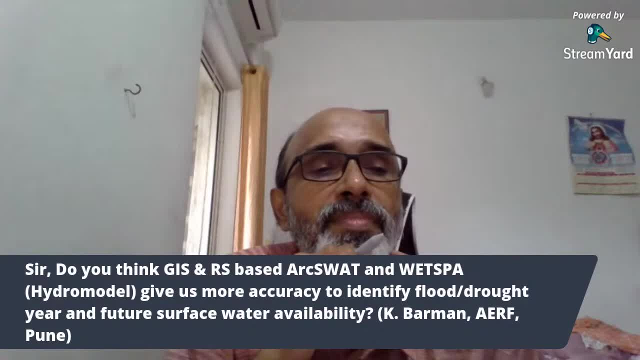 next question, please, okay. so the question is: do you think GISR R, SWAT and wet swabs pair model, hydraulic model gives us more accuracy to identify flood throw out here and which surface water availability? so, as I mentioned, SWAT is concerned that the concept is or the same, so even now, or the other. 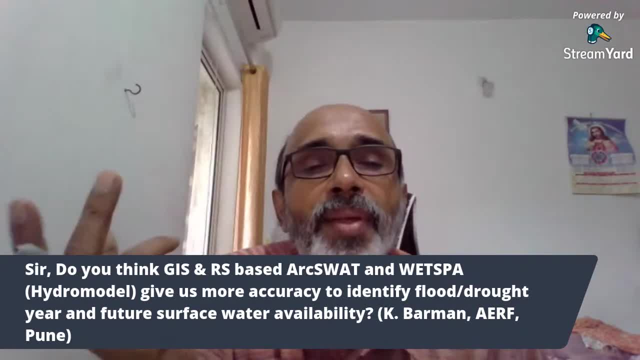 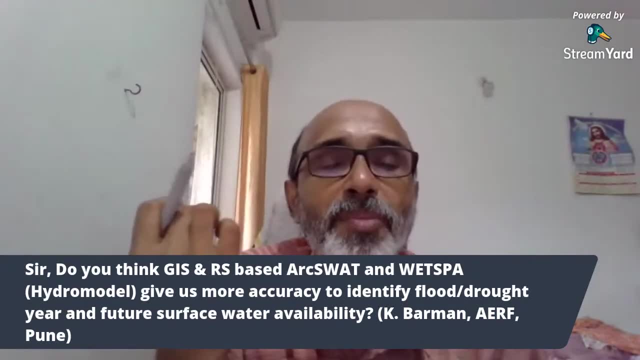 models. the model is. most of the models are based upon scientific basis and then the the results will change for sure. so what will be the cost of effective красing for yawayesh isktốcpsadeer? almost important what kind of input you are giving the data. the data set is much more important. so if 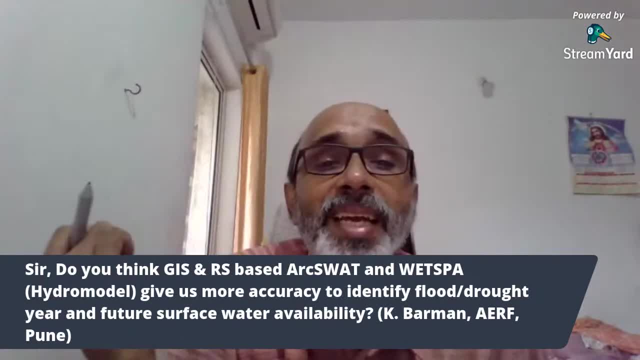 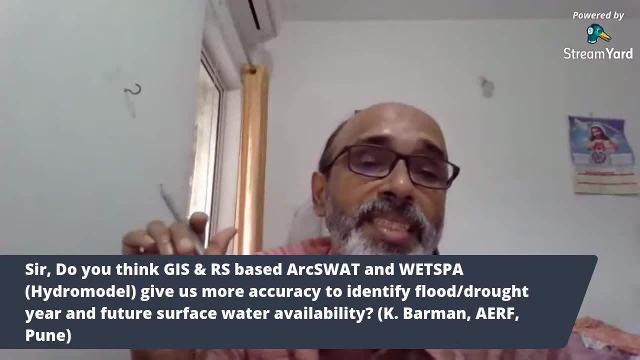 you put accurate- i mean the, the best data- then you'll get a best output. but if the data set is wrong, if the data set is not proper, that is the major challenge as far as the vehicles are concerned. so, model, most of the models will be giving support, reliable results, but otherwise, 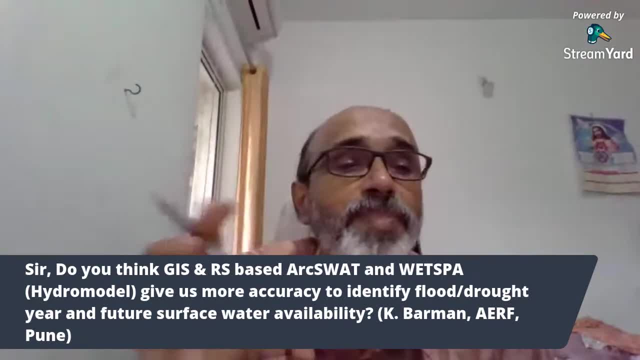 the issue is that data set so outside or even uh, um, all these models, they had a model that it will be very similar, similar kind of, though there can be some variation, but results will be almost same. but the data is the main issue. so, if you have the 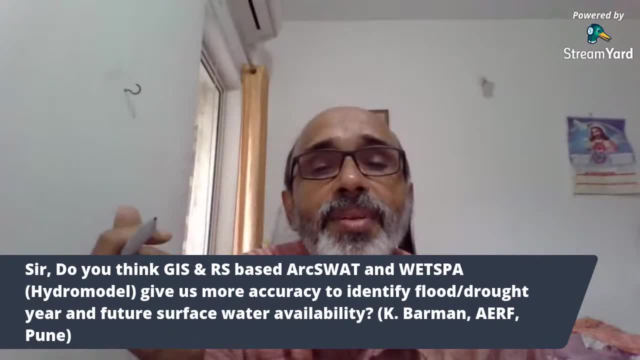 very good data, then, whatever the results you are getting for blood or production, we can go in a better way. but please remember that the flood is concerned, flooding is concerned. so this model, like a swat or these things that may not flood, these concerns generally, it is even based. even based means it is for a few hours time or few days. 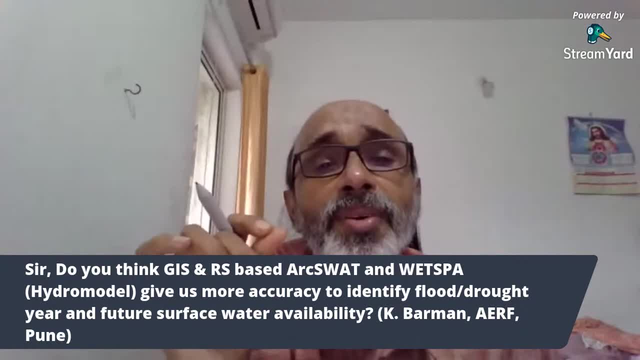 time it is happening and then we need to capture all those. so in a swat model or that kind of model, we may not be able to do, but in my she or she trying that kind of model, the advantage is that it is grid based and then it is a process based uh model. so that way, uh she. 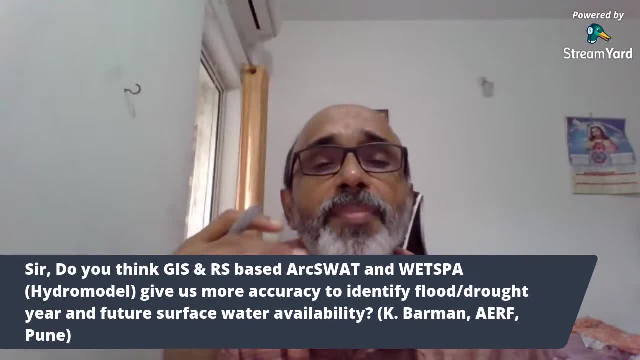 plan or my she she model or in a physically based model, can give a better prediction, better way of giving the output as far as the, the, the, the, the funding is concerned, but the drought is concerned, it is, there is not that much. uh, it's not different, but the flood is. 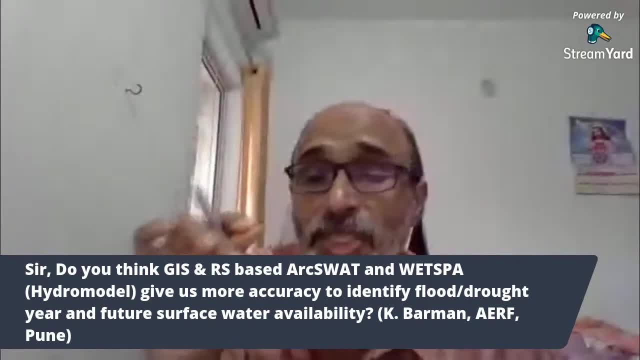 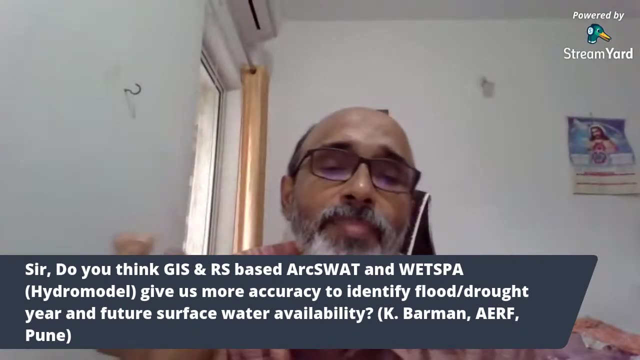 concerned, it is very much areas, basic, basic, specific and that particular area basis, short, small grids, small areas to be considered. and then time is very important. so it is always better to go for a hourly basis prediction, but most of time my model, like swat, is only daily basis. 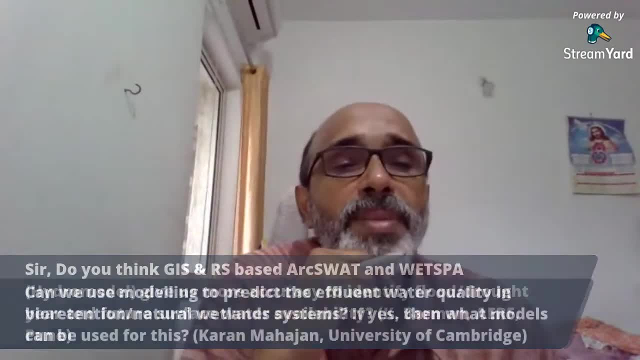 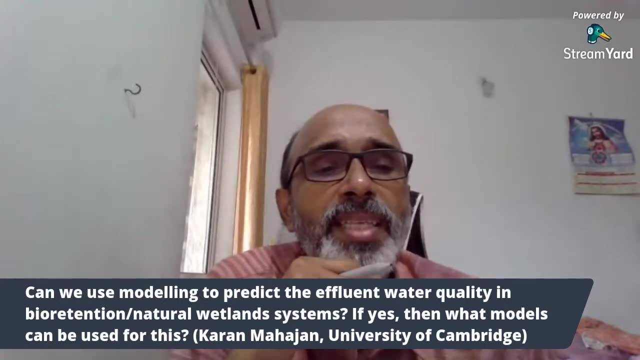 prediction and that may not be sufficient. okay, next question: please, can we use more modeling to predict the affluent water quality in a bioretention natural water wetland systems, eps? then what models can be used for this? so here i'm say, to see that effluent and water quality. so 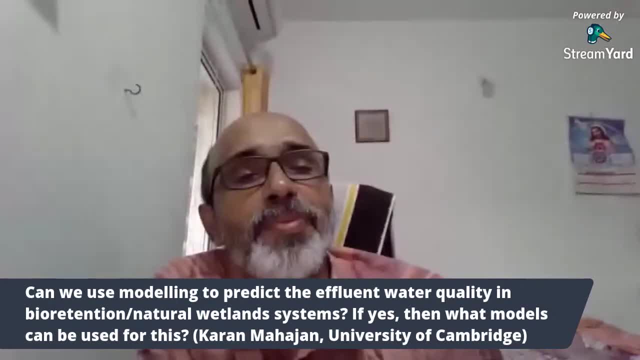 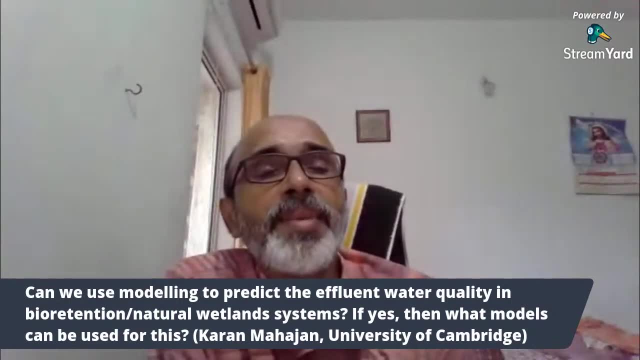 there, as i mentioned, this model like a sheet rank where the transport phenomena also can be easily simulated. actually one of my phs who recently graduated, so she has used a sheet and model. so there the advantage is that for a small scale, especially grade level by gld and nogu, remain true to service to well the most: the néstor. 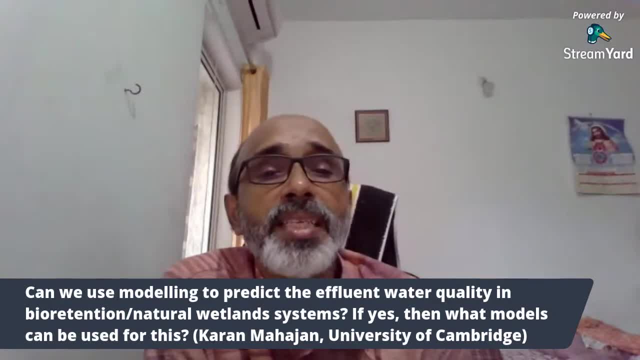 field is the one is the one that we can use for the largerED at the time water quality is concerned. we take a small river basin or small areas where you, even with a private model, we can club together. so sheathland is one of the suggestion model for these kinds of studies as far as water quality is concerned. 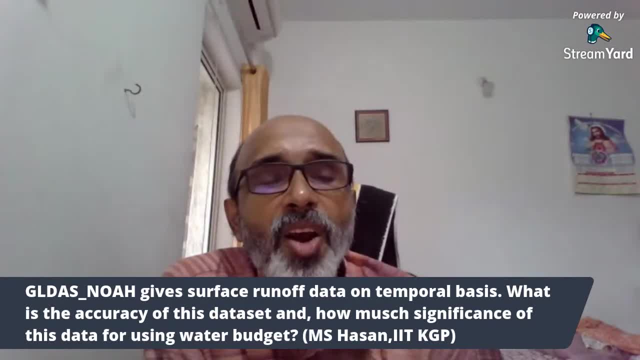 next question: please, uh the no muss surface run of data on temporal basis: what using water budget? so actually this, uh, this data set i have not used. actually my colleagues, like, of course, rajadamshankar and professor hindu, they are all working on this, uh, this, uh, real, like. 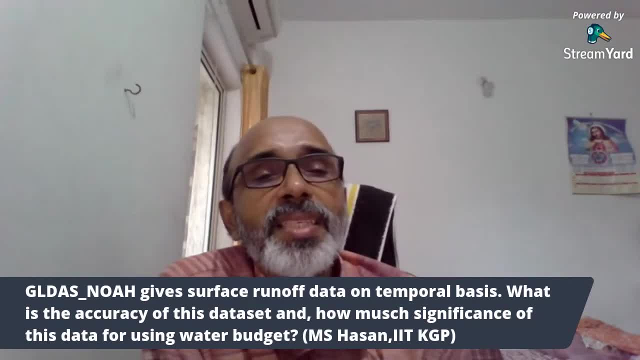 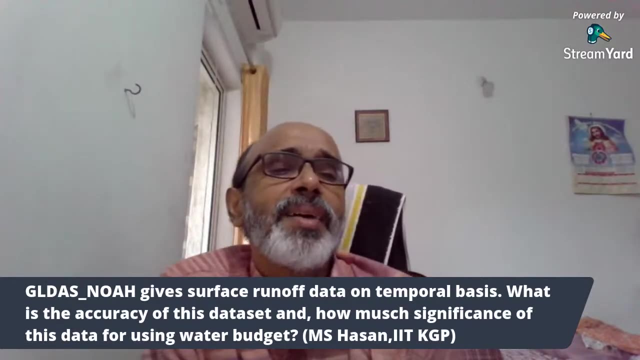 remote sensing data or this large scale data is concerned, since i am not a person, since i work more on ground basis or the the river basis, more scale, this basin level, so that way- but many of these shows that, uh, in a large scale, these kinds of data sets are giving a support reasonable. 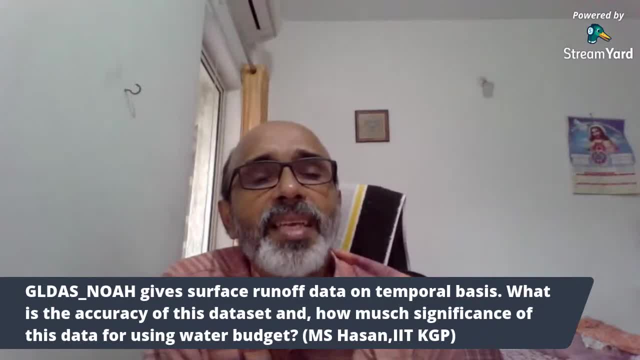 results. when we take on an average sense like the, the, the, when we compare with what is, with respect, imd or other kinds of data sets, it gives a reasonable results. that is what i understand from my colleagues and the papers published. so most of the database is available. we can. 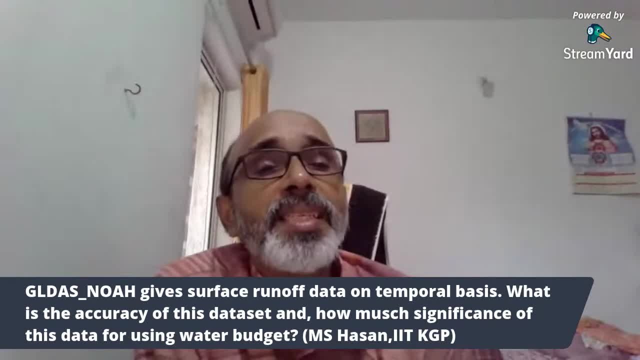 reliably use. as far as the for especially these are these kinds of data set- is available. when you go for large scales, for example, if you want to do for entire country, or if you want to do for a very large river base like gadget basin, then these kinds of data 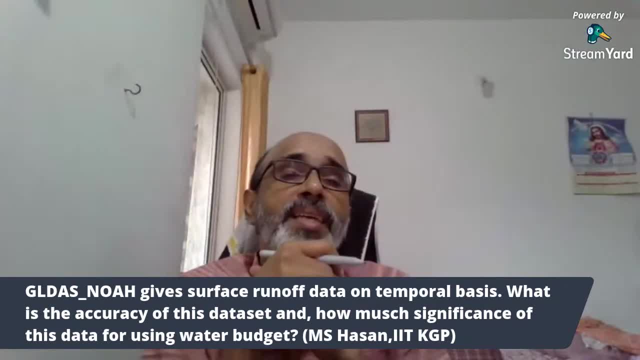 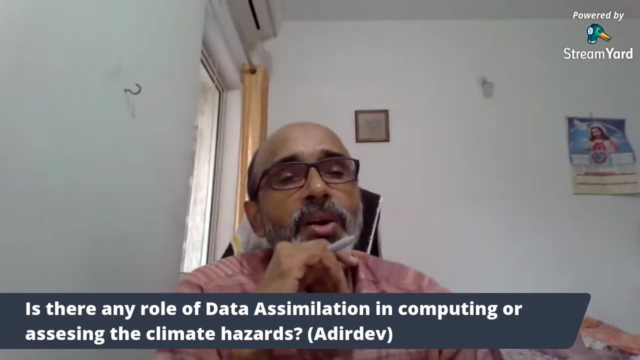 situations, but they're going for small river basins, then these kinds of data set, the utility will be less since you may get only one or two points. uh, particular gritty, good discount set. so that kind of restriction will be there, okay. next question, please. okay, is there a lot of data? 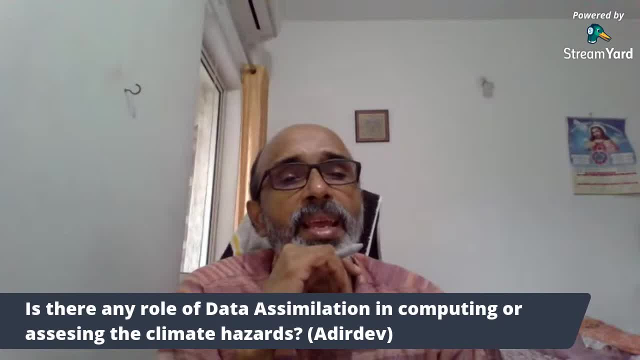 simulation, computing or assessing the uh climate hazards. of course, that assimilation is. a lot of work is going on, actually my colleague, professor raja ramsangar. he is working in this area for data assimilation is a very important tool which we can utilize for the hydraulic impact assessments. 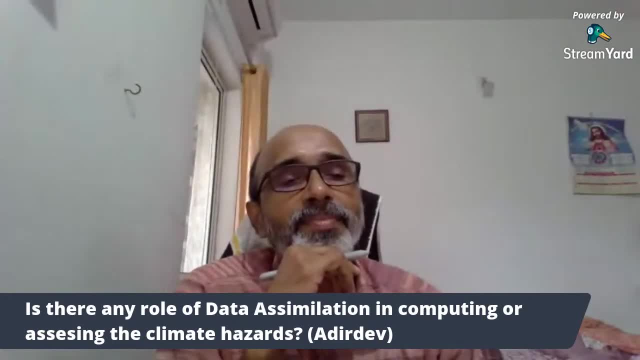 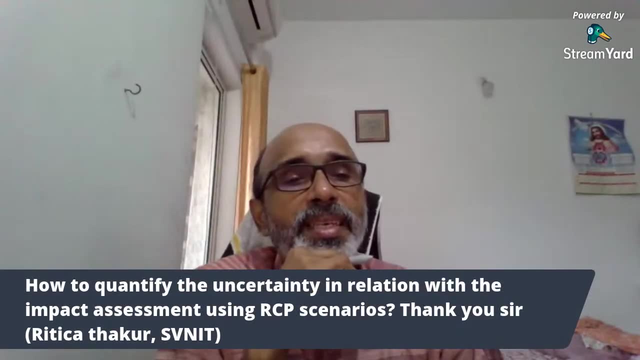 that this can be very much used. next question: how to quantify the uncertainty in relation with the impact assessment using rcp scenario. so how to quantify the uncertainty in relation and with the impact assessment using rcp scenario. so the uncertainties, as i mentioned, uncertainties are with respect to gcm, uncertainty can be there. 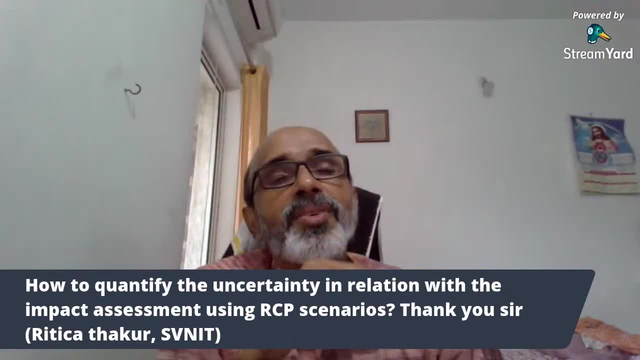 with respect to the model uncertainty can be there. so a variety of uncertainties we need to look into. so that way, when we look into uh assessment, so we see that uh say, when you take a rcp- rcp 4.5, 8.5, whichever you are choosing- so we need to see that, especially a gcm scale level, a lot of uncertainties. 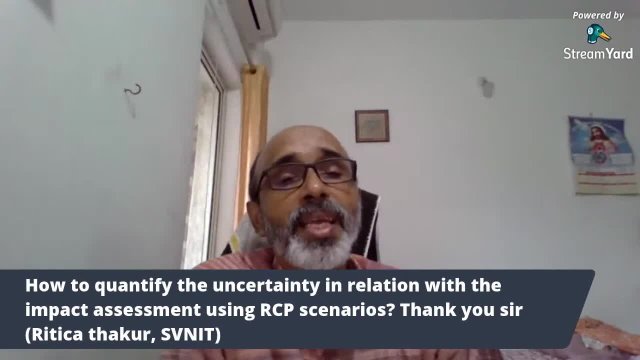 upset even, uh, some of these students say they consider 15 to 20 gcms and then they study the uncertainties and then identify the best and then compare. so that kind of a number of gcms, always, you can do a variety of models. like you know, another important model is called the hoa model is also. 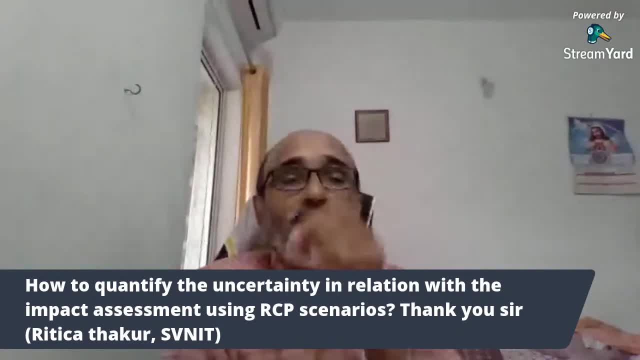 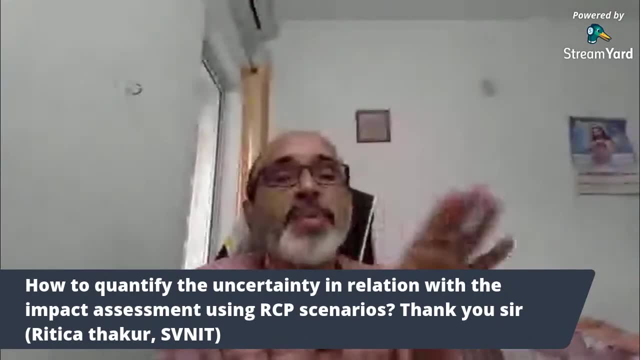 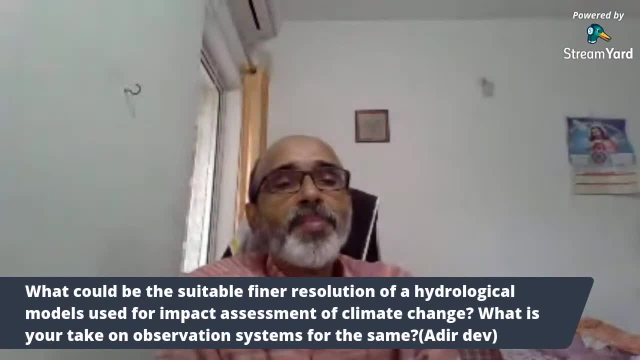 so what could be the suitable final resolution of a hydrological model is used for impact assessment of climate change. what is the? what is your take on observation system for same? so here generally. so you see that that depends upon the river basin. so, for example, a small river basin. 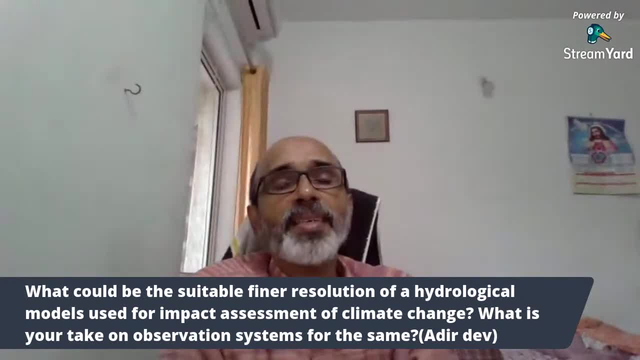 like this: whatever we are talking, it is hardly 3500 square kilometer area, so there minimum is should be 0.25 degree or 25 by 25 square kilometer. i mean that should be the minimum grid scale, but it is always preferable to go to 0.1 degree at least 10. 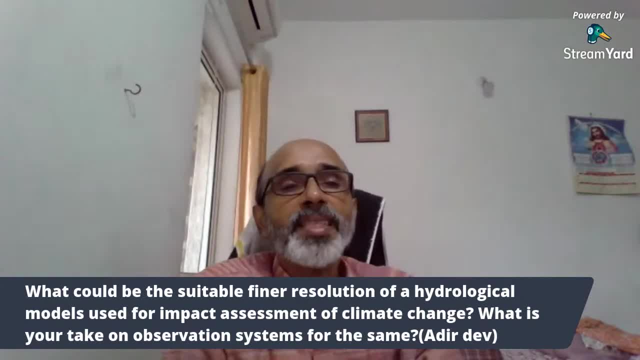 kilometers by 10 kilometers. that is most preferred as far as the impact assessment, hydraulic impact assessment- is concerned. so it is finer, which is better. but the issue is that the data data generally, for example the hydrological data, the rainfall data, is available, with a good distribution of rain gauges, all those things available, especially in the historical data. 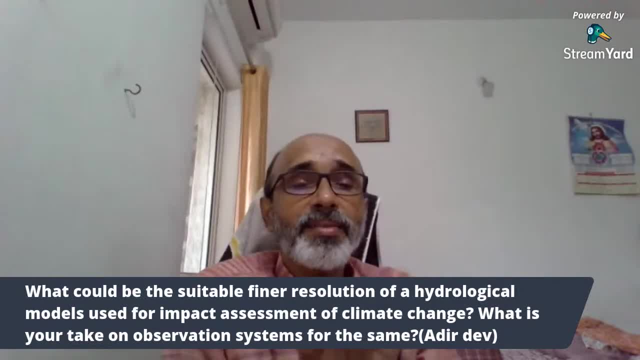 from that we can do a lot of assessment and that so correction can be done. so 0.1 degree by 0.1 degree is more preferred, but at least minimum requirement will be 0.25 degree. i mean 25 kilometer by 25 kilometer. that is a minimum requirement in most. 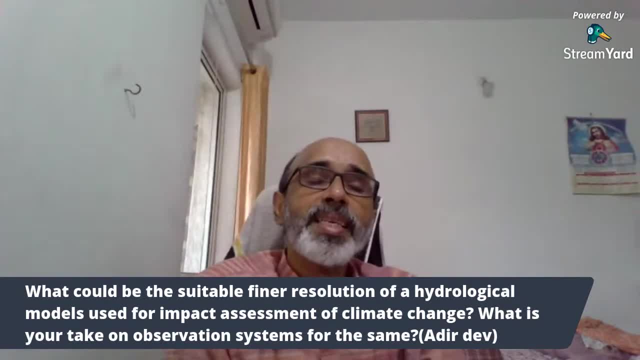 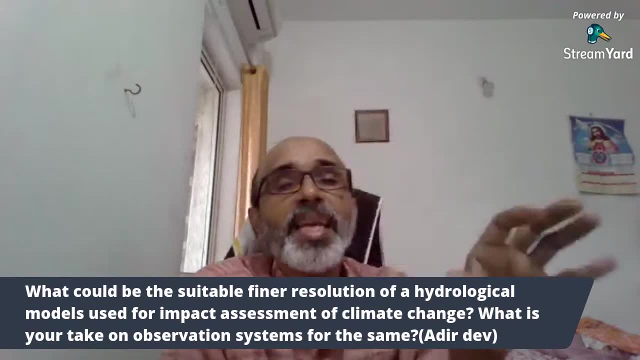 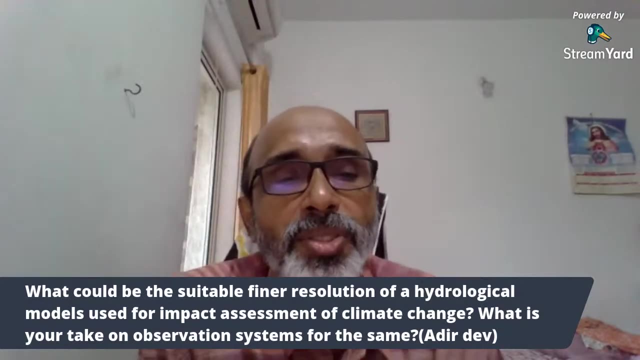 of the river basin scale, so so that we get to say, for example, if i am 5000 or 6000 square kilometer area, there are at least 10, 15 weeks. we can see and then get a reasonable understanding what is happening with respect to the, the climate change. on the hydrology, next question, please. 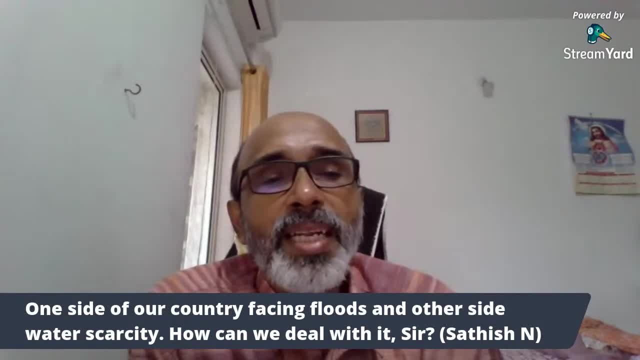 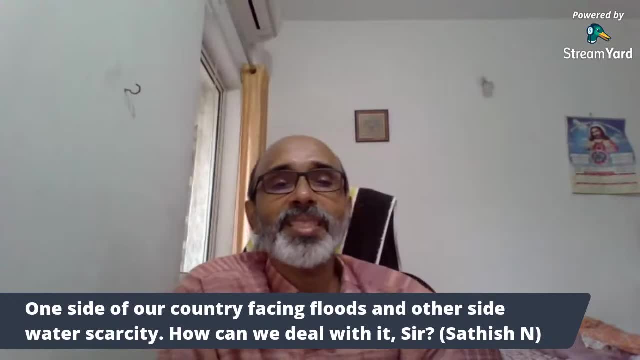 okay, one side of our country facing floods and other side water scarcity. how can we deal with it? so this is a very general questions, psychological questions. so here you see that one, one aspect is that, of course, this climate change and then its impact. so you see that. 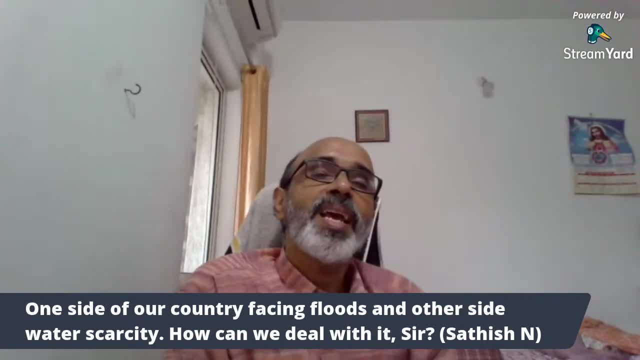 if you study the, the land use, land cover, change. what is happening now, unfortunately, say. now you are running newspaper recent times even the environment policy the government is changing. so if you read the newspaper recently, a few years ago, the environment policy the government is changing. so one aspect is that if you tighten the environmental policies and then so that 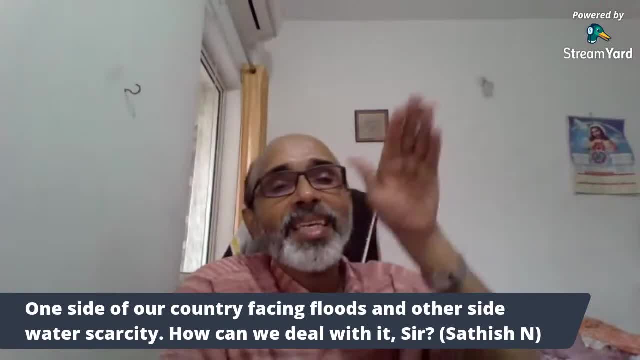 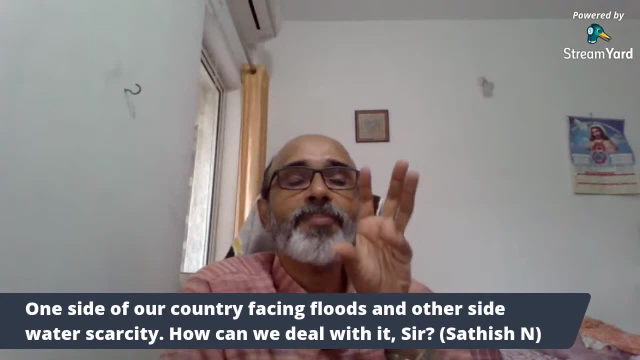 not much changes should take place now. what is happened is happened now further we have. we cannot go for a further relaxation in this policy, so we need to tighten the policies and then we need to go for further protection of the environment and forest should not decrease. all those these things should happen so that whatever the mass can be reduced and then 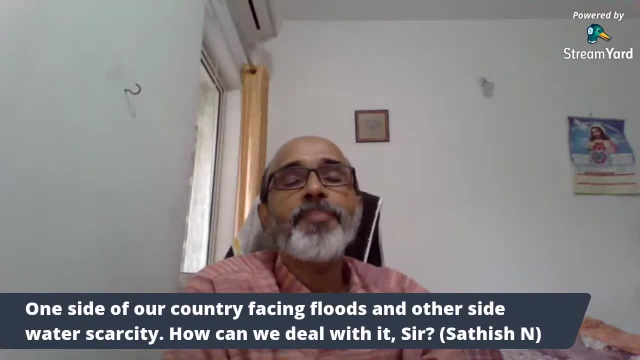 of course, and the, the water scale cities concerned there. you see that many times, as i mentioned, in india is concerned even so much of what is used for irrigation purpose. so as a researchers here, all of us need to put a lot of efforts to come with the. 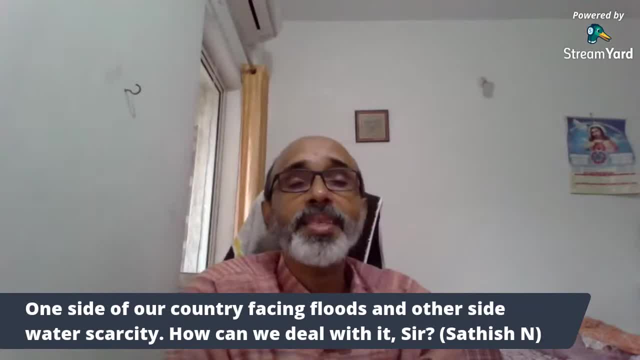 scientific farming, then efficient water utilization or irrigation and plant growth- all those we need to look for so that way we need to see that the the blood situation can happen. but is so the various measures government can? now we should have most environmentally strict rules so that further relaxation should not be allowed, and that is one aspect. and then we need to go for. 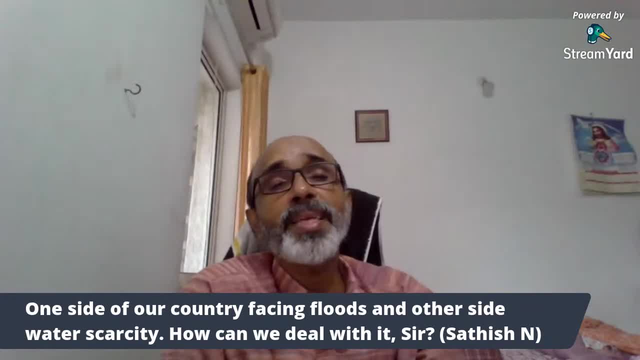 planning and then land use, land cover change. so many many places like in places like kerala, asam, etc. you can see many, lot of construction activities, lot of land use. land change took place in the last two few decades and a lot of construction took place in the flood plains of the rivers so that